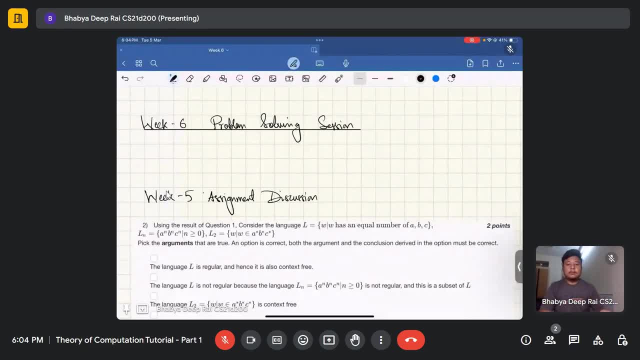 Good evening everyone. welcome to problem solving session, week 6 of theory of computation. So this week's topic is Turing Machines and Decidability. Turing Machines and Decidability. So before I deal with some questions on decidability and do a short recap on Turing Machines, I 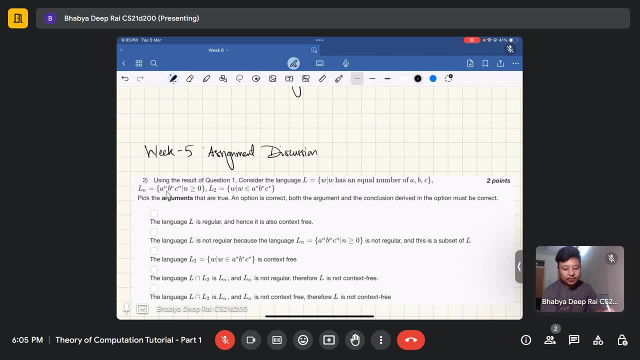 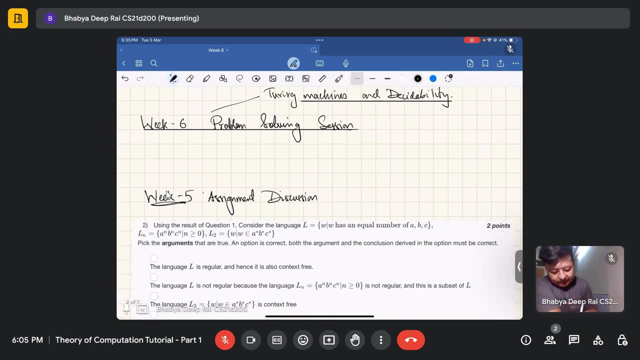 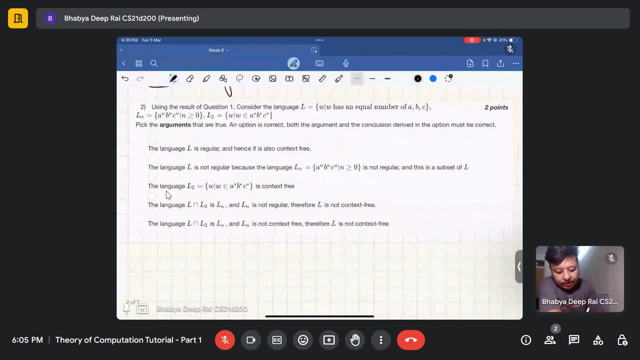 will discuss just two questions, Questions based on the previous assignment, that is, week 5.. So let us begin. so this is assignment discussion. So the question says: consider the language L. W says that W has an equal number of a. 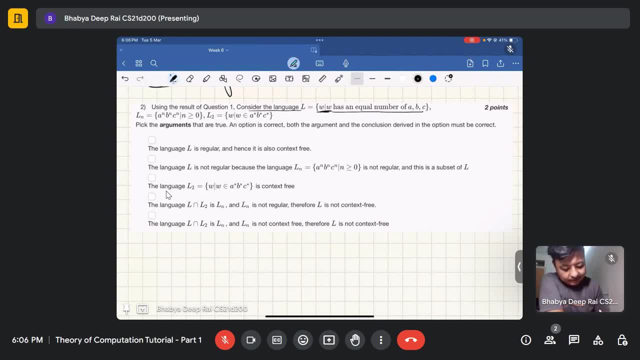 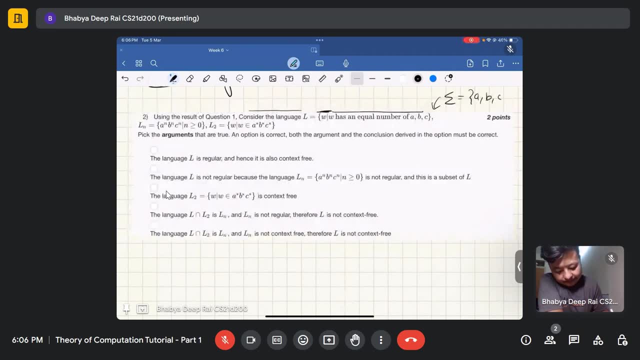 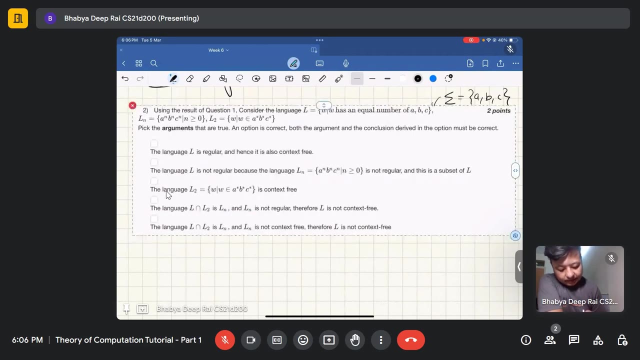 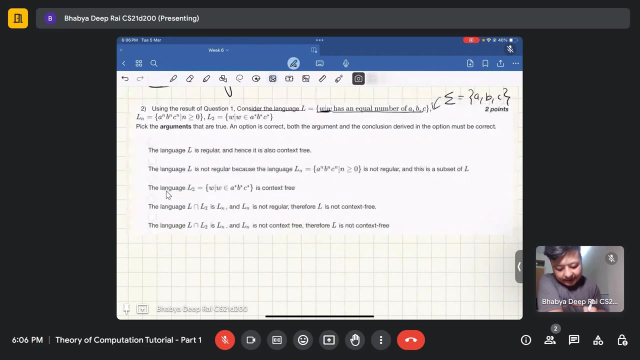 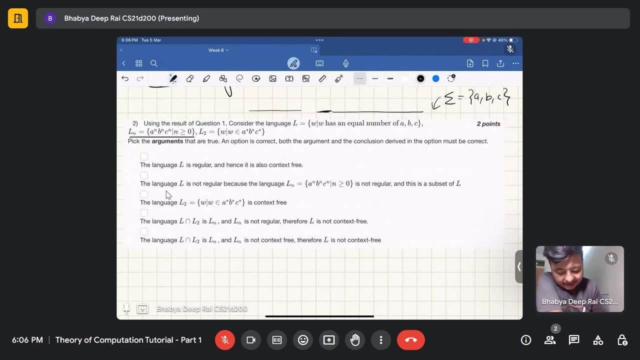 b, c, d. So here we can see that sigma has a, b, c, the alphabet, Next L. this is the first language which is called L. Next L is a to the n, b to the n, c to the n and L2 is W, such that W is in a star, b star. 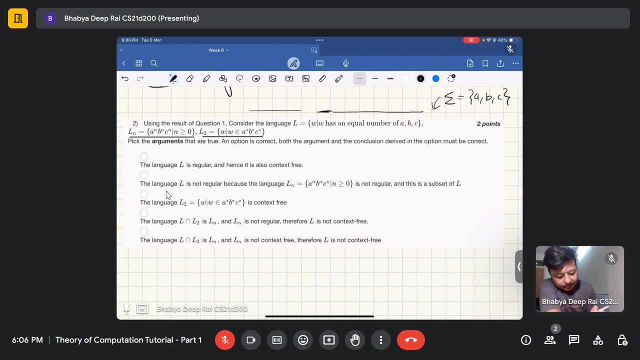 c star. So immediately, first let us see what the question says. pick the arguments that are true and option is correct. both the arguments and the conclusion derived in the option must be correct. Yeah, So next let us look at the options. 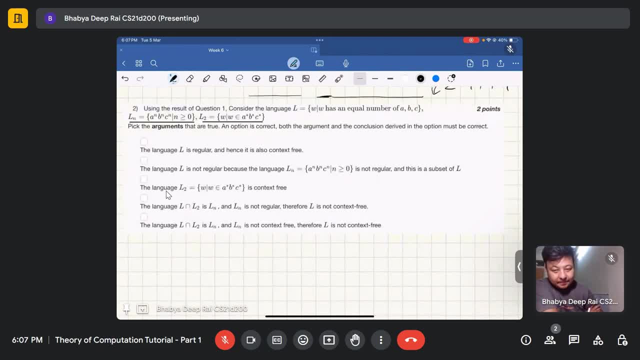 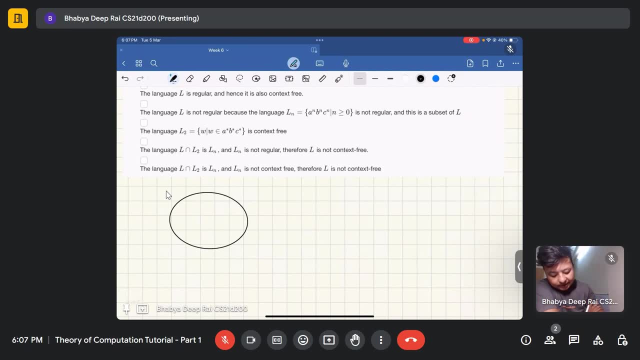 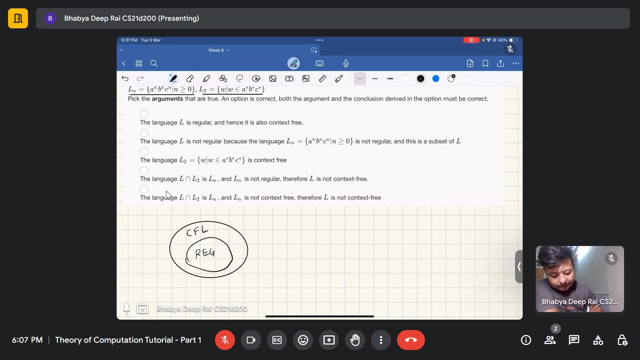 First one is: the language L is regular, hence it is also context free. Well, this of course does not make sense, because the regular language sit inside context free language, So all regular languages are context free, and hence it does not make sense to say: oh sorry. 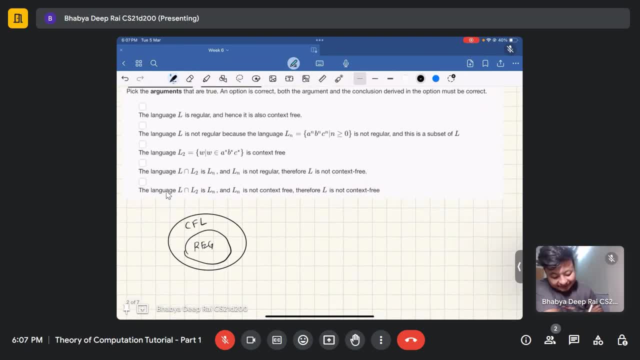 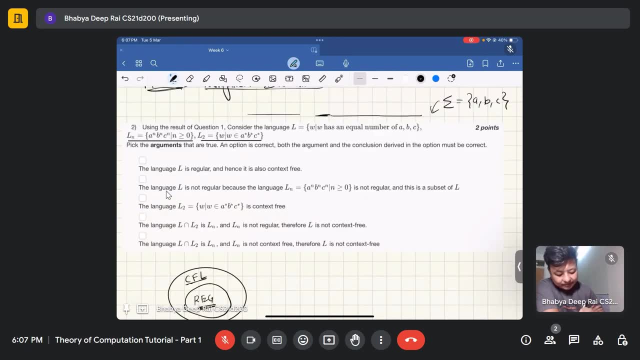 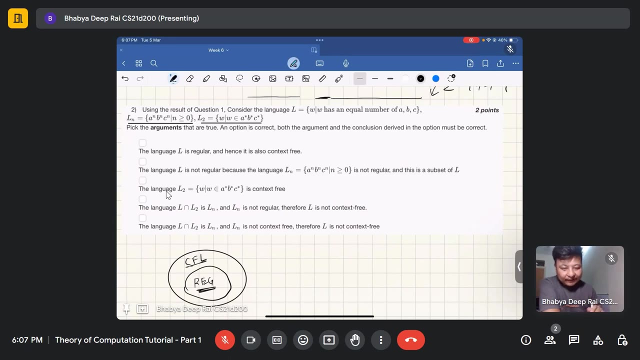 it does make sense. The fact that a language is regular also means that it is context free. It is saying the language capital L is regular. Okay, What does capital? what is capital L, W, such that W has an equal number of a, a's, b's and c's? 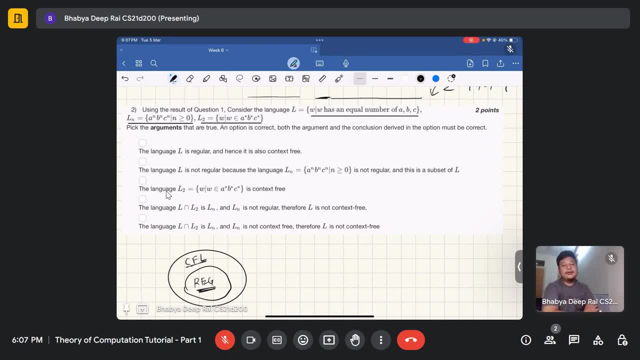 Now, on face value itself, this language does not seem very regular. We have not seen any DFA that would recognize such kind of language. Okay, And this, this does not appear to be regular, but of course I mean there are a lot of. 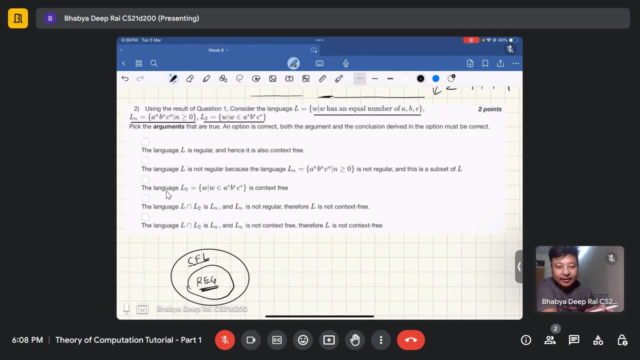 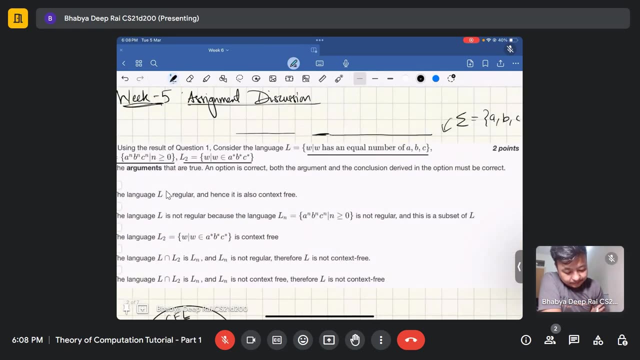 tricky languages whose definition makes us feel that uh, uh, makes us feel that way that it is not regular. uh, it is regular, but in fact it is not. So let's see: Uh, W says that W has an equal number of a, b's and c's. 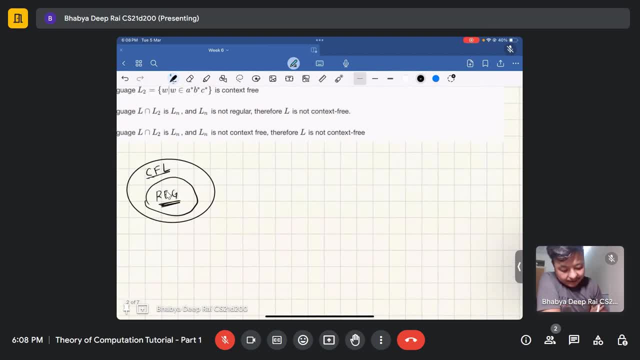 Okay, Okay. So, um, W says that W has an equal number of a, b, c, right? So, uh, one way to disprove this B using pumping lemma. Okay, Choose something like a to the b, b to the b to the b, c to the b. 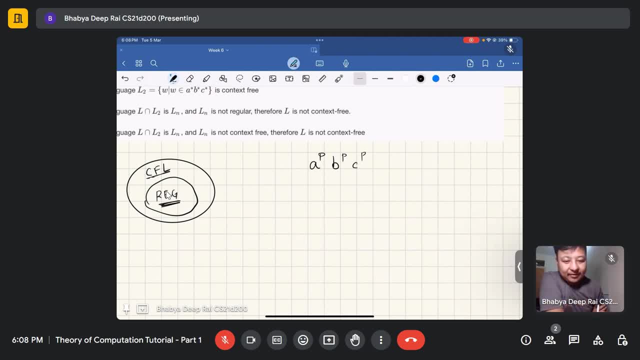 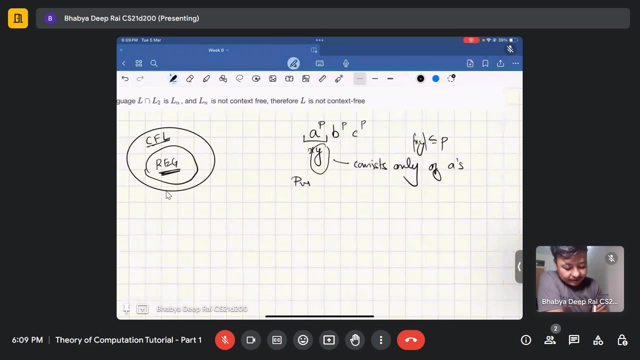 Now this guy has an equal number of a's, equal number of b's and equal number of c's And by the pumping lemma, uh, x, y is at most of size b, Right, Right of at most p and therefore y consists only of is right now you should pump y. that's what the 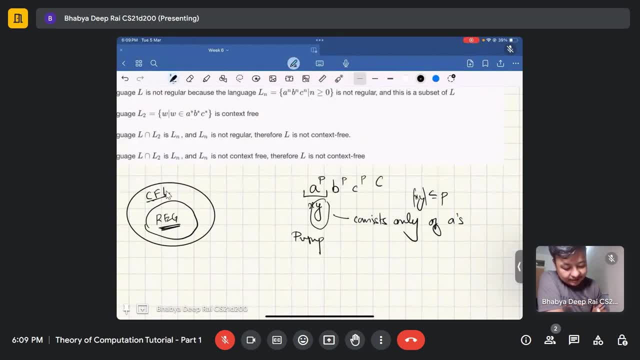 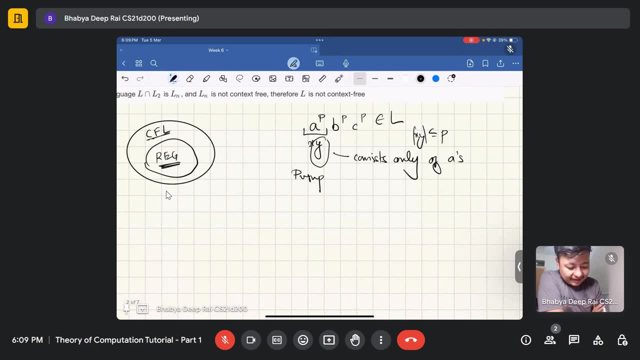 pumping level says: right and this- this guy is in the language- l right and uh, let's assume that l is regular. that's how we do it in pumping level. if you assume that l is regular and p is the pumping length given by the pumping lemma, then pumping lemma says that no matter. 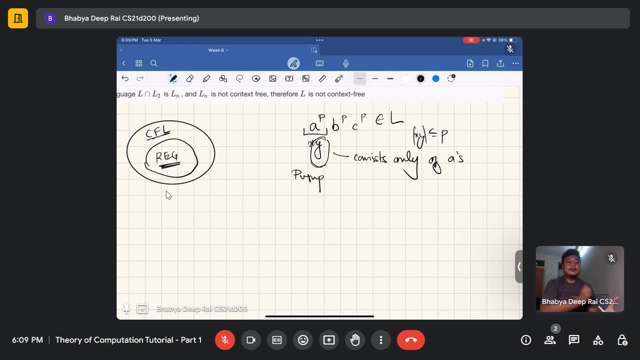 how many times i pump y, the string will still be in the language right. so if we pump y's, okay, we get a to the p and uh- let's say uh- consists only of a's right. y, consider only of this. let's say y equals um. 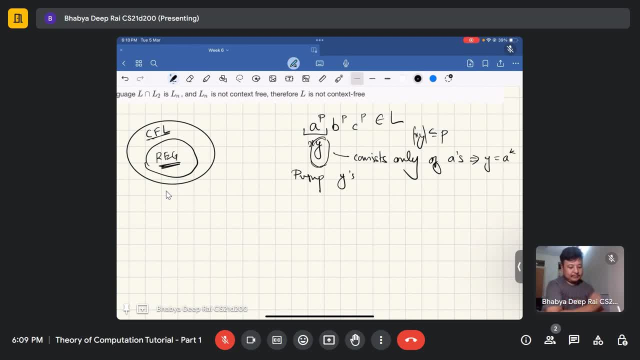 a to the k, then if we pump y's, x, y square um, z. if you do that and this part is z, then what do you get? x is some x, y is totally a to the p, and if you add one more y, then you have k, more a's. so there you get. 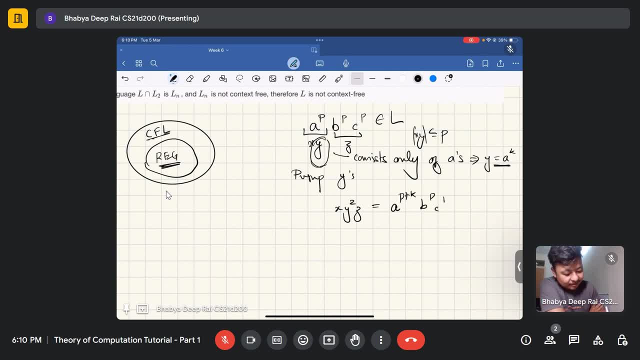 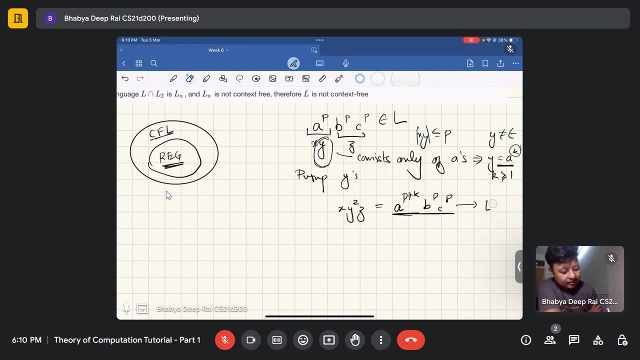 a, p plus k, b to the p, c to the p, and since y cannot be, cannot be empty, this k is greater than equal to one right and therefore, according to pumping lemma, this should be inside l, this should be inside language, but uh, clearly this is not inside. clearly this is not in. 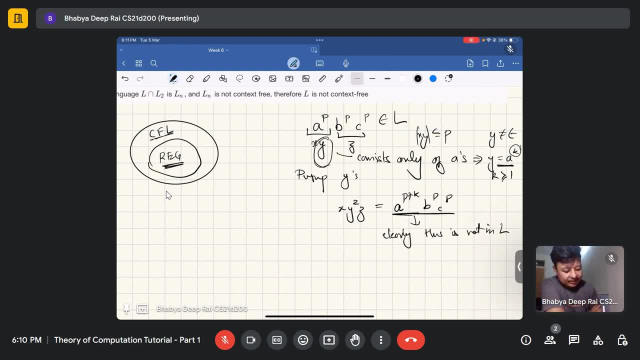 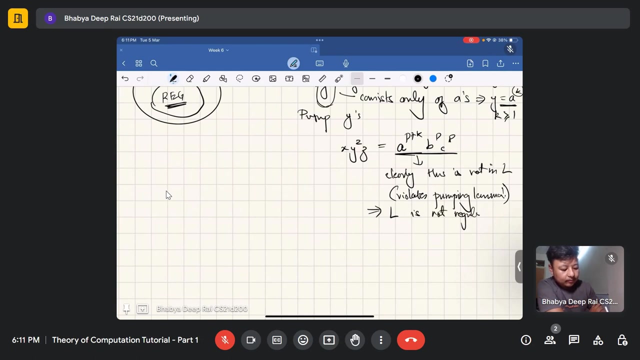 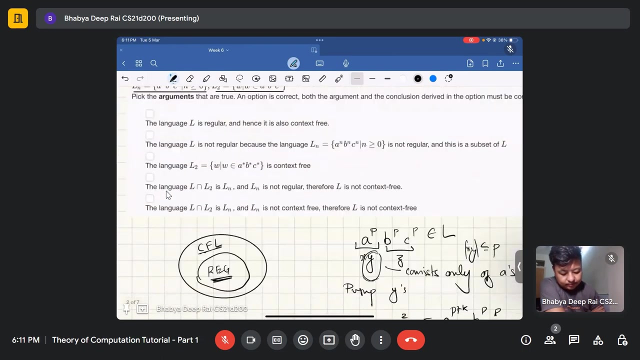 l, but which this violates. pumping level: pumping lemma would not have been violated if um pumping lemma would not be violated if l use l was actually regular. so this shows us that l is not regular after all, okay, so, uh, language- l is regular- is out of question. so option a: 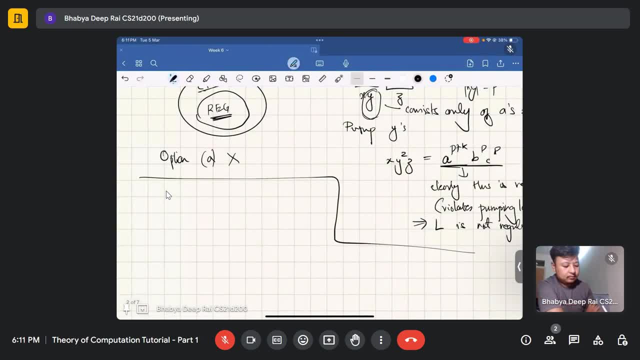 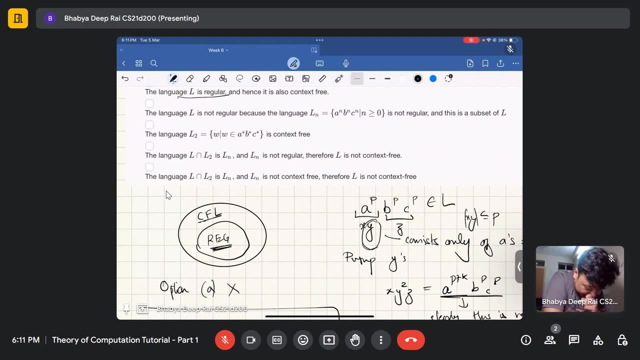 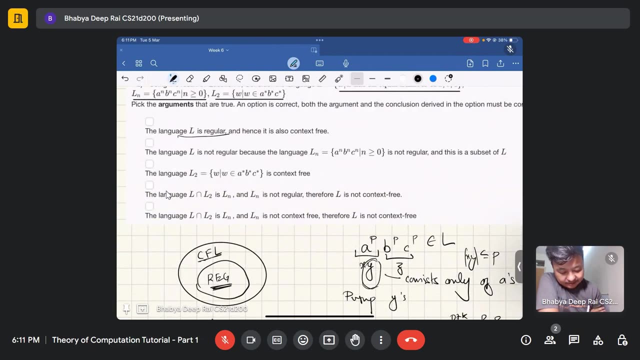 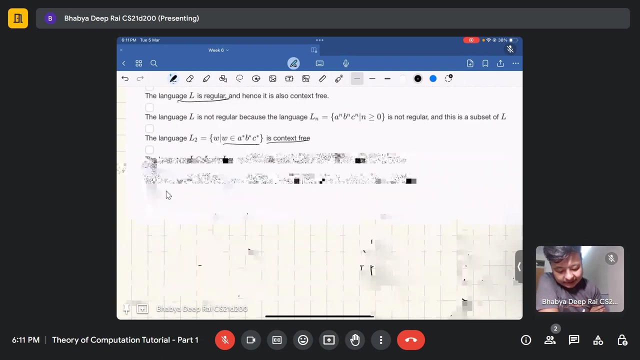 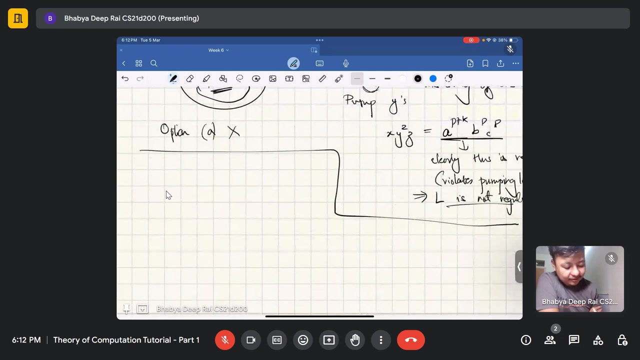 is from. let's look at the next one. the language l2 equals all those strings uh, where a star b, star, c, star, uh, w is in a star b, star, c, star is context field just to back it. thanks, and call it play, because learn what it does. 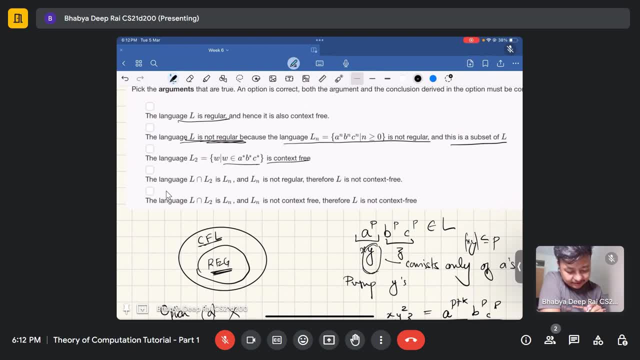 so okay. the next one is the language. l is not regular. okay, l is not regular. okay, that makes sense, because, uh, here it means l is not right, so l is not regular. but what is the ln a to the n, b to the n, c to the n is not regular. 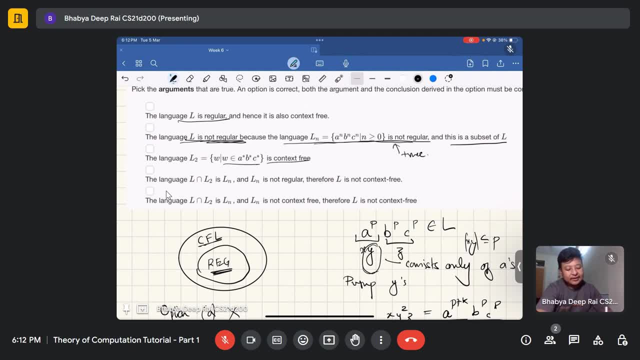 This is true. This statement is true. We've seen that, In fact, this is not even dCFL deterministic quantity language Right And this is true. This language- a to the n, b to the n, c to the n- is very difficult to compute. 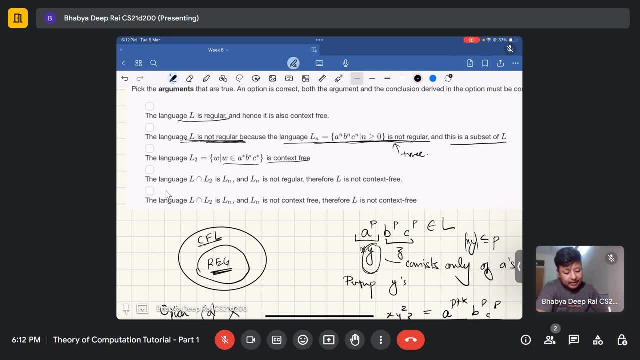 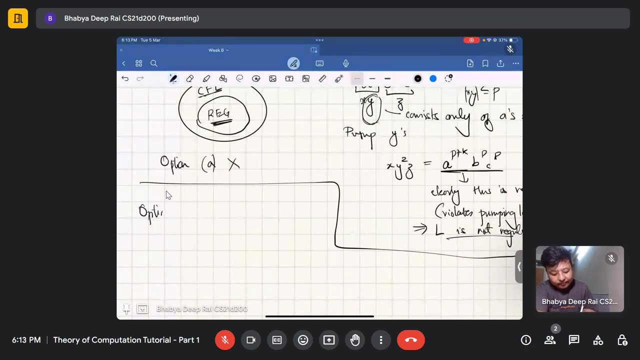 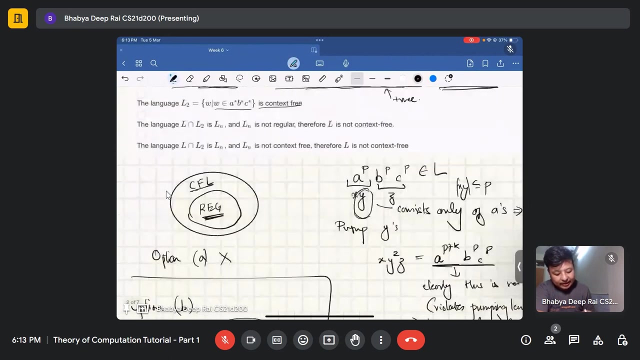 Right, It's not regular, That is true, And this is a subset of l. Does it make sense? Is it enough to say that? So let's look at option b. What option b means is okay. the language, l is not regular. 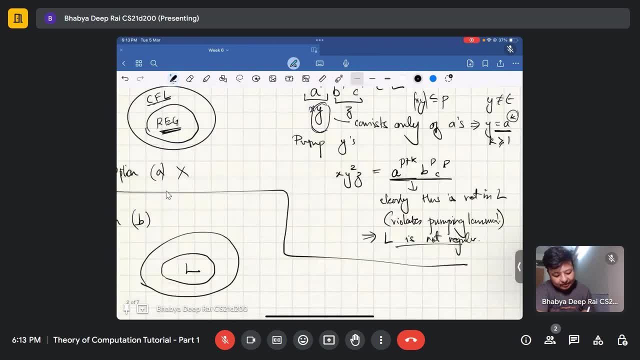 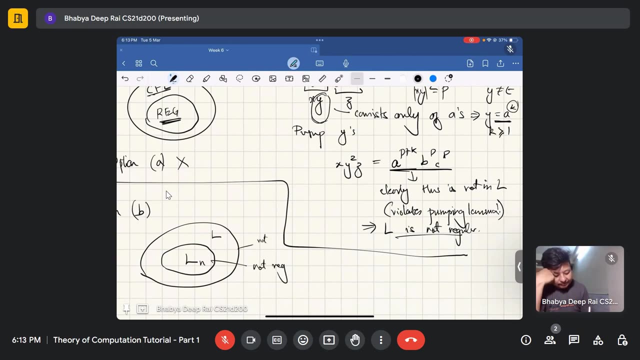 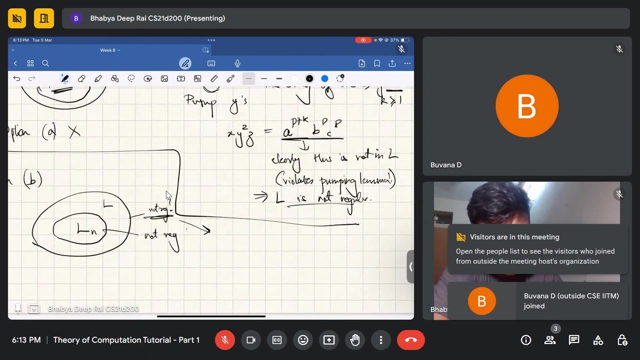 Because the language ln- okay, the language l- is not regular because the language ln is a subset. And since ln is not regular, then l is also not regular. That is what it's saying. Is that true? This can never be true. 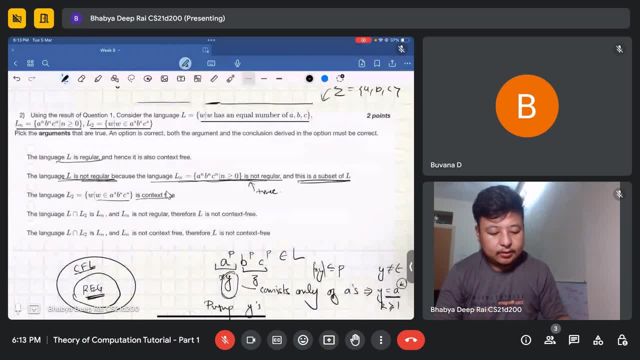 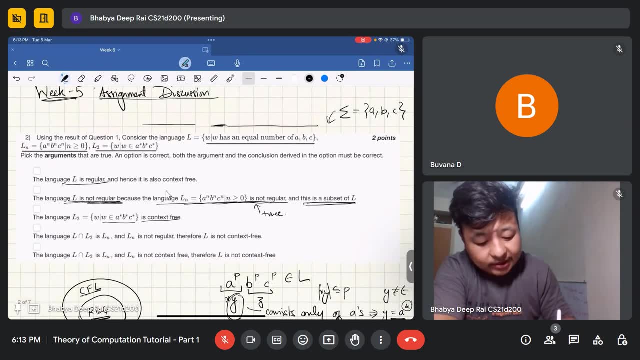 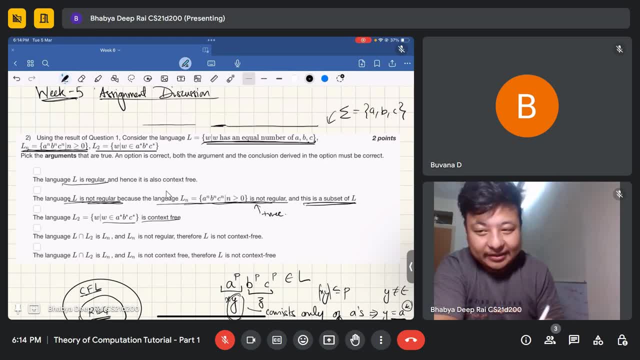 And a string which has equal number of a, b, c, but they are in sequence, Okay, a to the n, b to the n, c to the n, And l2 is all the strings which are of the form a, star, b, star, c, star. 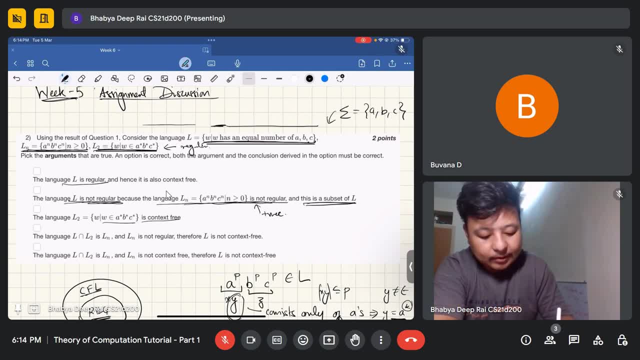 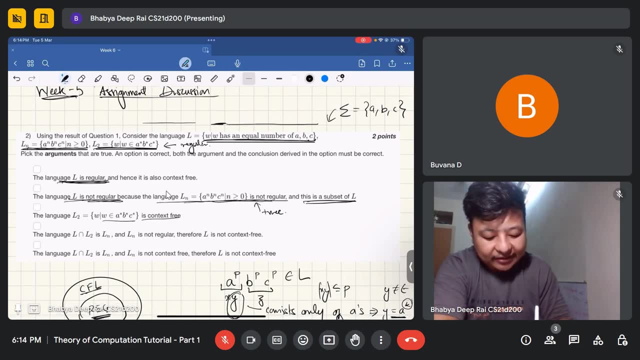 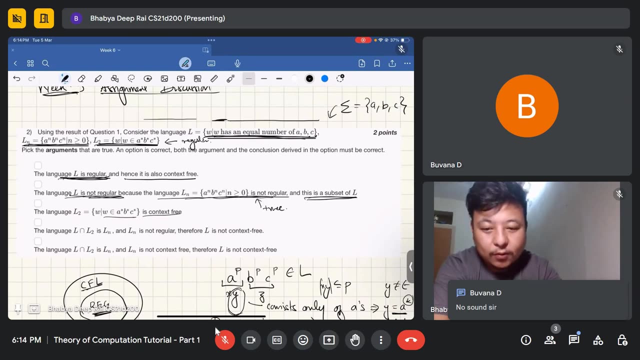 So this one is clearly regular And the question says the following: the language l is regular, hence it is also context-free. So, firstly, what is l? l? is this equal number of a's, b's and c? Oh, hello. 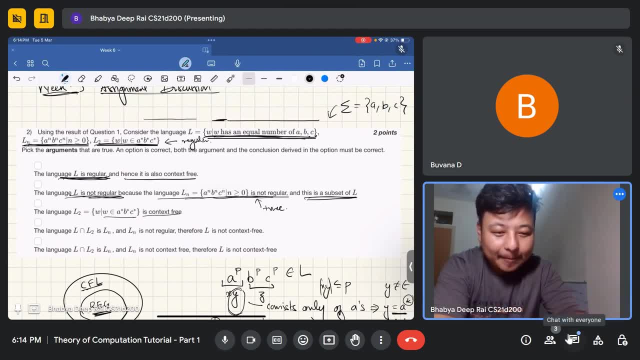 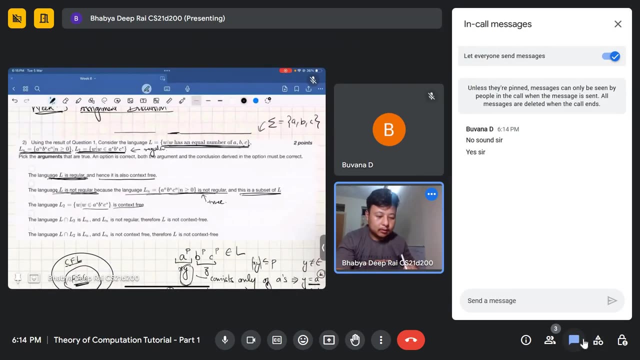 Hi Moana, can you hear me? Really sorry, I had put my mic on mute. Now can you hear me? Hello, hello, hello, oh, okay, okay, yeah, okay, I saw your chat. okay, good thanks. 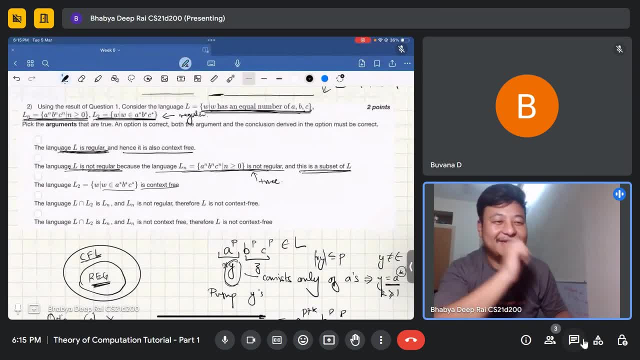 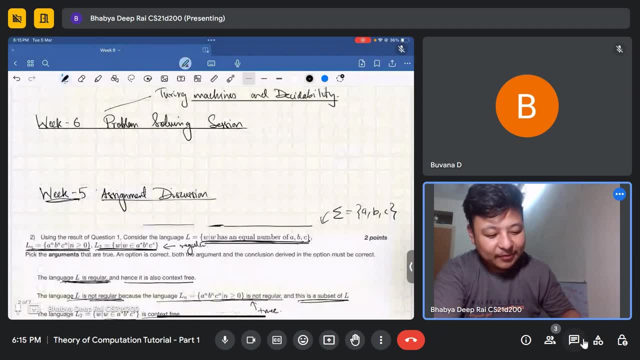 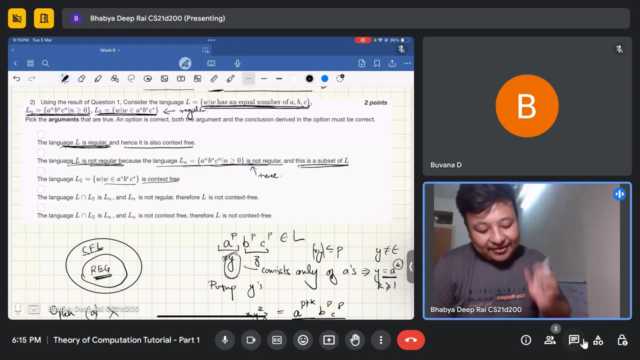 It seems there was a miscommunication on the timing. I think it got mixed up with the rescheduling last time, So so people didn't get notified properly, it seems. But thank you for showing up. Uh, okay, so let's, let's see. yeah. 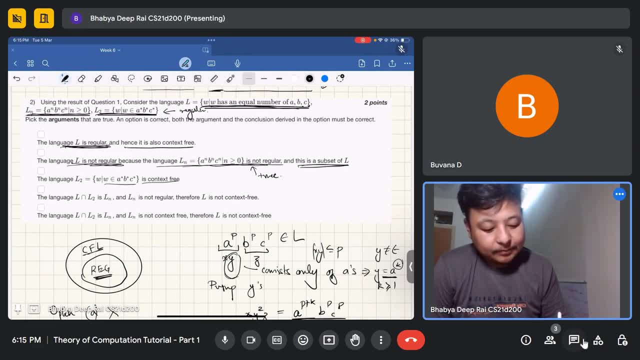 So, Moana, there are three languages given to us. okay, Equal number of a- b. so I'm discussing. I'll be discussing two questions from the previous assignment, then we'll move on to this week's haunted okay. 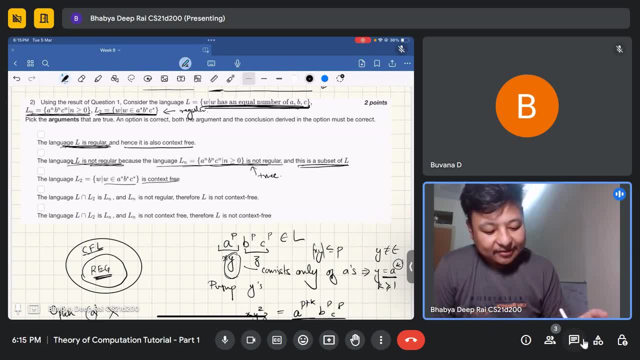 So the previous week's assignment said that there is this language which has equal number of a's, b's, c's And ln: is a to the n, b to the n, c to the n And l2 is a star, b, star, c, star. 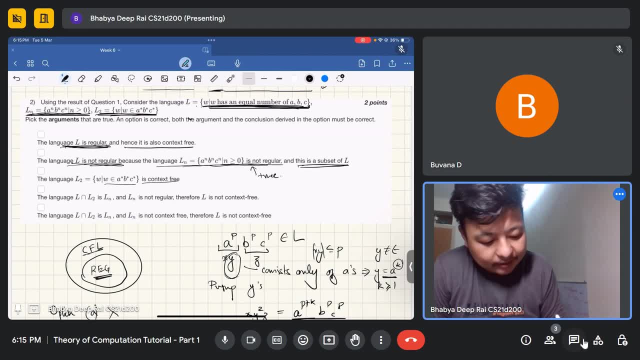 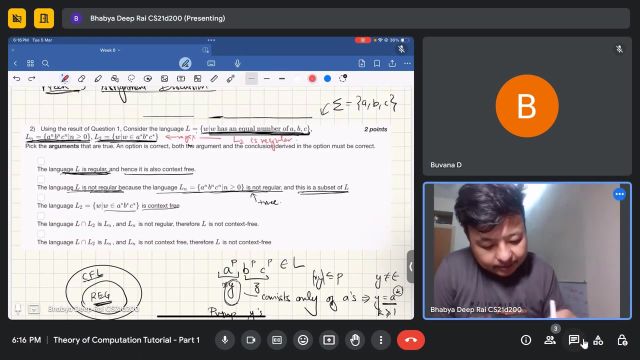 So this is this l2, okay, this guy l2, is represented using a regular expression. So definitely, l2 is regular. Okay, So let's, let's see what. what about the others? okay, Uh, okay, so the first one. 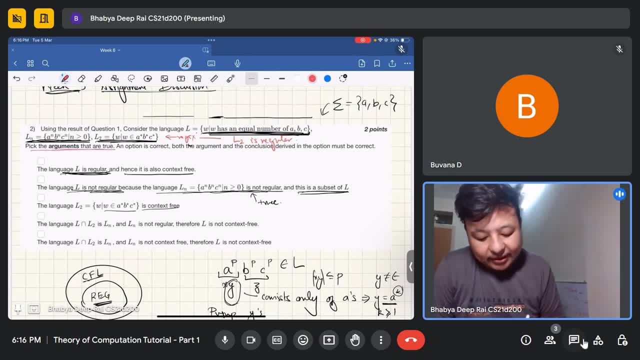 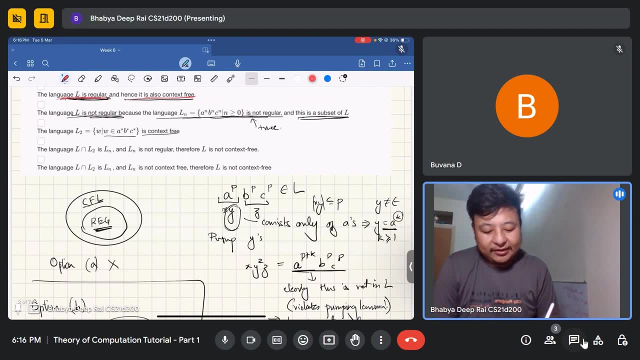 Uh the the. it says: pick the arguments that are true. okay, The first one says the language l is regular, hence it is also context-free. Well, first of all, is it true that you know? if your language is regular, it is also context-free. 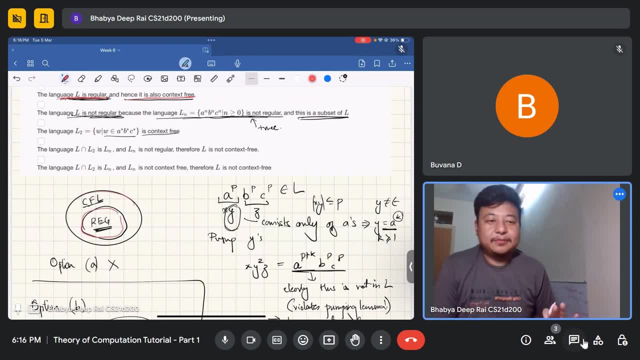 The answer is yes. Every regular language is inside a CFL. Okay Why? Because, uh, any DFA can be simulated by a PDA without using the stack. Because PDA is more powerful: it has a stack. If it decides not to use the stack, it can do anything. 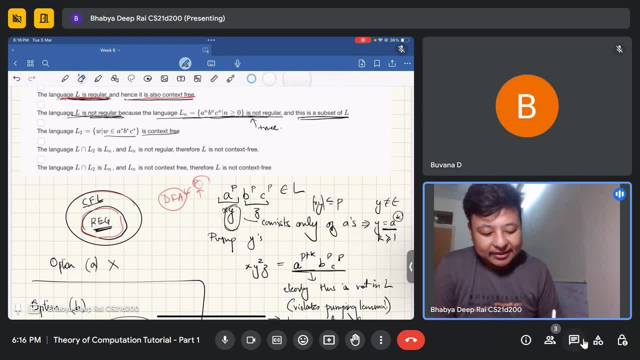 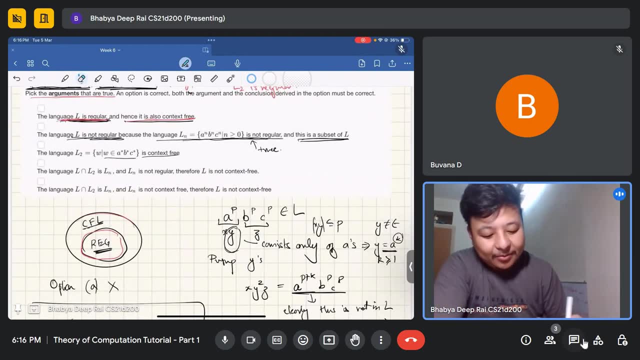 Okay, It can do anything that a DFA can do. So regular language is clearly under uh CFL. So in that way it makes sense to say: if a language l is regular, it is also context-free, But it is talking about this particular l. 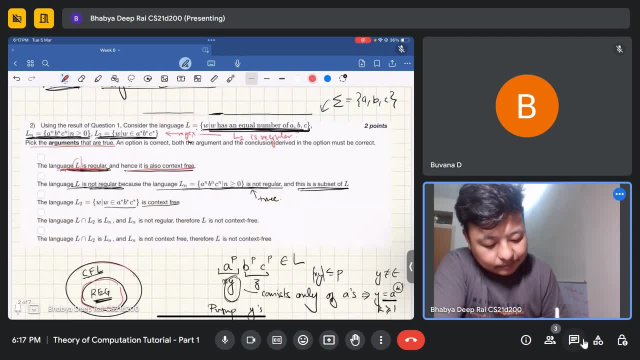 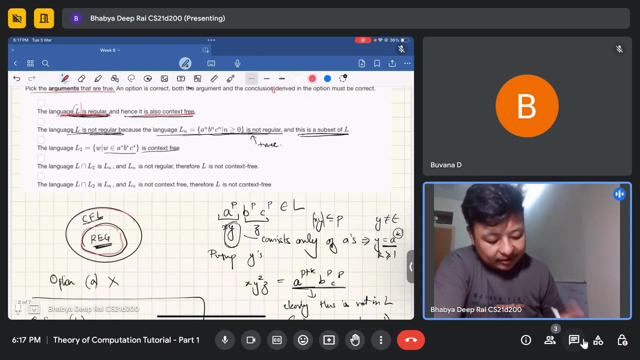 The l it talks about is this guy? Okay, Uh, w says that w has an equal number of ABCs. This language is it regular? That is the question first, And the answer is that it is. It is not actually regular because we can use the pumping lemma to disprove that it is regular. 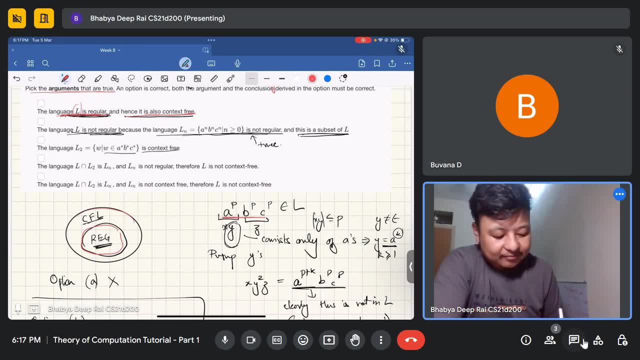 Okay, How do you do that? Well, take, say for example, a to the p, b to the p, c to the p. If this language was regular, then pumping lemma says: oh, you can actually split it into x, y and z, where x, y is at most p. 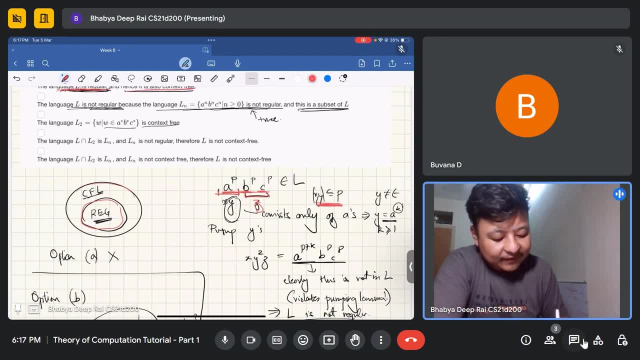 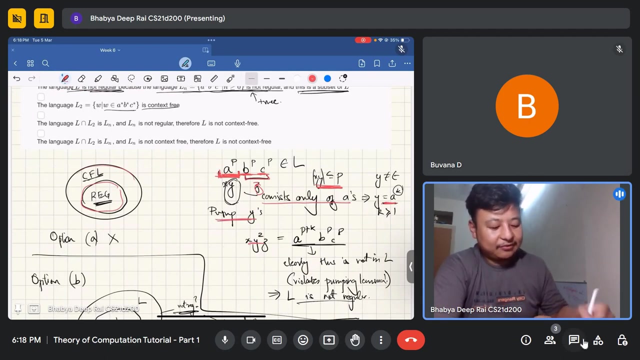 Length at most p. So if x, y is of length At most p, then x, y is entirely consisting of a to the p, is, or in other words, y consists only of is, y consists only of is. so let's say y is some a to the k. pumping lemma says: if you pump y, okay, and let's say I do x, y square, then I get more number of a's than b's and c's. and according to pumping lemma this should be in the language. 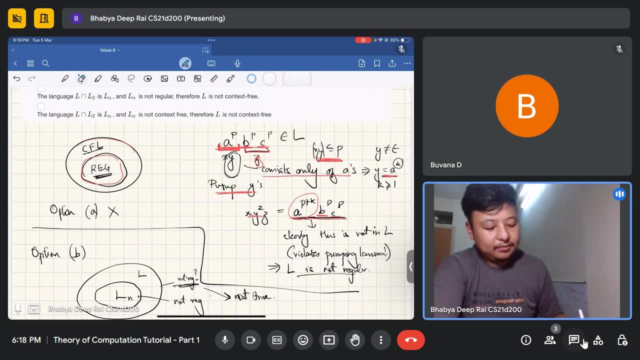 If this was, if the language was regular. But but clearly this is not in the language, because number of a's, b's and c's are not equal. So therefore l is not regular. Okay, So option a is not an option at all for us. 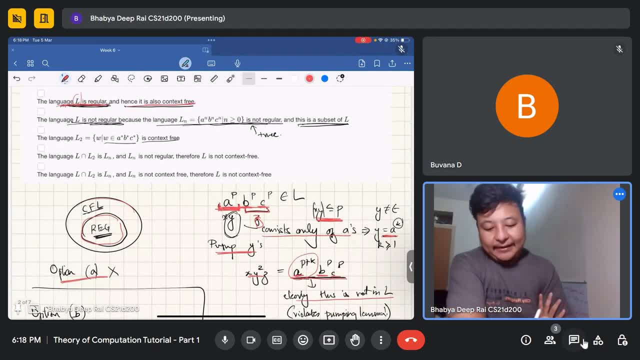 Let's look at the next option. Okay, A language, l, is not regular because the language ln equals a to the n, b to the n, c to the n. L is not regular and this is a subset of l. Okay, 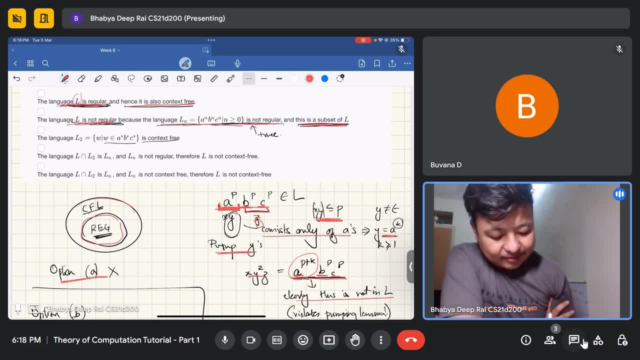 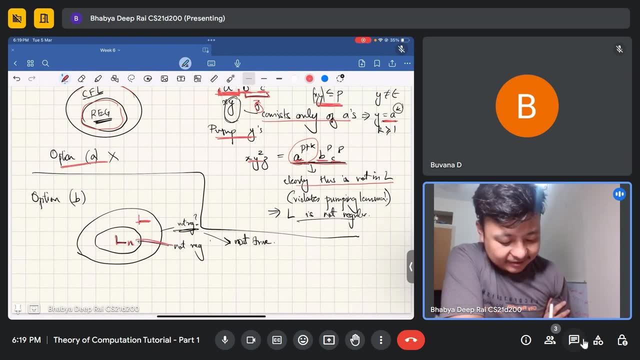 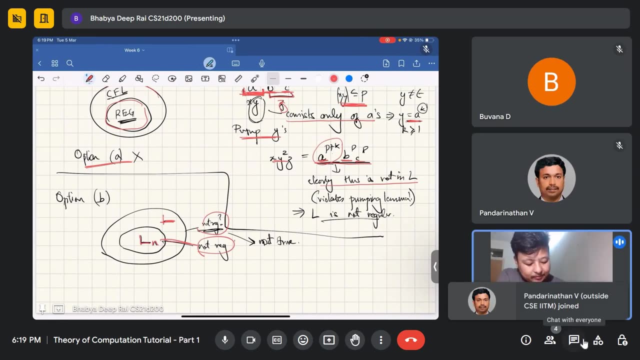 It is saying l is not regular because ln is a subset of l, ln is a subset of l and since ln is not regular, l is not regular. Okay, Does that make sense? Can can we get a counter example of this fact? 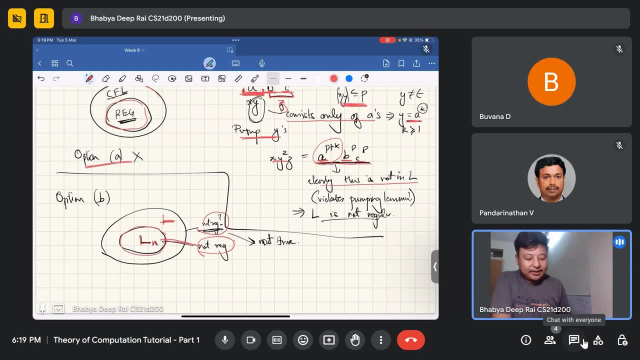 That is the question. The smaller set is not regular, but can it be that the larger set is regular? Do you have any counter examples for that? Can you talk about a smaller set which is not regular, but a larger set which is regular? 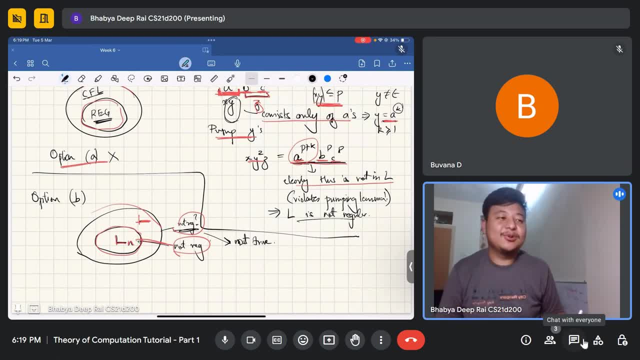 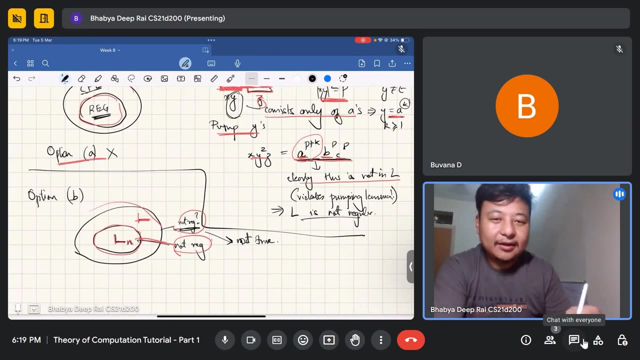 Okay. Or in other words, what is the largest language that is regular That you can construct? in some sense, This is visible, right? What I am writing, Is this visible? Yes, Yes, Okay, Okay. So it is visible, right. 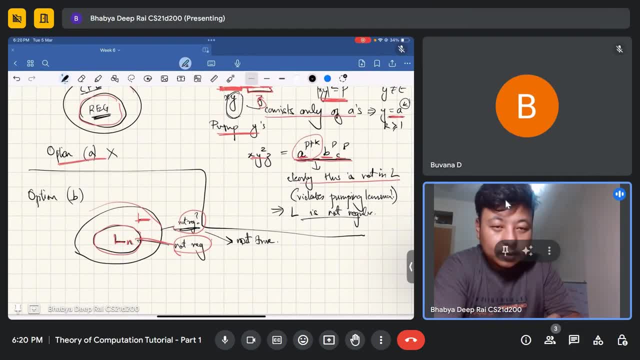 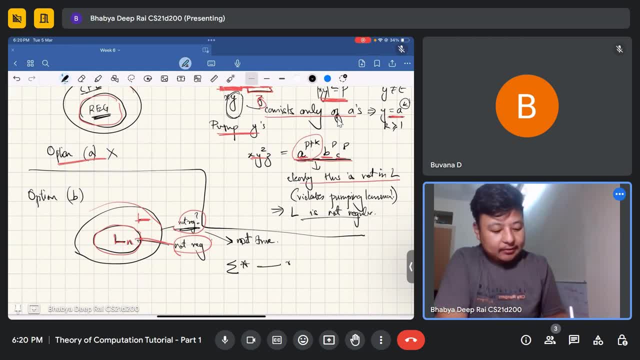 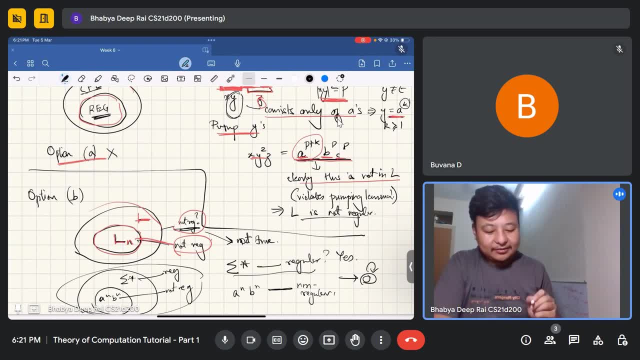 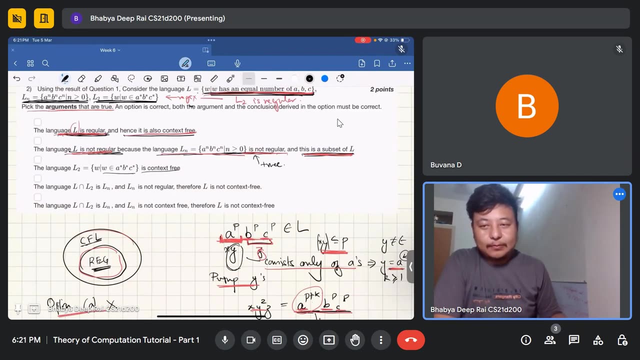 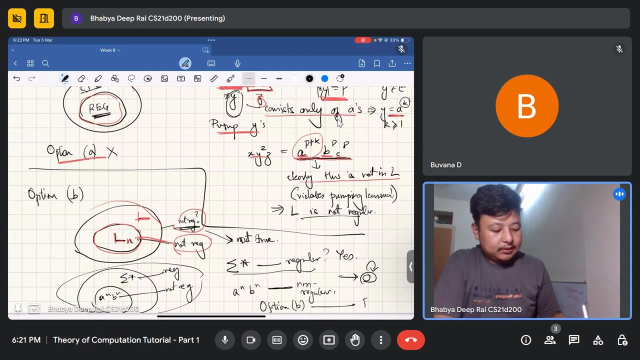 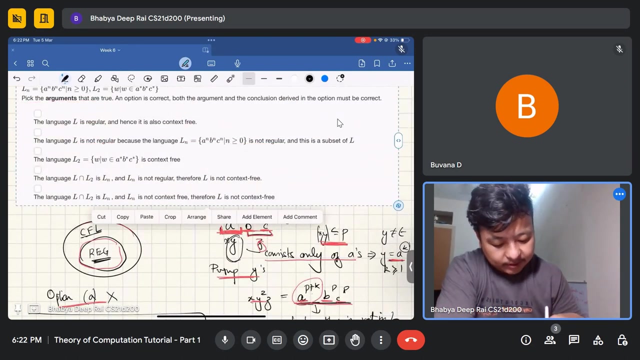 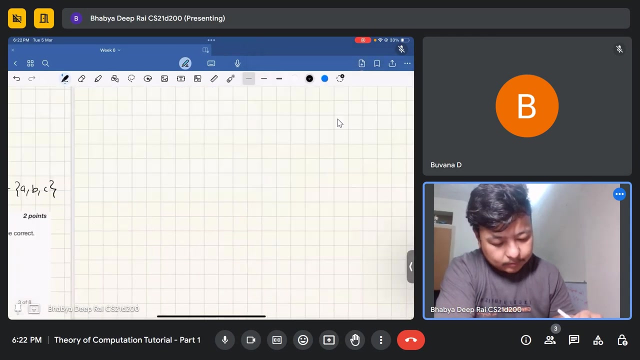 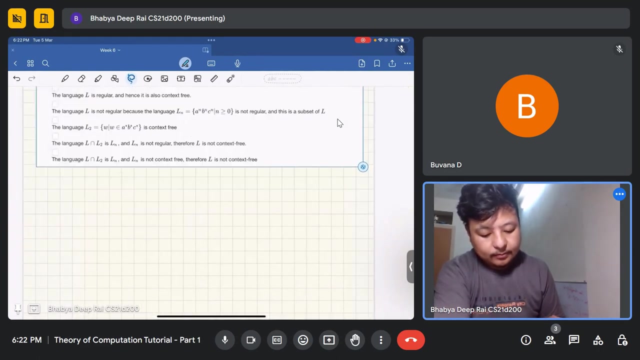 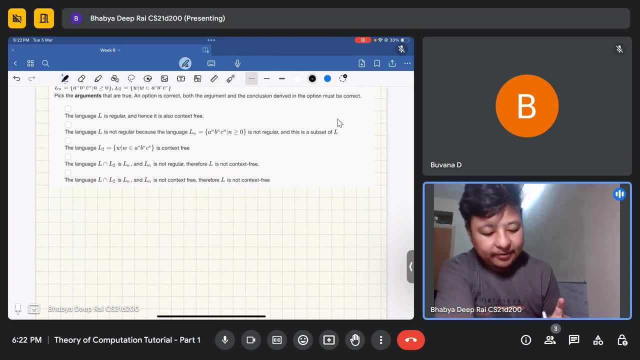 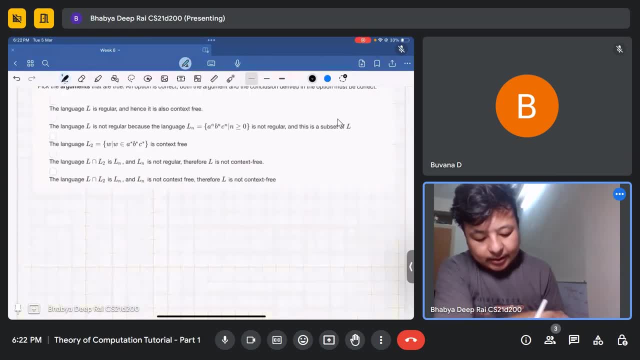 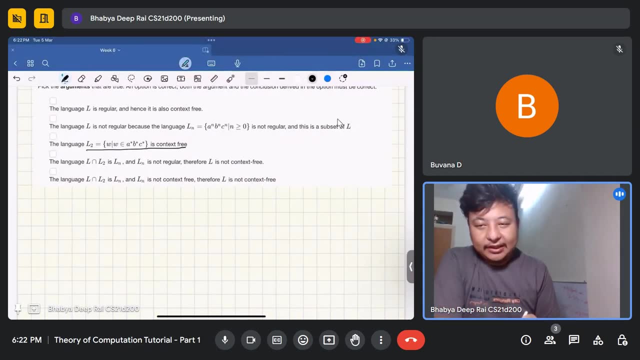 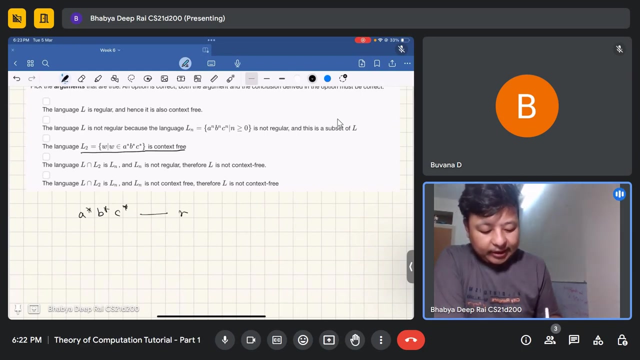 uh. so next they are saying: the language l2 is context free. the language l2, w in a star, b star, c star is context free. uh, so is this true? well, a star, b star, c star is already regular and any regular language is context free. like i said, regular language is nothing, but those which have dfa's. 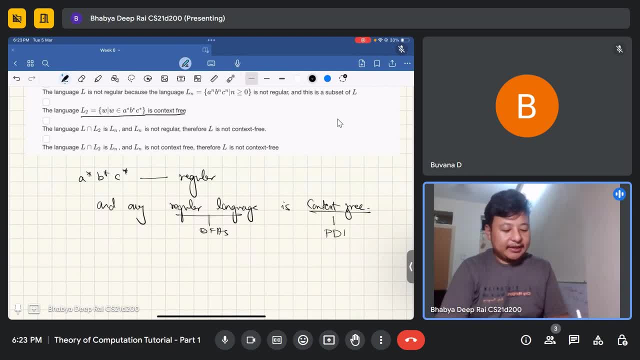 context: free languages are nothing but those which have pdas, and pdas are nothing but a dfa's with stack. and if you uh, anything that can be computed by dfa can be computed by a pda, because you just don't use the stack at all. you just don't use the stack at all and it is as powerful as a dfa. 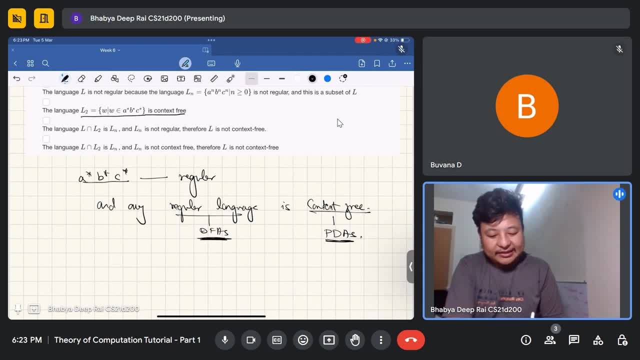 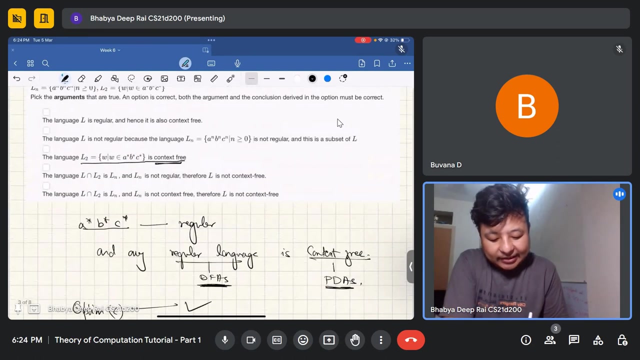 so if a to this b, a star, b star, c star is regular, then it is also context free, okay, so option c is correct. okay, now let's see the language. l intersection l2 is ln and ln is not regular. therefore l is not context free. so let's see l intersection l2. 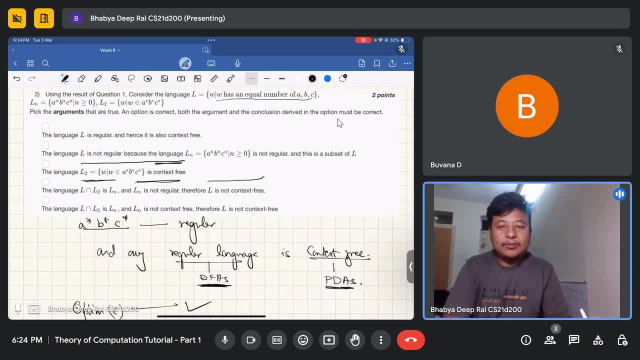 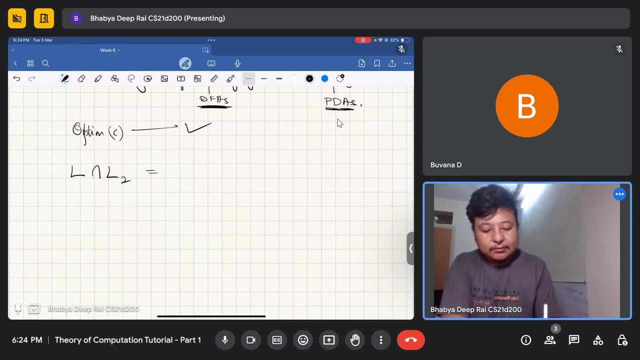 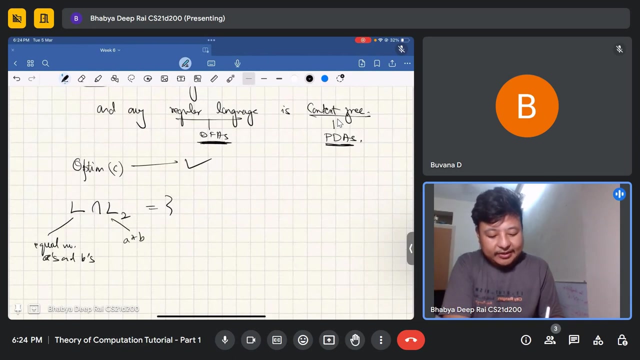 what is l? l is w such that w has equal number of a, b, c and l? l2 is a star followed by b star, followed by c star. okay, oh sorry, l intersection l2, l is equal number of a's and b's. that's right, right, yeah, and l2 is a star followed by b stars. 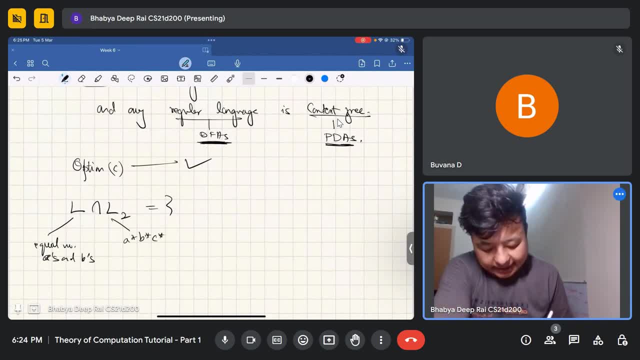 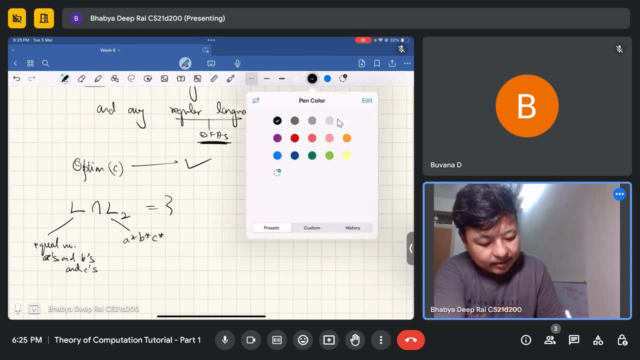 followed by c star. now l2 is regular. we know that. and uh, equal number of a's, b's and c's is non-regular. we've already shown that. we've shown that this is non-regular and l2 is regular. you've seen that right just now. 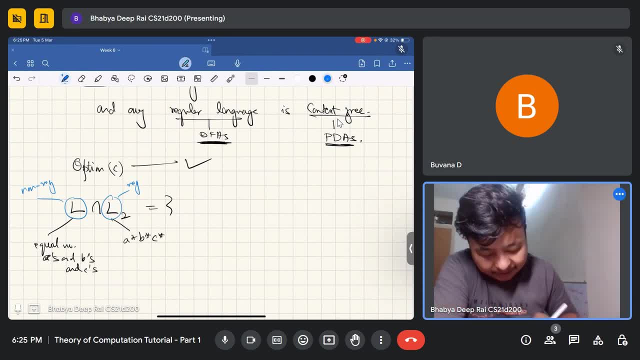 now, what is the intersection? what is equal number of a's, b's and c's? this could be something like a, a, b, b, b, c, c, or it could also be like a, b, c, a, b, c, or it could also be a, c, b, c, b, a and then again abc. 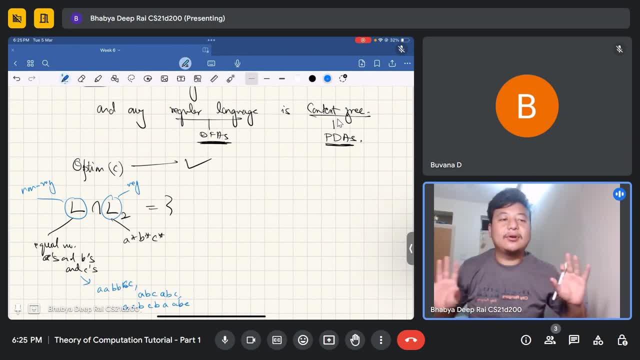 anything like this is allowed: a's, b's and c's could occur in any order. but what does a star, b star, c star say? star b star says: uh, first a's will show up, any number of a's, then any number of B's will show up, then any number of C's will show up, right. 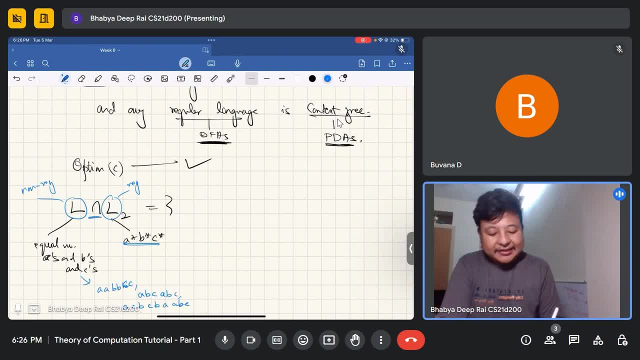 Now, what do you have? You are looking at their intersection. What are the languages which are common between this and this? This is things like A, B, B C, A, A, B, C, C, and so on. 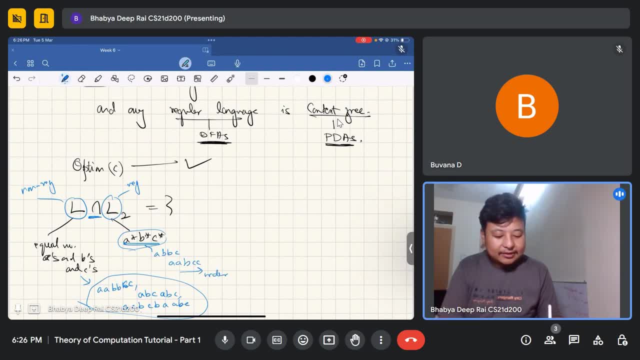 This talks about order and this talks about number of elements, Number of symbols. Number of symbols should be same: Number of A's equal to number of B's equal to number of C's. Their intersection will be all those strings that has A's followed by B's followed by C's. 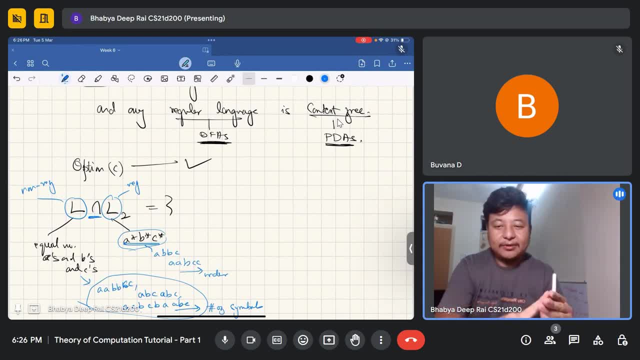 Additionally, number of A's equal to number of B's equal to number of C's. right, Both the behaviors are combined. So what do you have? You have all strings Of the form A to the N, B to the N, C to the N. 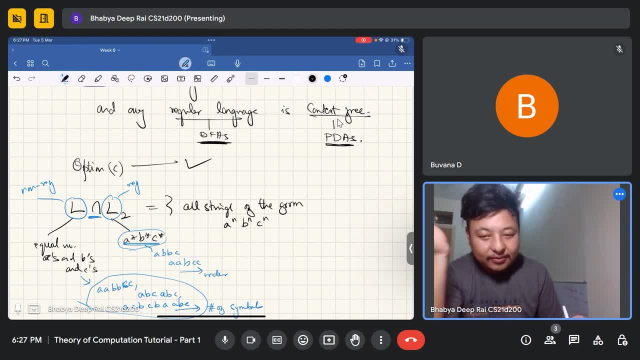 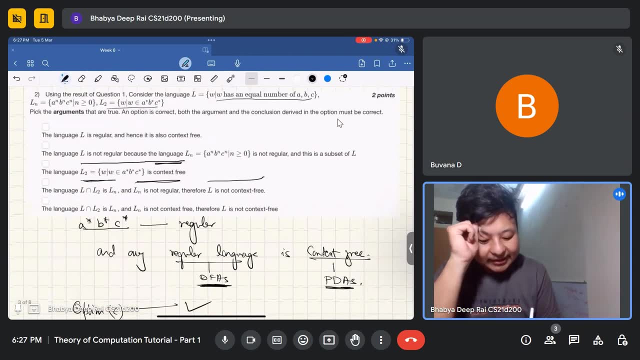 B should follow A, C should follow B and their numbers should be equal. So that is the intersection. So what is this? What their claim is? it is LN. that is true. LN, if you look at, is A to the N, B to the N, C to the N. 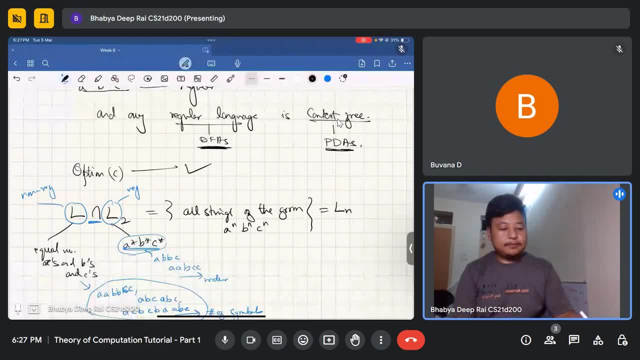 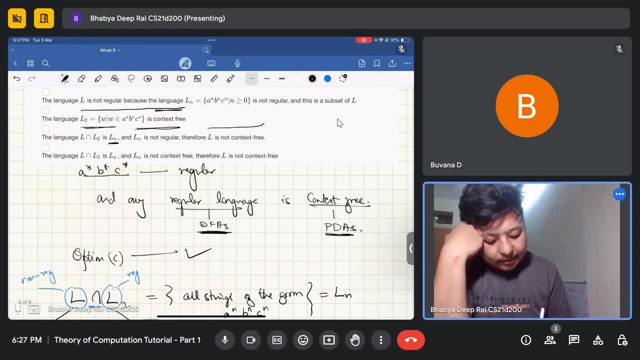 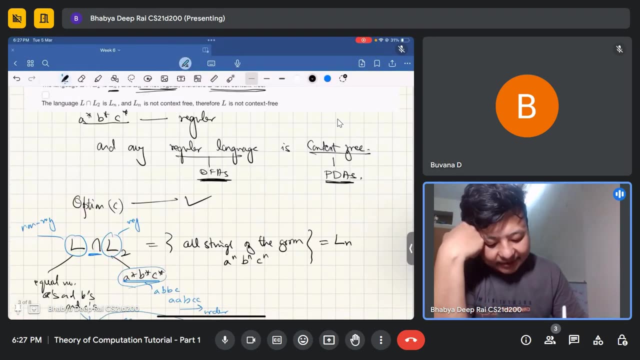 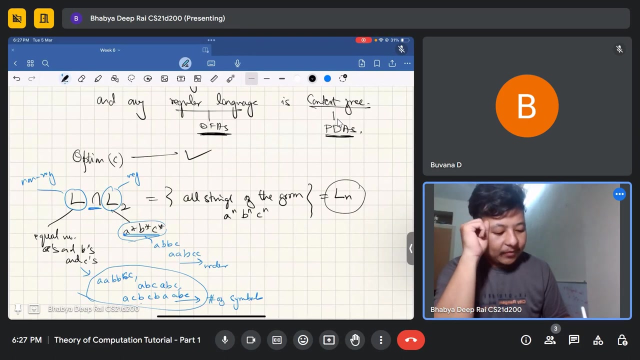 So this part is true. Clear, This part is definitely true. Next, LN is not regular. Therefore, L is not context-free. That's what they are saying. What is LN? This guy is it not regular? Yeah, it's true. 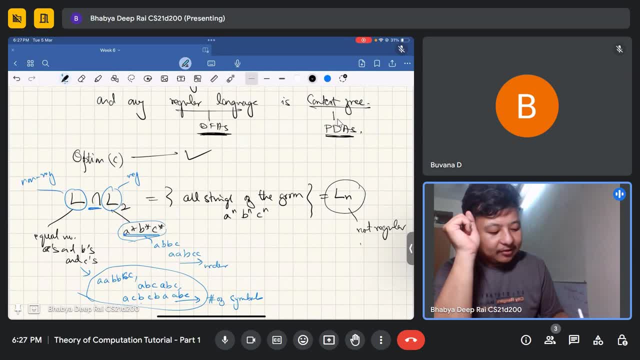 It is not regular. Additionally, it is not context-free also. You may have seen it in the lectures that A to the N, B to the N, C to the N is not context-free, Whereas A to the N, B to the N is context-free. 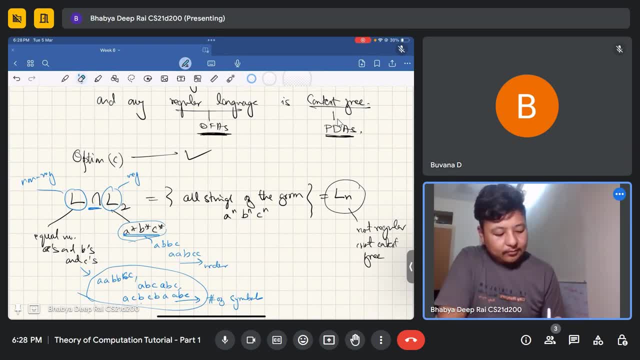 Now the question is: is it because it is not regular? you can say that. if you say that, oh, since LN, LN is not regular, LN is not regular, L is not context-free, Can you say that LN is not regular? 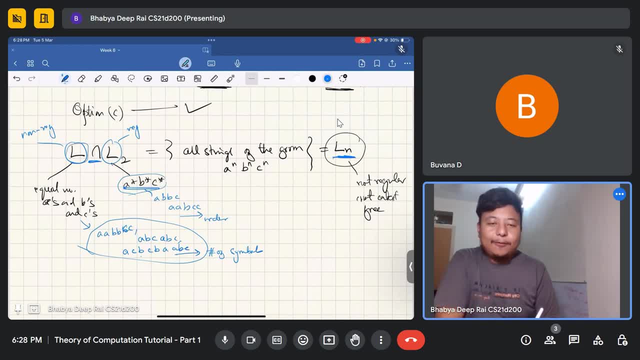 so L is context-free. Can you say that Such kind of a claim does not? we've never seen such kind of claim, So it's already it makes sense to suspect this. It is kind of suspicious to talk about this. 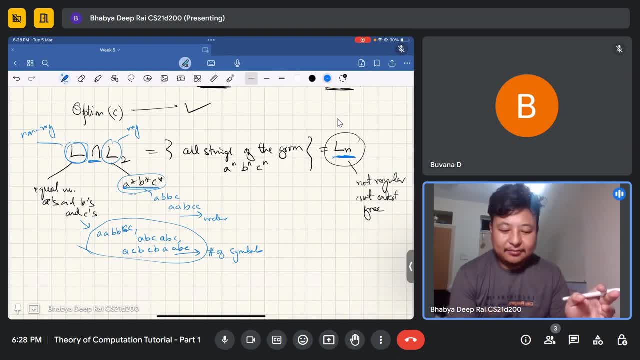 this way. And but LN is not regular. Say LN were context-free and we already know that this is context-free, Right And intersection of context-free languages is also context-free, Then everything is well and good. So, even though this was not regular, 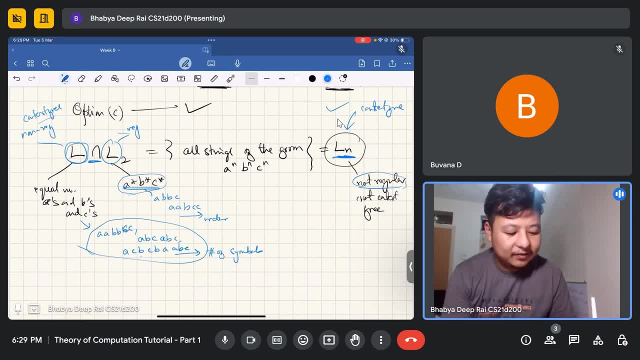 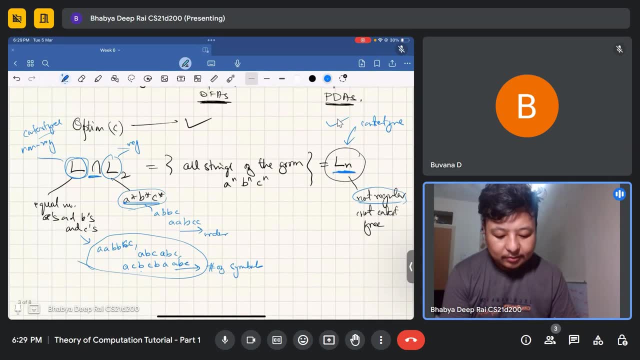 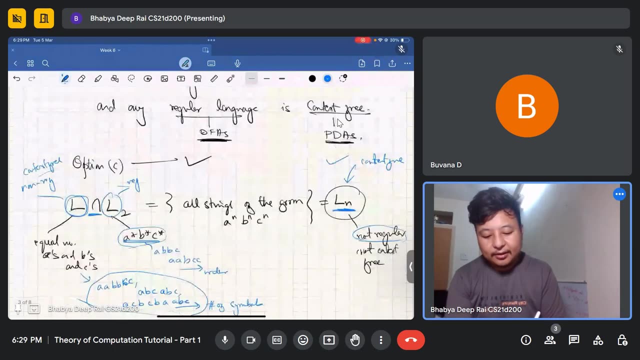 and it was. and let's say it is context-free Even though this is not regular, then everything is holding, It's all good. So it does not make sense to say L is not context-free, Okay, So option. 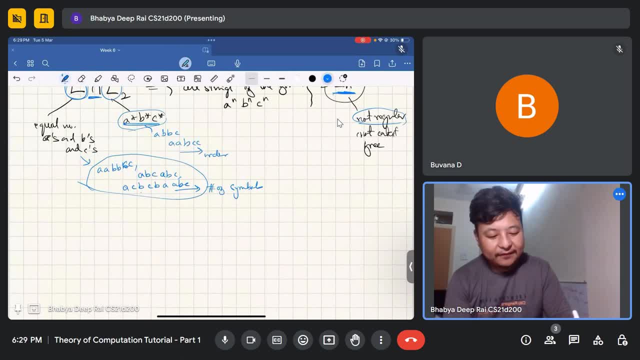 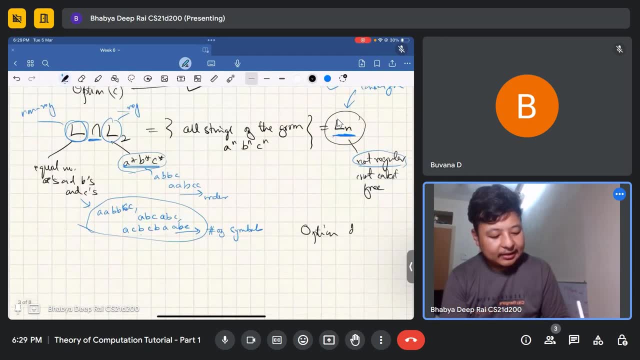 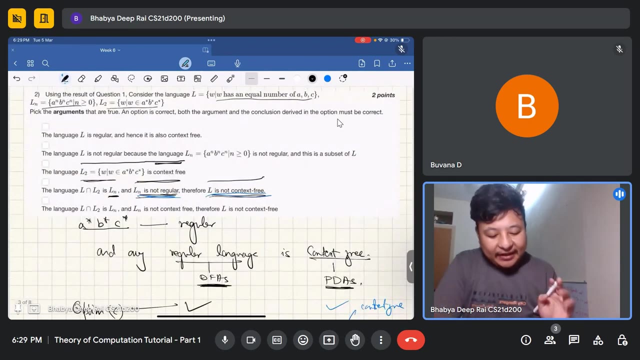 so there, we have a contradiction, We have a, but if you are not convinced, we are going to look at the next option. Okay, Option D is not true, But finally, we will look at this option. Okay Again, L intersection L2 is LN. 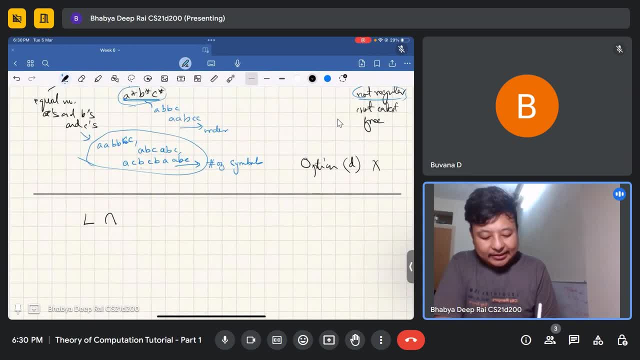 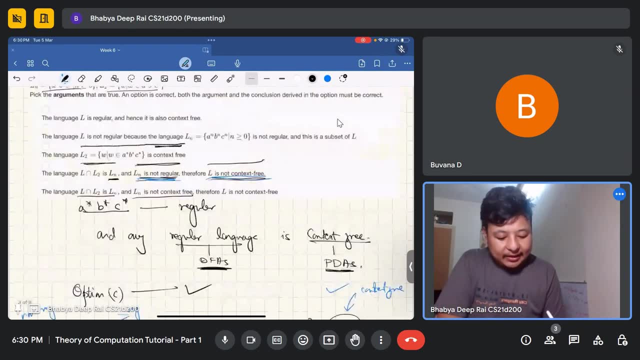 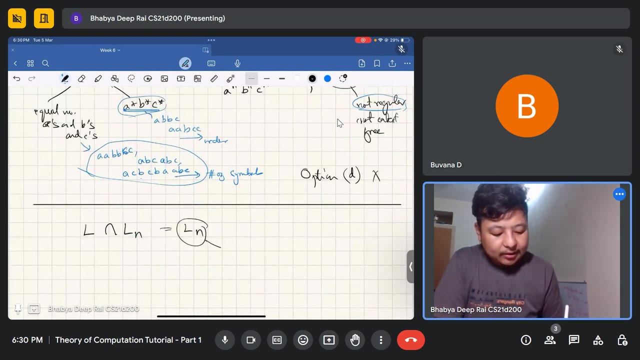 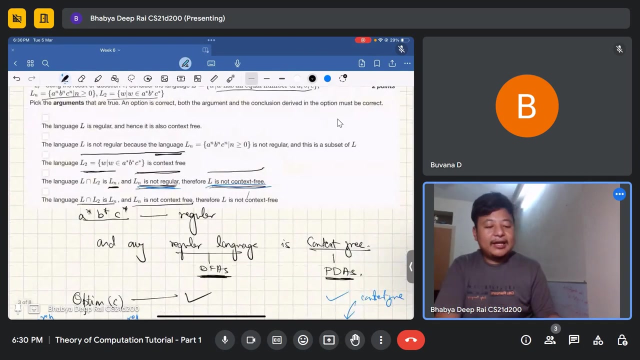 and LN is not context-free. Therefore, L is not context-free. L intersection LN, which is nothing but A, to the N, B to the N, C to the N, which is nothing but LN. Okay, this is not context free. therefore, L is not context free. therefore, L is not context free. 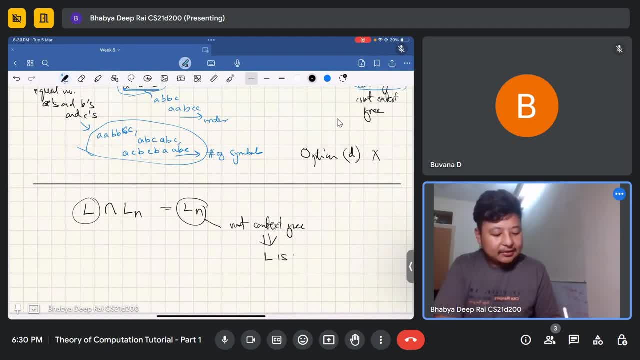 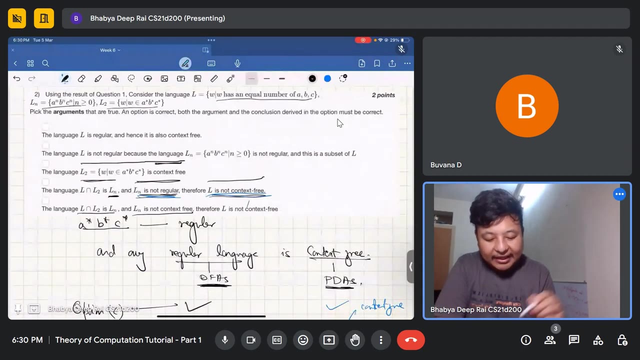 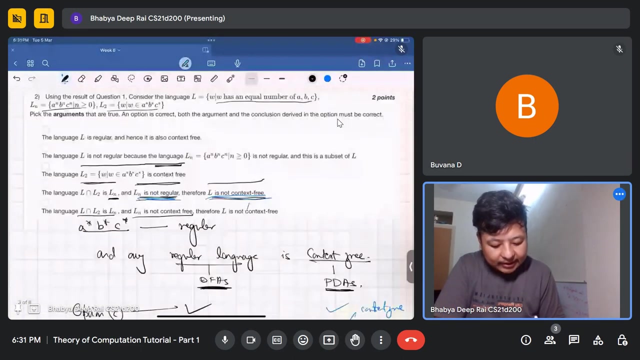 this is not context free. this means L is not context free. now, does this make sense? yes, why? because Ln is again to remind you, Ln is the a to the n, b to the n, c to the n right, which is, no wait, not Ln here. L intersection L2. really sorry, L intersection L2. 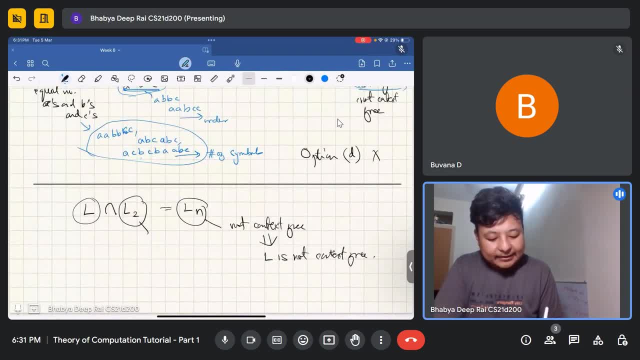 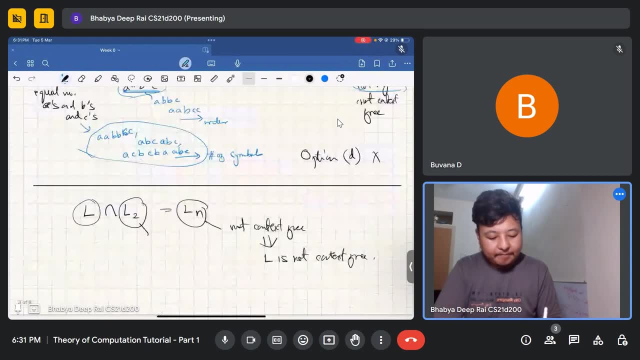 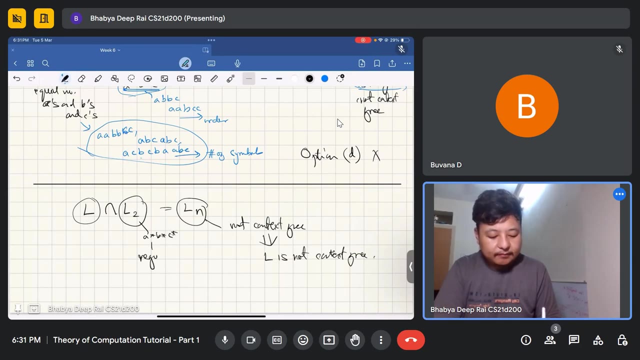 okay now L2 is defined as ac star, b star, c star, which is regular. if it is regular, it is context free. also, what we know from the lectures is that intersection of CFLs gives a CFL. so if L is a CFL then definitely Ln equals L intersection. L2 is also a CFL. 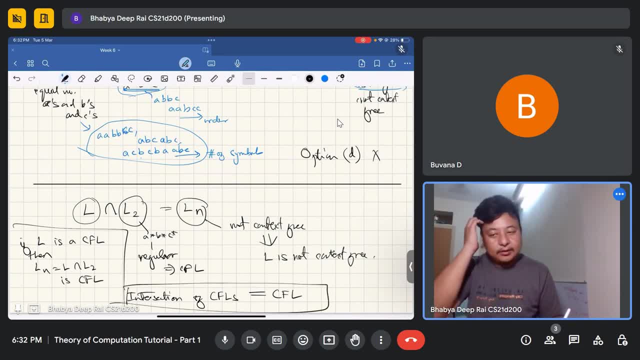 because of this theorem: closure property right. but that is not the case. but we are saying Ln is not context free, it is not a CFL. this is a question, right? so clearly there is a contradiction. since Ln is context free, it must be that since, and since Ln is context free and L2 is also context free, it must be that L is also. 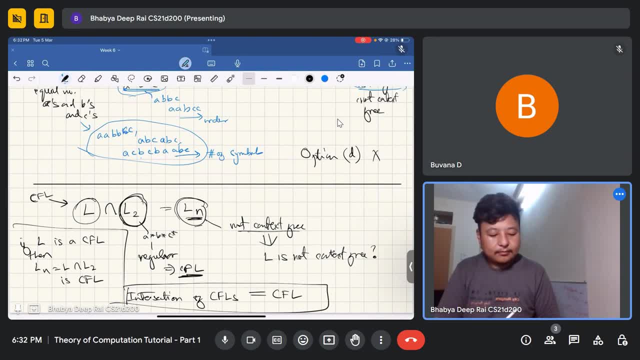 context free. so Ln is not context free. but Ln is not context free. okay, and this is. L2 is context free, then L is not context free, because if L was context free, then Ln would become context free, right, because intersection of context free languages is another context-free language. 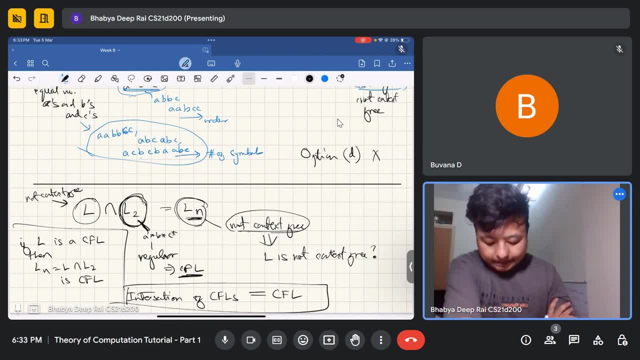 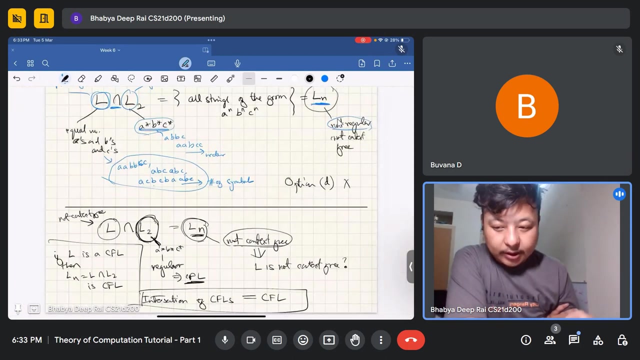 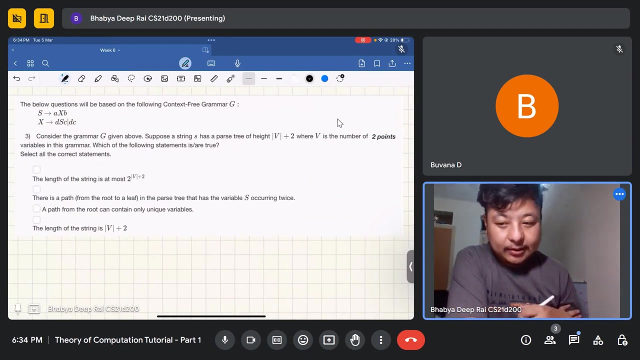 okay, is that clear? yeah, Hello, Okay, so it's clear. right, Gowana? Just let me know if you want me to repeat anything. Okay, so we'll look at the next another question in the previous week's assignment and then we'll move to this week's thing, okay? 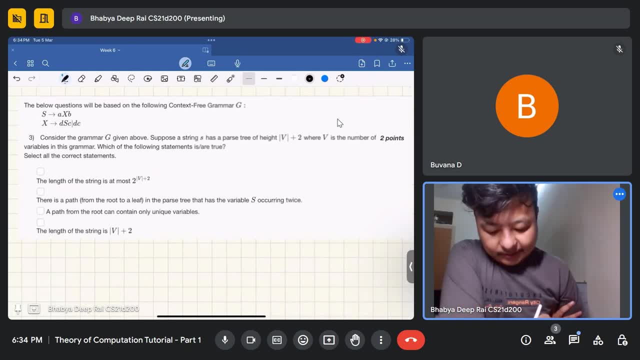 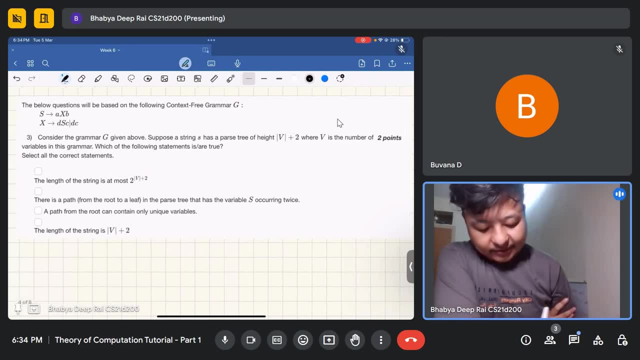 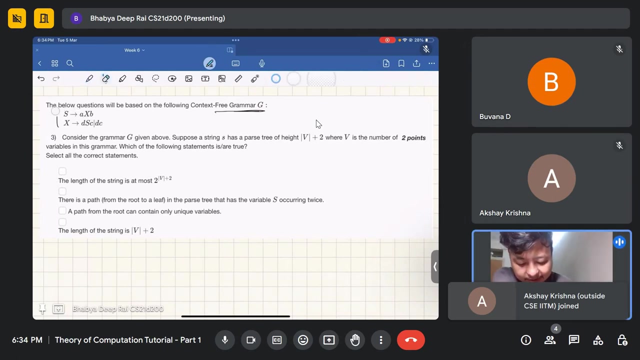 So here's the question. okay, It's a simple question, rather. So here's the question. S is so here's the grammar given to us. Okay, here's the grammar given to us. S generates, okay, S generates EXB and X generates BSC or BC. 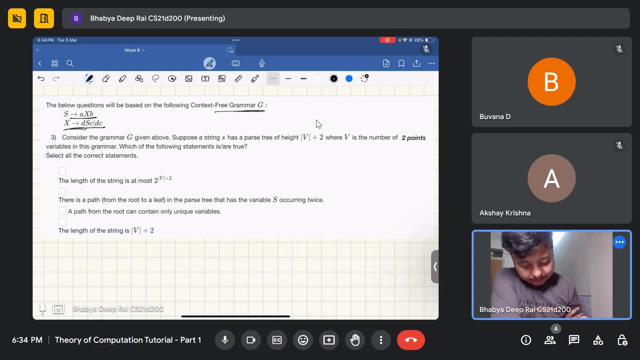 Okay and okay. Can you explain? Can you identify the variables and terminals here in this grammar? Oh, Akshay is also here. Terminals A, B, C, D. Terminals is A, B, C D. 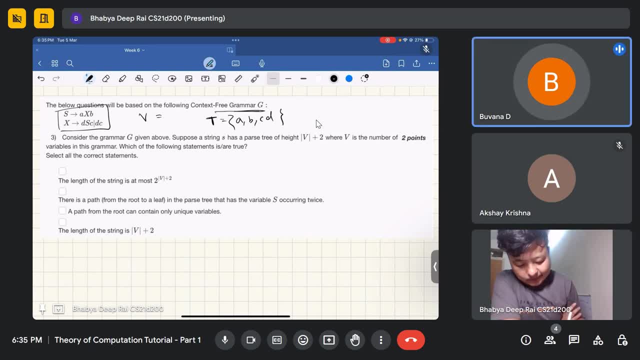 Good Variables. Variables: starting variable S and X. Good yeah, Starting variable and X. Okay, good, So let's move on. Consider the grammar G given above. Suppose the string S has a pass-tree of height V plus 2,. 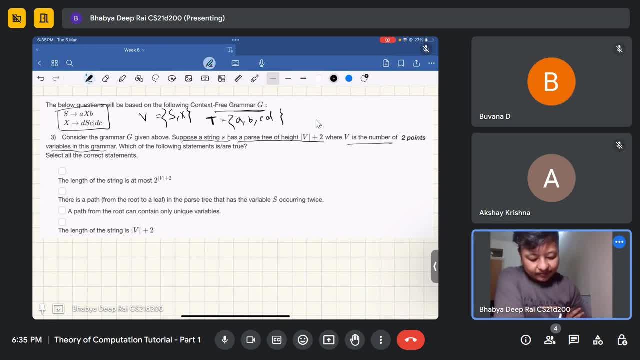 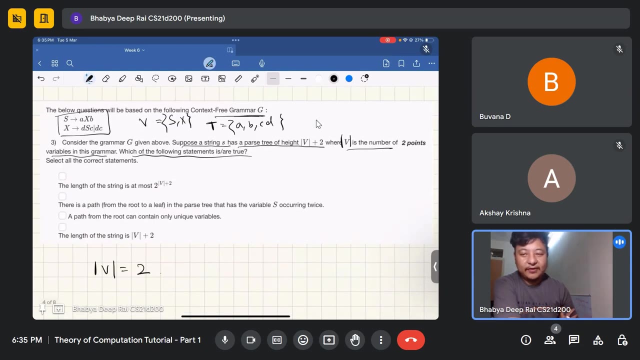 where V is the number of variables in this grammar. Okay, it should be So. it's a number of variables in the grammar. Which of the following statements are true? So, firstly, we have: this is equal to 2.. Number of variables in this grammar are 2.. 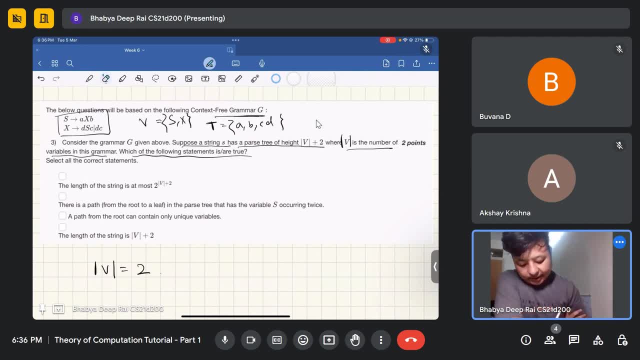 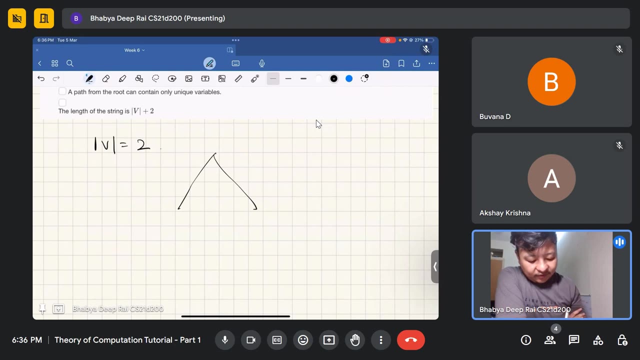 So the cardinality of V is 2.. Okay, So now it says: suppose the string S has a pass-tree of height V plus 2. You've all seen what a pass-tree is right? It looks like this: 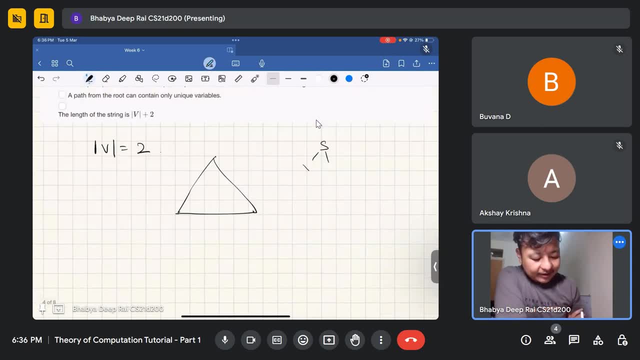 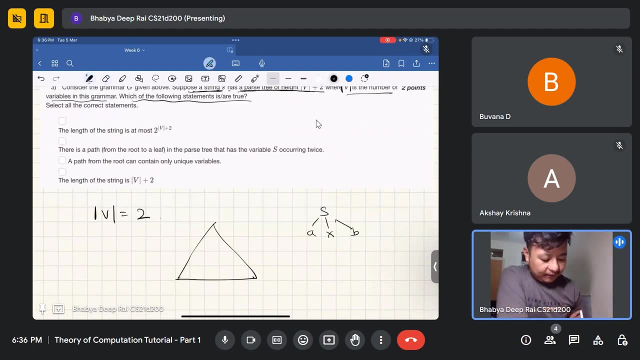 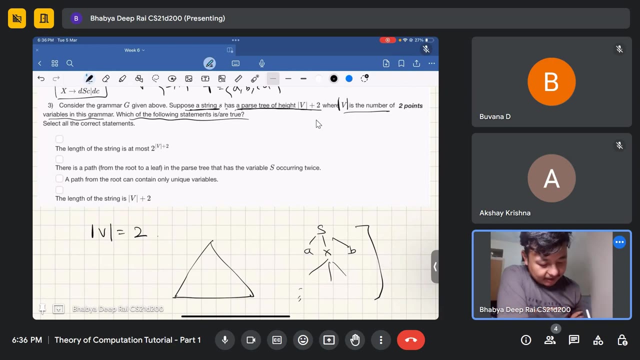 You know, you have a production S, And after S you get, say X, what A, X B, And from X you get something else, and so on. What we have is the height of the pass-tree is size of V. 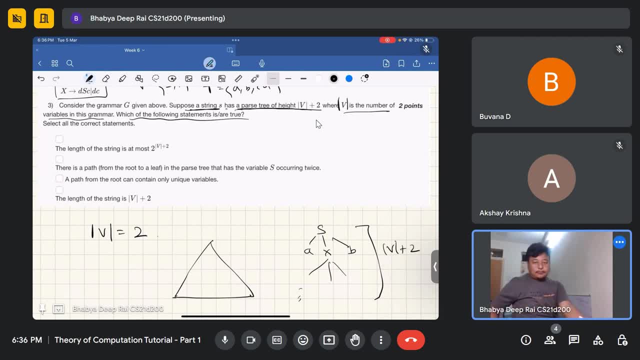 So we have V plus 2.. Okay, And what is size of V? 2 plus 2, which is equal to 4.. 4 is the length of the pass-tree. now, height of the pass-tree. Okay, Now, what are they saying? 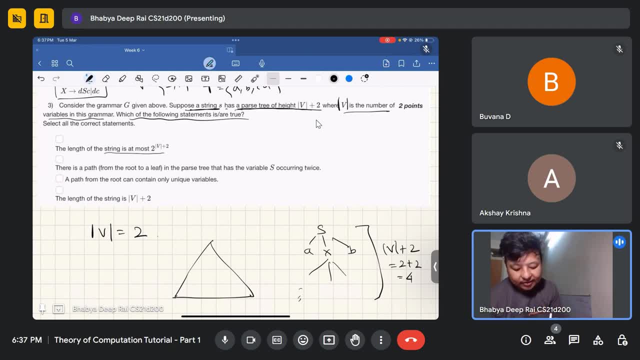 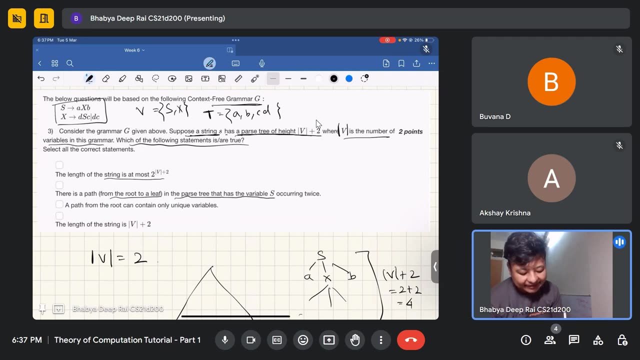 They are saying the length of the string is at most 2 to the size of V plus 2.. Okay, That is one thing. Next is there is a path from root to leaf in the string, The pass-tree that has the variable S occurring twice. 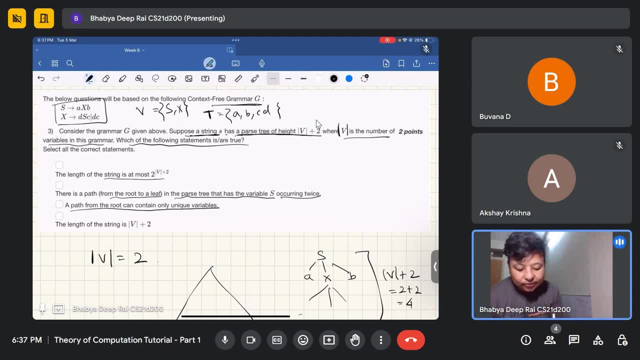 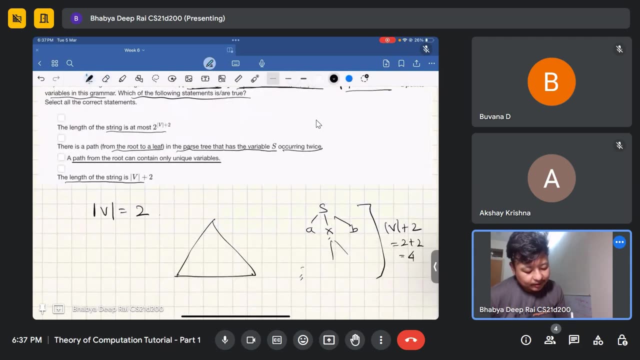 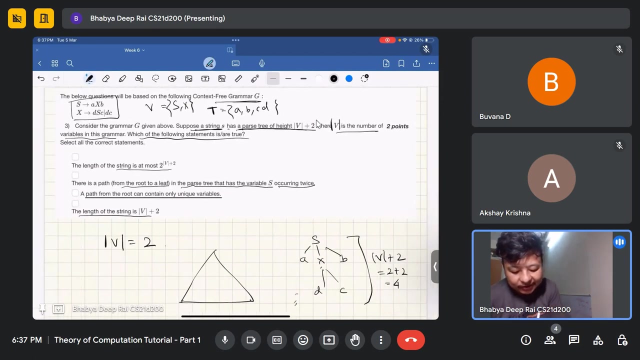 Next, a path from the root can only contain unique variables. Next, the length of the string is V plus 2.. So let's see X could generate DC. but if X generates DC, okay, if you look here, X could generate DC. 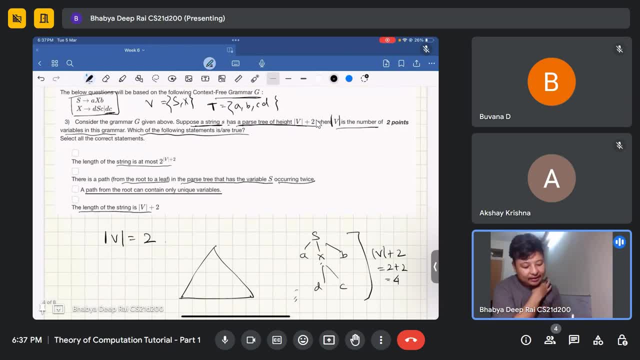 but if X generates DC, then our computation has stopped. Our output is A, D, C, B, Right, But the height is not 4 here. Height counted with the number of edges, okay, not the number of nodes. So 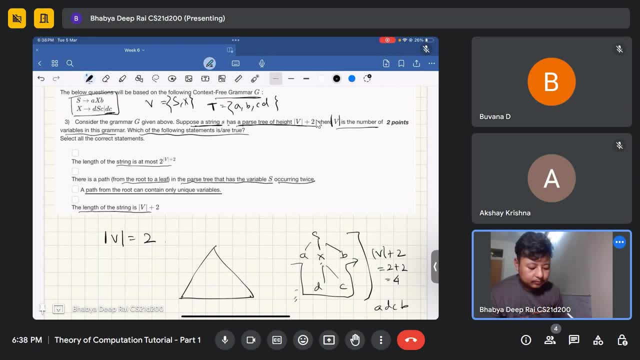 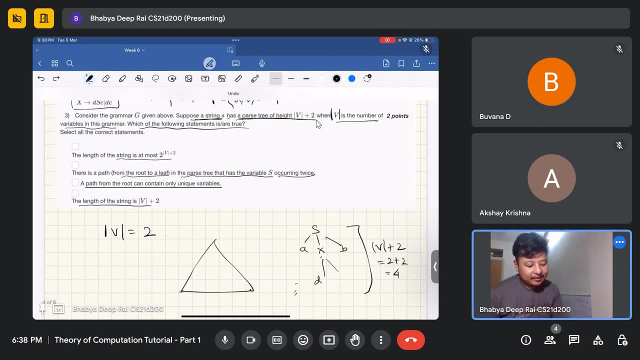 so okay. So X cannot be DC. X cannot generate DC. It needs to generate something to give a greater height, So it needs to generate D, S, C, Okay Now. okay Now, since we have an S here, you can always generate more height. 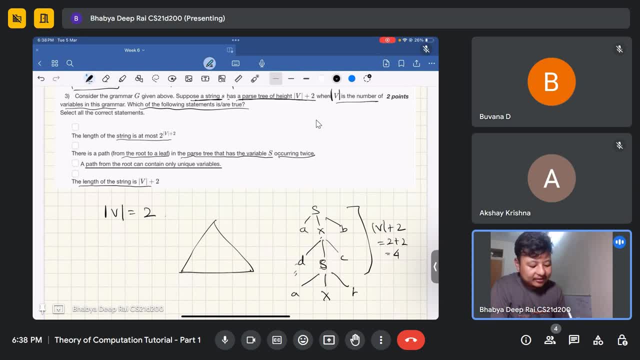 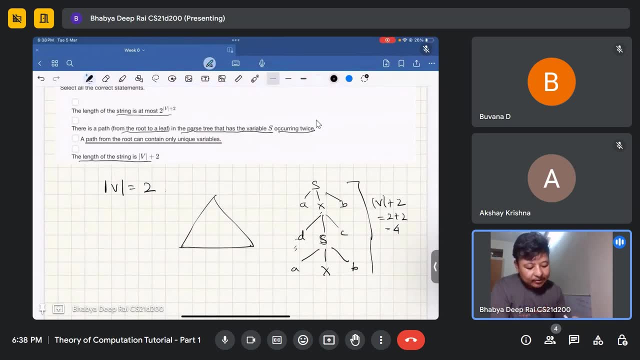 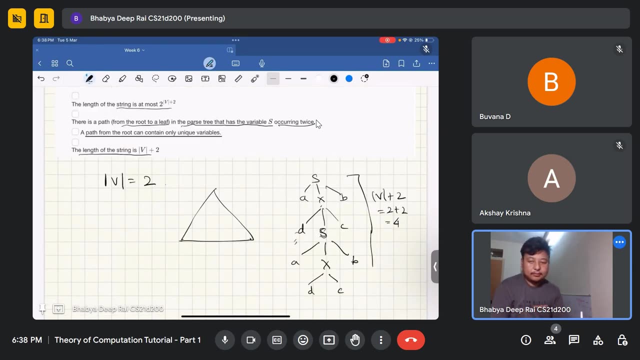 Now S will again generate A, X, B, because that is all that it can generate Right Now. what is the height? The height is 3.. X can only generate now D, E and C. Okay, 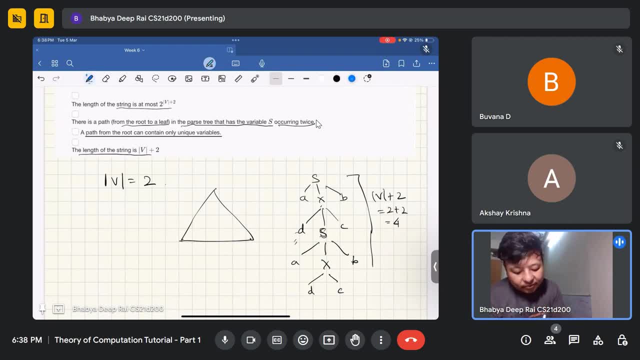 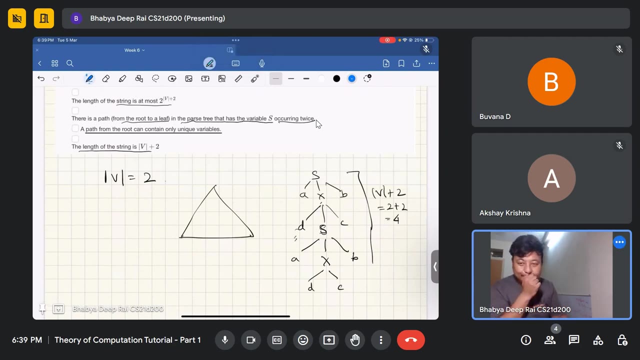 So, firstly, there is a path from root to leaf in the path tree that has variable S occurring twice. That is always the case, As you can see. that is always the case Because there are only two points. In other words, this can be seen as an application of Pigeonhole Principle. 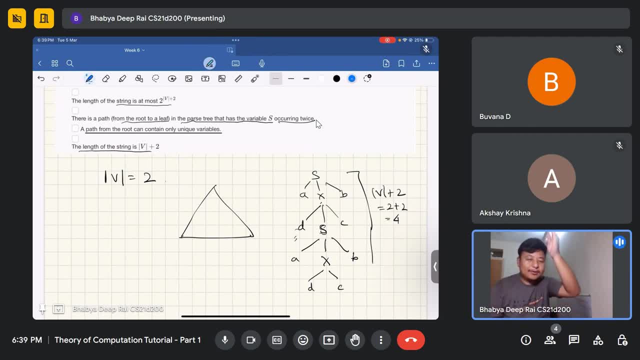 There are, you know, V plus 2, many more than V, many variables in the height of the path tree Right. And there is some path, which means there is some path of length, V plus 2.. And how many variables are there? 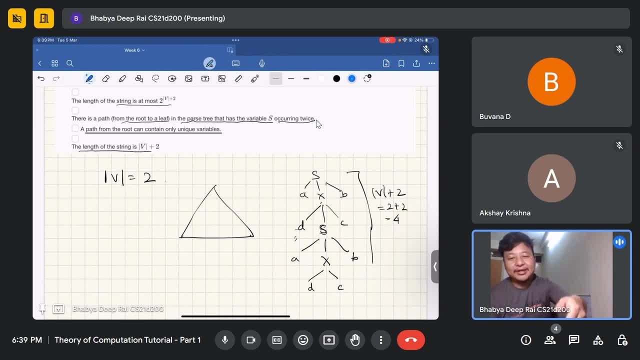 Only V many, So obviously there should be more than one in the path, more than one variable in the path, Right? So okay, I think I got charged a bit, So occurring twice. That is true, A path from root can only contain unique variables. 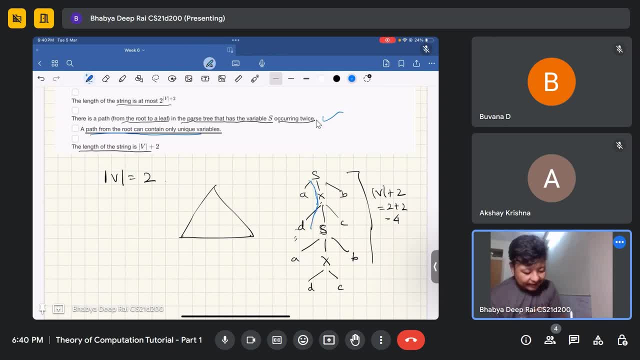 Is that true? No, I encountered X, then I encountered S, only It's not unique. Unique meaning encountered only once. Okay, This is clearly false. The length of the string is the size of V plus 2.. Is the length 4?? 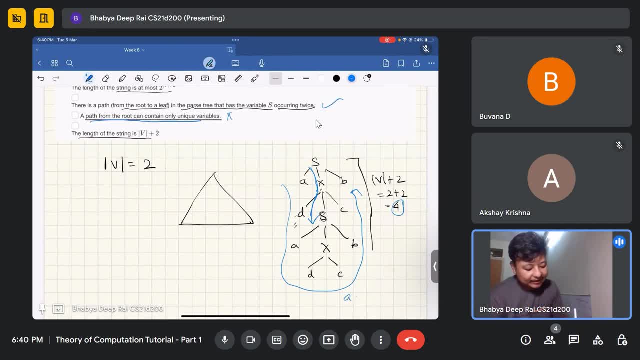 V plus 2 is 4.. No, No, Because our output is A, D, A, D, C, B, C, B, Right. What is the length of this? 1, 2,, 3,, 4,, 5,, 6,, 7,, 8.. 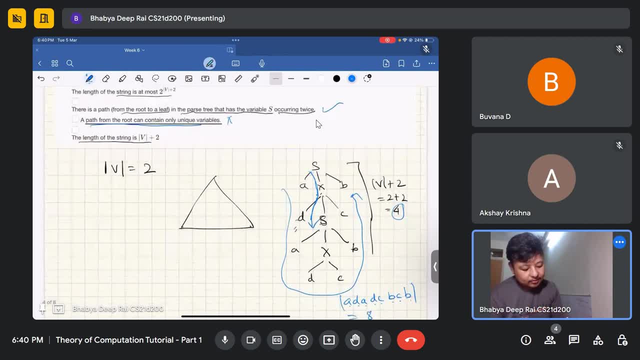 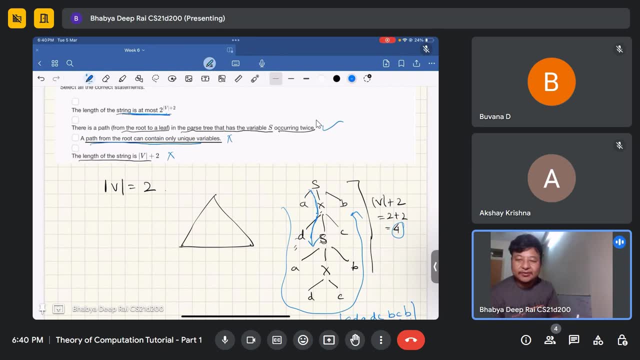 8 is the length. So this is not true. The length, our length, is 8.. The length of the string is at most 2 to the size of V plus 2.. Is that true? 2 to the size of V plus 2.. 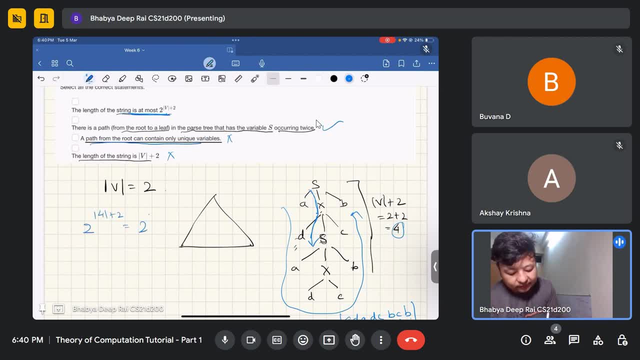 What is 2 to the V plus 2?, Which is 2 to the 4,, which is 16.. We have 8.. 8 is at most 16.. So the answer is yes. So A and B are true. 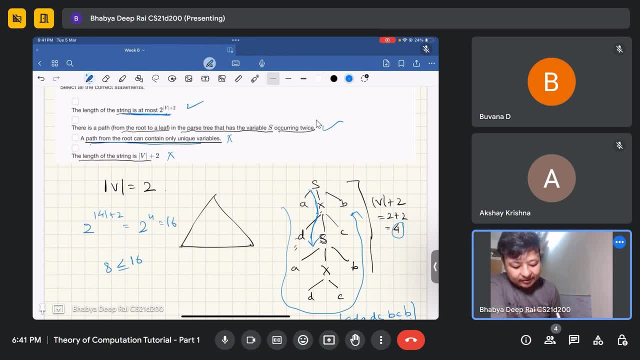 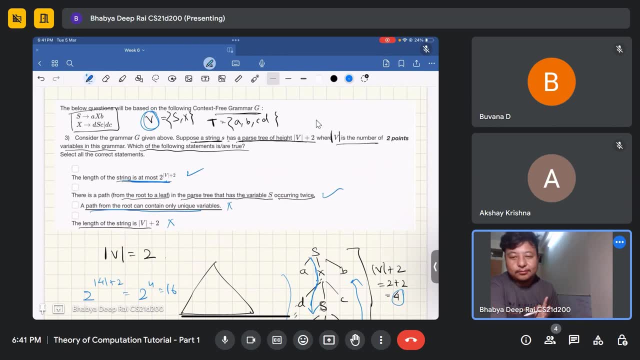 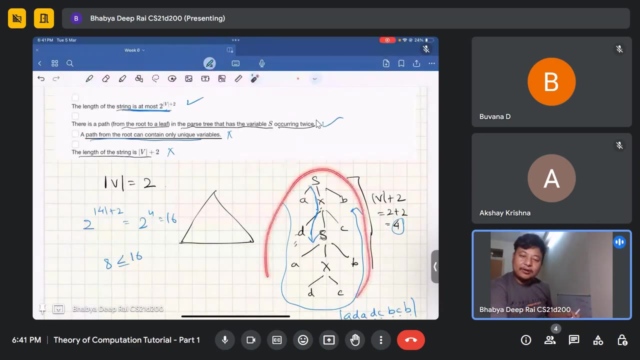 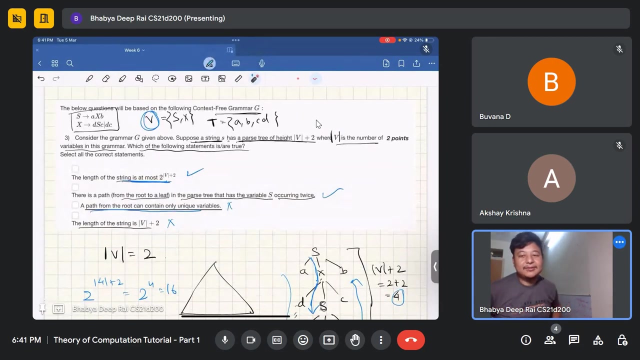 And the remaining two are false. But take note that there is nothing special about the number of variables, Variables being 2.. Okay, We can- actually I showed this, But we need not show this actually. We can just look at what is called the pigeonhole principle. 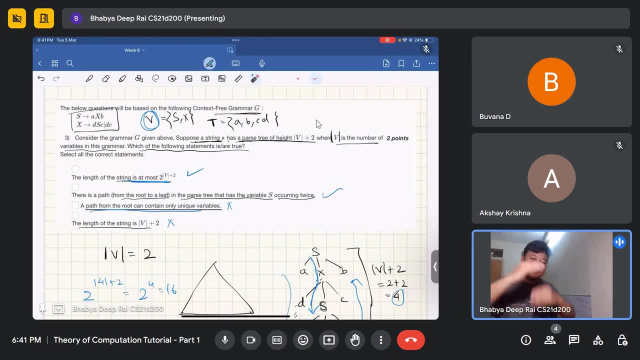 in discrete maths. Look at the fact that the height of the tree is very big. The height of the tree is very big, Much larger than V. So in any path there must be more than V. More than V, There must be more than 2 extra variables encountered in every house. 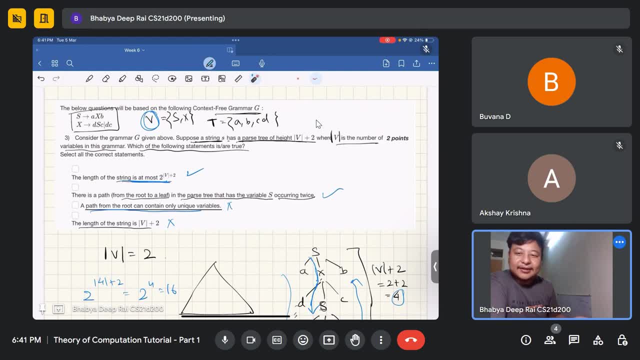 So that will give us most of the thing. And next is that you know at every level it is having at least two children. So the leaves of the tree is: If you take a binary tree, it is always true to the N. 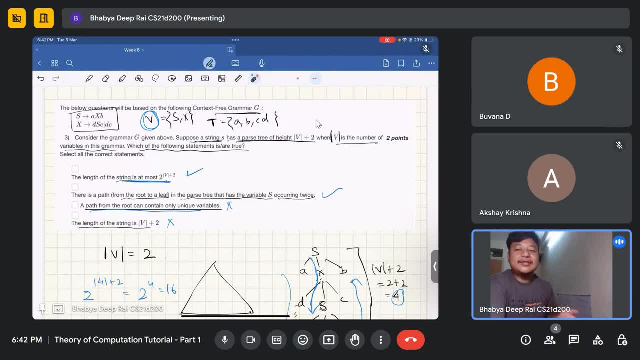 the number of children, where N is the height of the tree. So you can only say that the maximum number of children it has is true to the N. So therefore the length of the character generator is at most to the height of the tree. 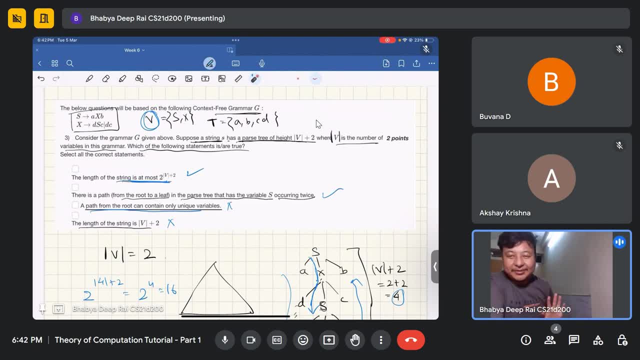 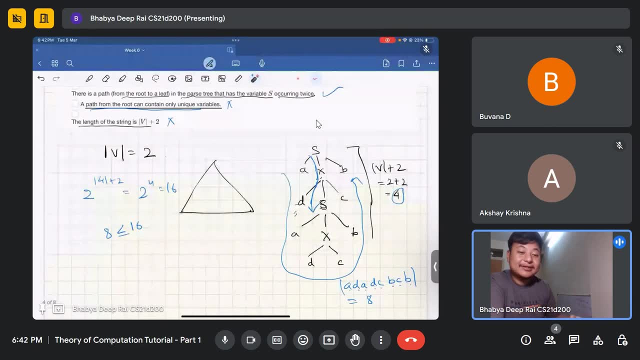 That is another way to argue, But here, since they are giving us an explicit example where there are two variables exactly, and this is how it behaves, we can analyze it further and say that, oh okay, this is the longest string that this particular string is the longest that this grammar can generate. 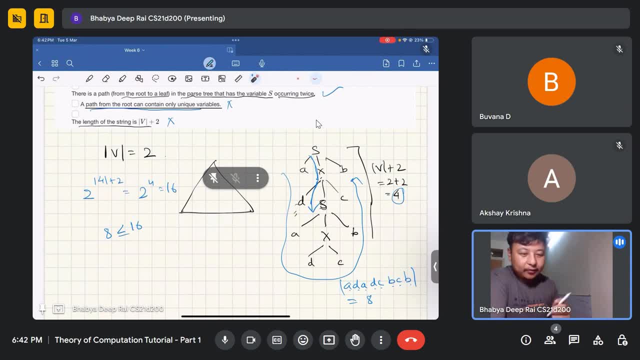 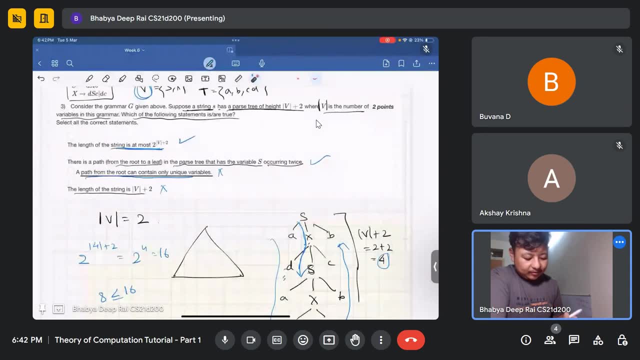 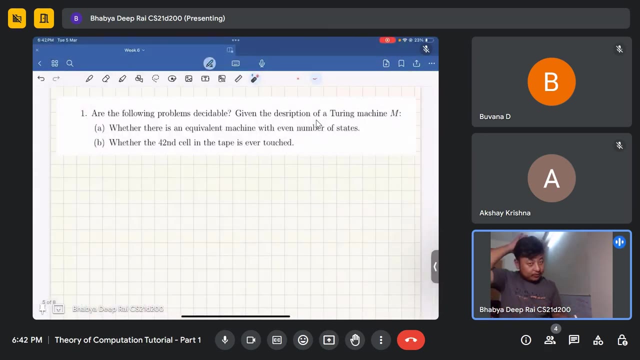 So that is another thing, That is another way to argue this. Okay, Good, So okay, I hope that was clear. It was not something too abstract, So I hope that was clear. So yeah, let's move on to this week's content now. 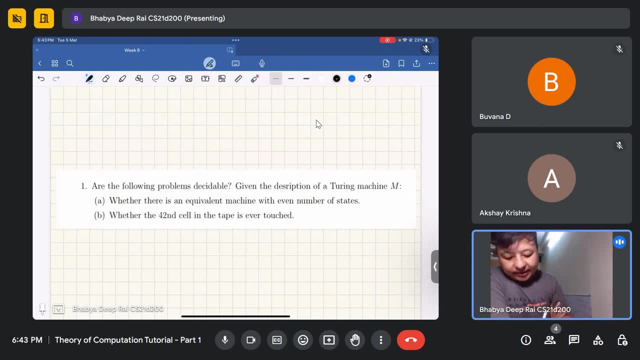 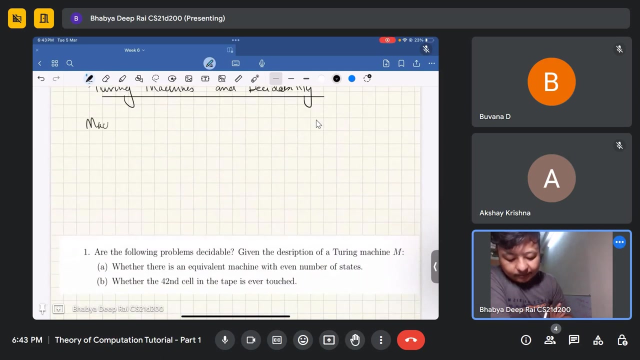 Okay, So this week's content is Turing machines and decidability. So we've seen machines already, right? What are the kind of machines we've seen? We've seen a DFA, finite automata or an NFA, And we've seen PDS and non-deterministic PDS. 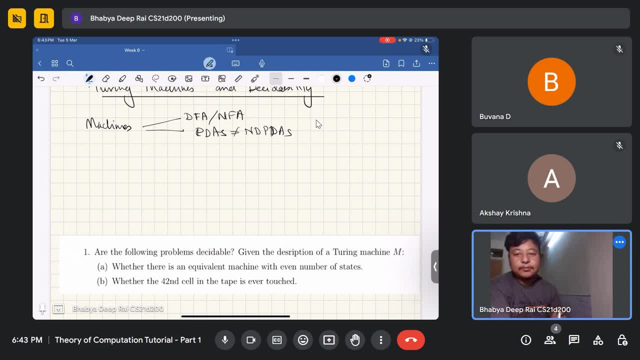 And we showed that these two are not equal in power, But these two are equal. DFA is an NFA, And there are some kind of models in between also, But this time we are only focusing on one, that is, Turing machines. Now, quick recap. 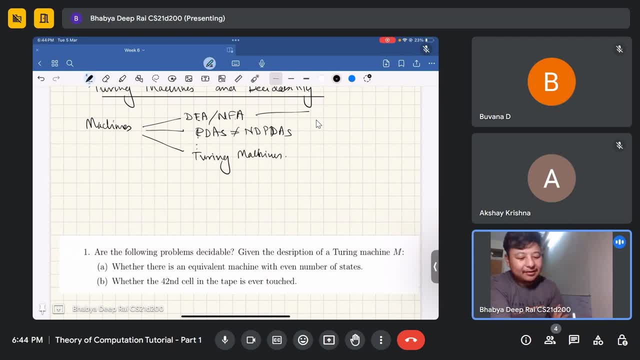 Here. what do you have? You don't have any memory or you have very little memory. constant memory, That is, you use states to remember. You can do simple tasks like modulo operations, right, And you can do regular expressions and so on, where you'd need just constant amount of memory. 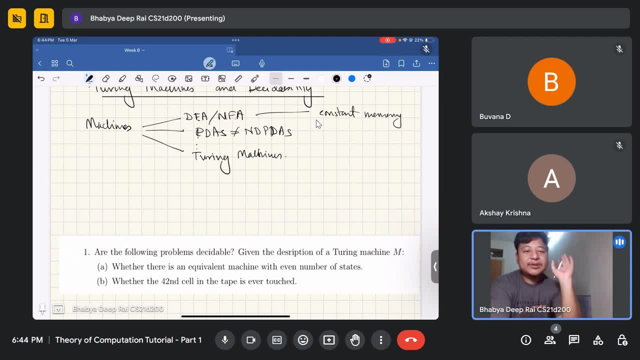 That means you just remember what state you are in, and that much memory is enough for you. What we want to do is we want to generalize the model, give it more memory, give it more memory and see what happens. So PDS and NPDS are one such generalization. 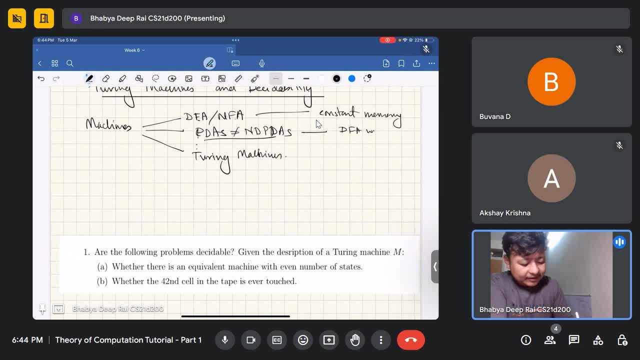 Here it can be seen as a DFA with a stack, And two weeks ago in the assignment we saw that what happens when you give a queue instead of a stack? what happens? and what happens if you allow only scanning once, and so on. 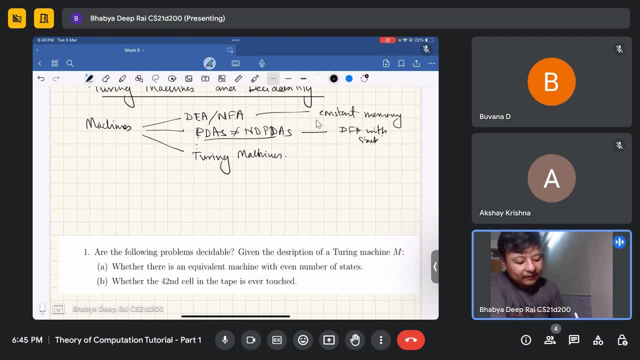 There are different questions you can ask, But this is: you know, you give it a memory but you don't give full access to the memory. It needs to be read in a certain order. That is what a stack is right. 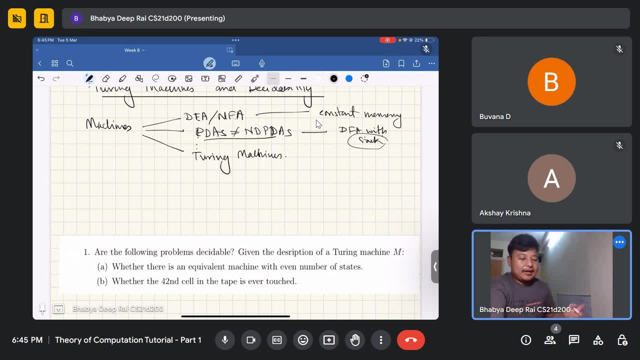 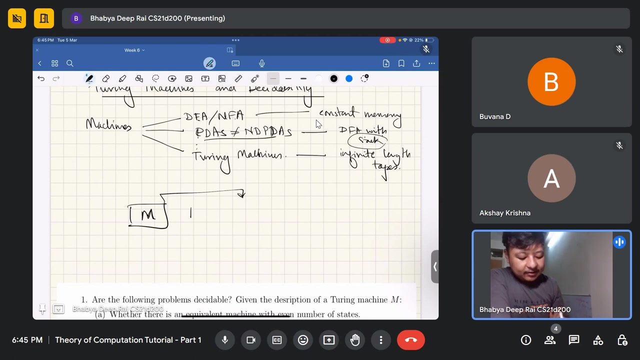 It needs to be read in a certain order. And finally, you have Turing machines, which are infinite length tapes. Okay, So Turing machines are- you can think of a machine M with a head. What is it called? A head is a pointer. 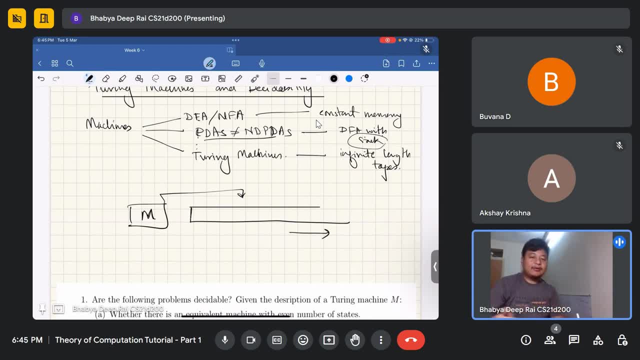 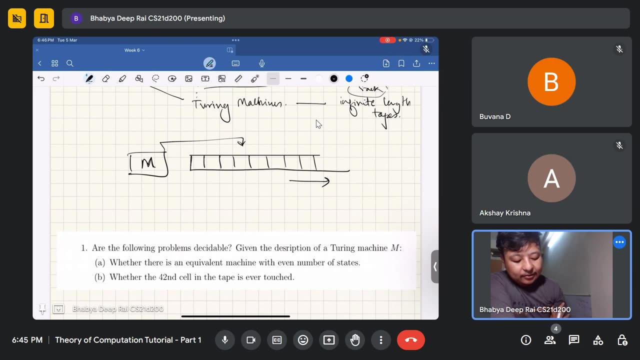 And there is an infinite tape. Okay, You can consider a one-way infinite tape, but it is equivalent to a two-way infinite tape. It can have infinite length on either sides And there are cells, okay, which are capable of storing your tape alphabet, which are taken from gamma. 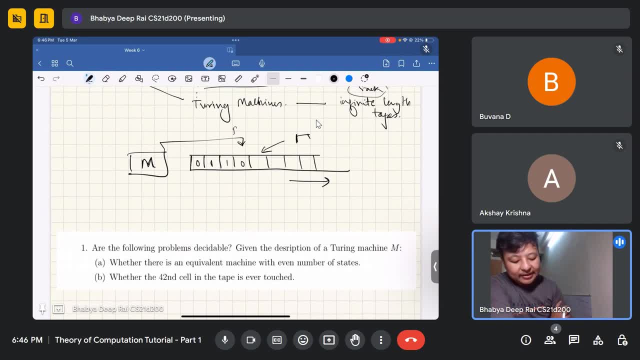 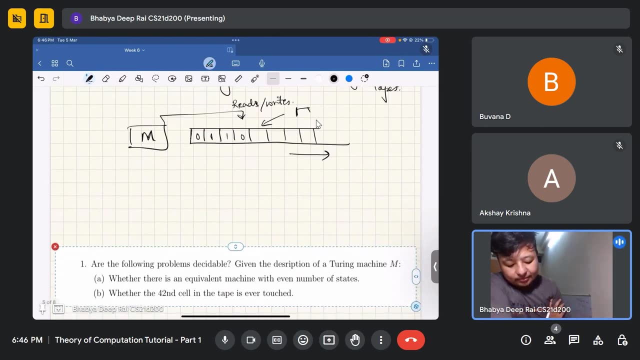 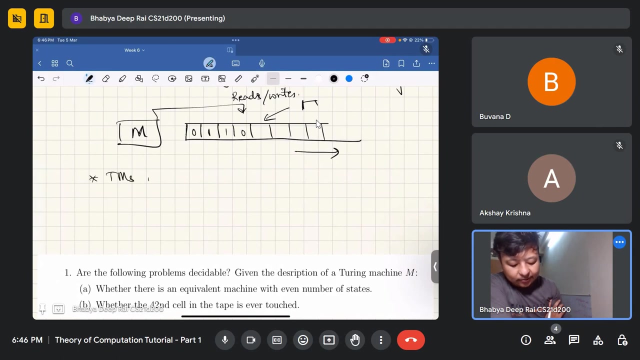 Okay, And you are allowed to perform reads and writes. And Turing machines may also be defined in different ways, But most of the ways are equivalent to each other. That is main important thing to know is that Turing machines with infinite- not infinite, sorry- multiple tapes. 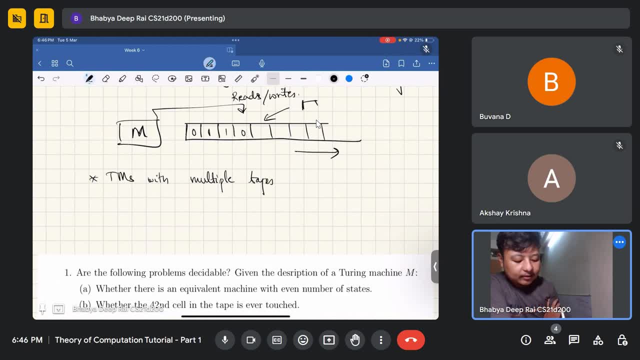 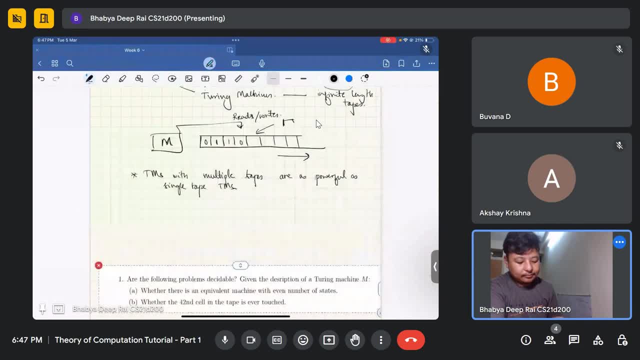 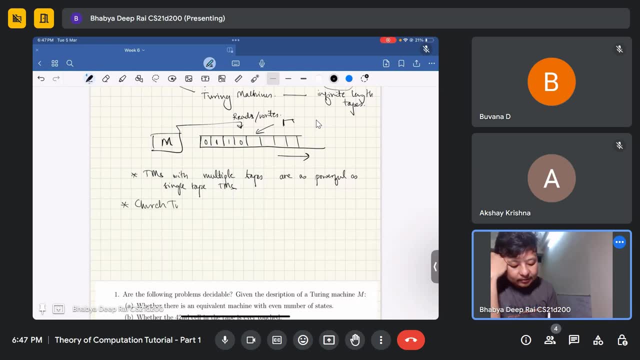 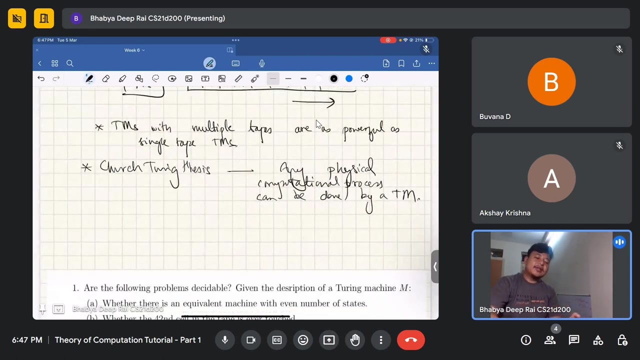 You have already seen that And and you saw the Church Turing thesis, Yes, Which says that you know any computational process, any physical computational process, can be done by a Turing machine. So what? what does it mean? It means that any computer that you can think of, okay, any phone or laptop or whatever Turing machine- is as powerful as that. 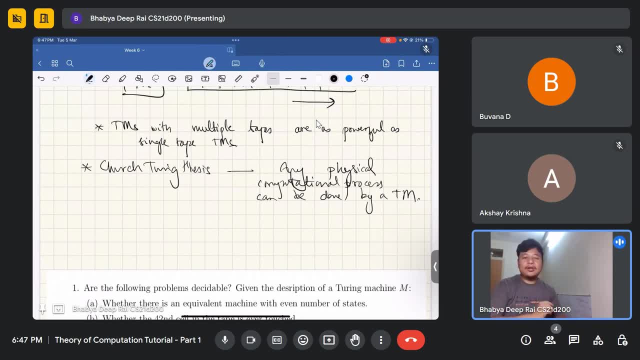 So Turing machine is not a weak model. In fact, Church Turing thesis says that you cannot actually build a machine which is more powerful than a Turing machine. By power we don't mean speed. By power we mean the ability to solve problems. 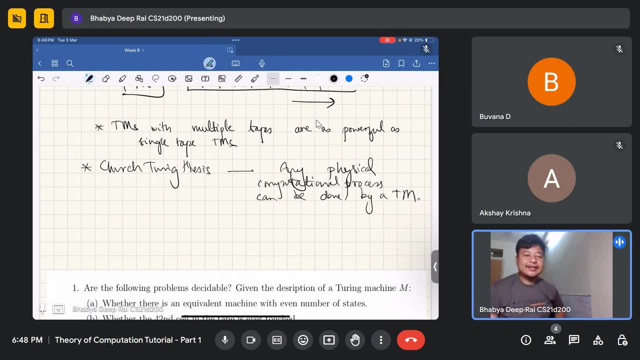 In other words the ability to decide languages, recognize and decide languages. So, but you know this, this is a vague thing to say, Okay, So you cannot have a very formalized proof for this. Hence it is not called a Turing machine theorem. sorry, Church Turing theorem, or Church Turing lemma, or whatever. 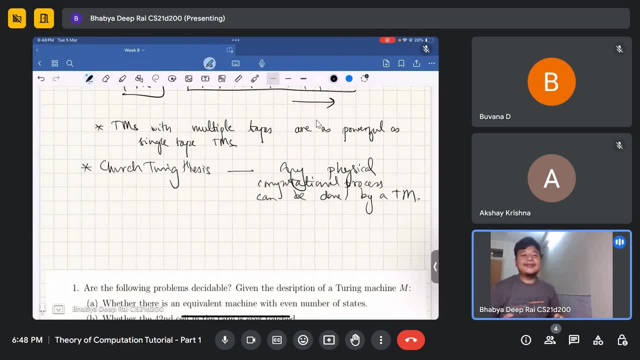 It is called a Church Turing thesis, because this is something that you know cannot be proved, But it is believed to be true, Okay, And therefore it also means that any algorithm you can write- okay, any algorithm that you can write, you can do it by a Turing machine. 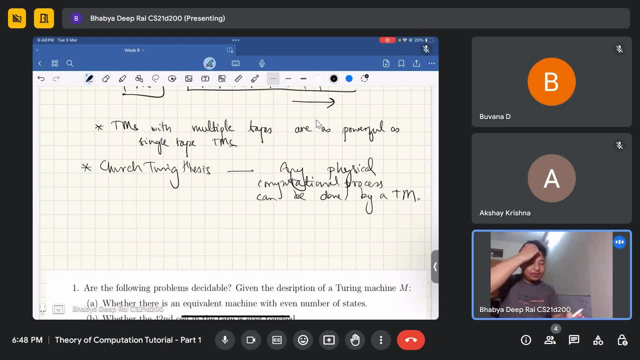 So when you think of Turing machines, I just want to make this small remark that when you think of Turing machines, please don't restrict to the view of you know the tapes and you know making marks here and there and so on. 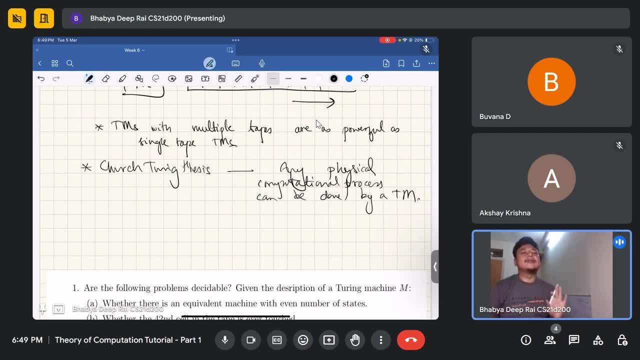 you can. you can abstract it out to algorithms. okay, so you can write description of turing machines as if you are writing descriptions of algorithms and since they are equivalent by the church turing thesis, it is always fine to write them as algorithms, because in bfs we were thinking: 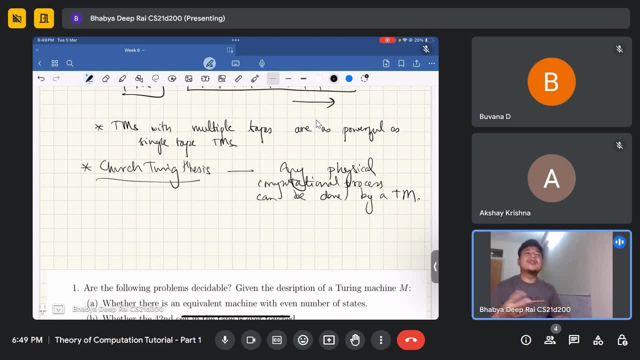 of states. no, moving from one state to another, turing machine, you don't need really need to think of it in terms of, you know, moving to one state, another, there is a, there is. people also teach in this way, right where? oh okay, move from left to right and then right, when you see an a. 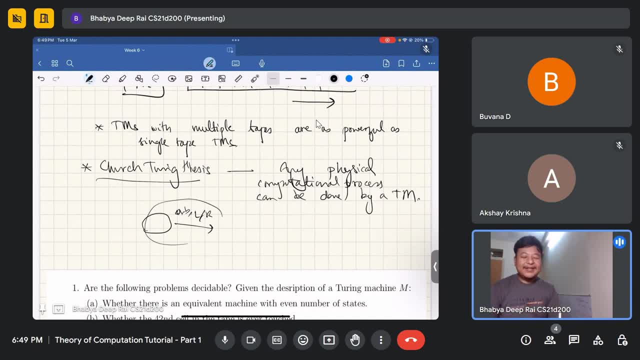 right or b and then move from left right. so this is a very restricted view about it. when you try to solve harder and harder problems, this this becomes very complicated and low level. so it's it's like coding in binary or assembly. so think, think of just. 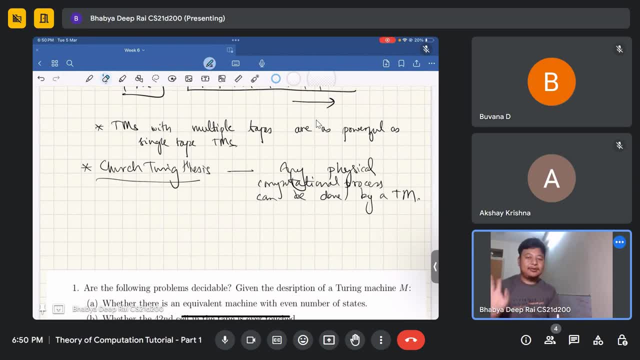 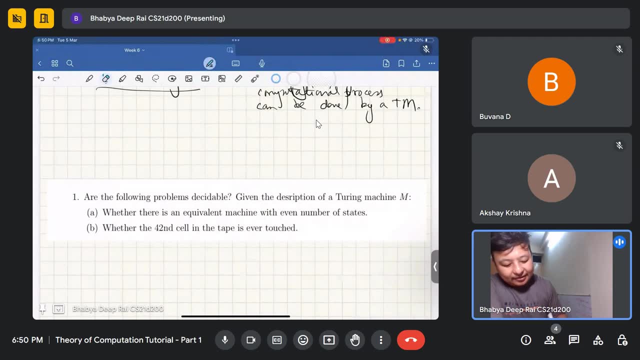 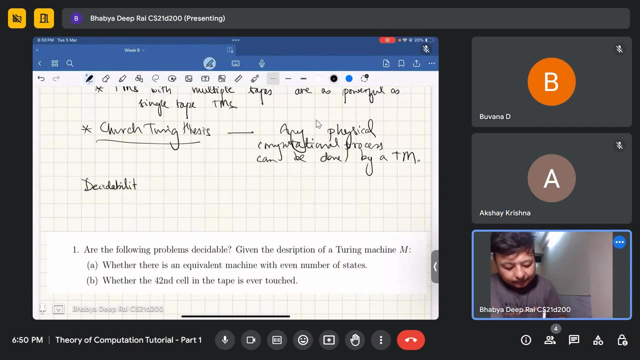 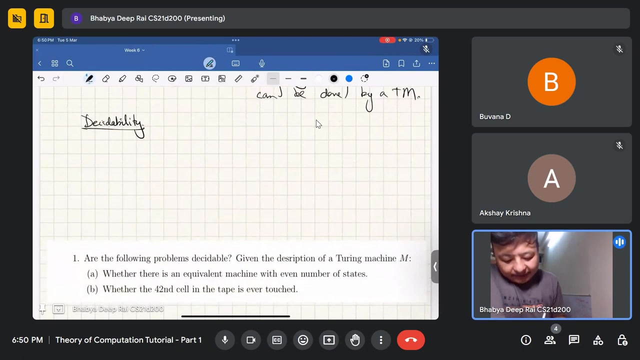 uh, your regular algorithm, pseudocode or c programming or something like that? okay, and that will always help. okay. now, finally, uh, the main topic, okay, is about decidability, decidability, okay. so what is decidability? a language, l, is decidable if there is a turing machine that accepts it. 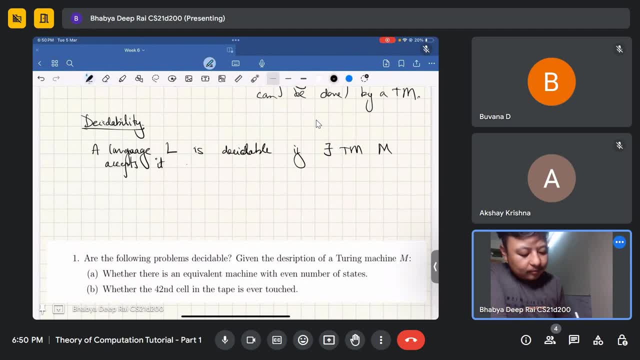 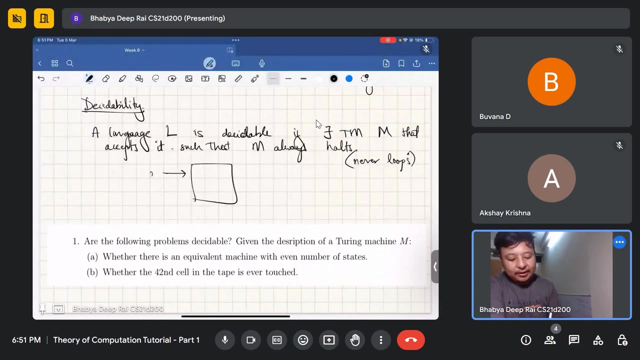 the turing machine, let me call it m- such that m always faults, in other words, it's never loops, loops meaning infinite. okay, you don't keep needing to wait for an answer, okay? so, uh, any input on any input. let's say, i give a machine m, it will never happen that it keeps. 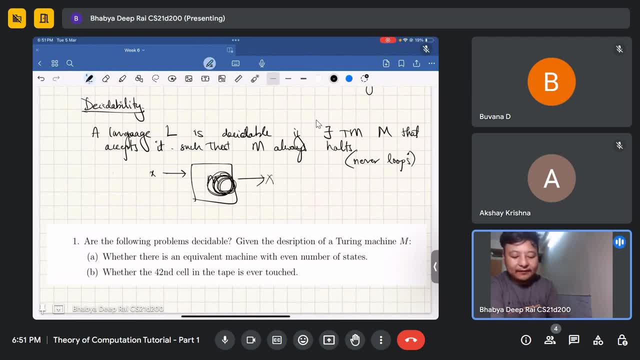 looping, infinite looping, and it will never give me an answer. it will never happen. it will always give me an output, given an input. okay, then, if, uh, if such a turing machine exists for the language which accepts all the strings in the language, then it is uh, then the language is called decidable. furthermore, such a turing machine, 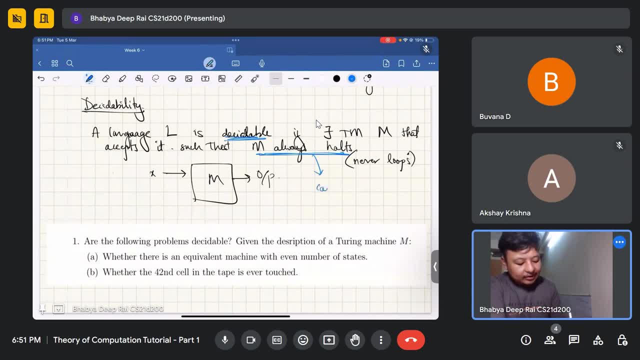 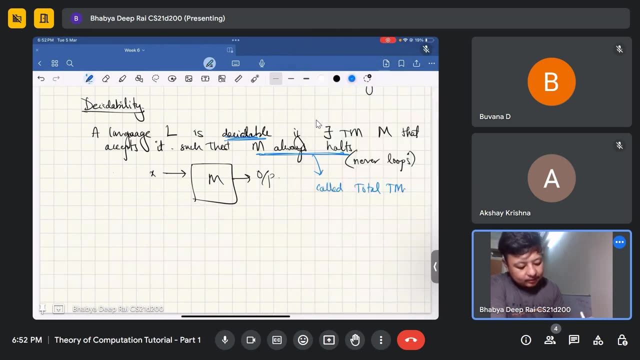 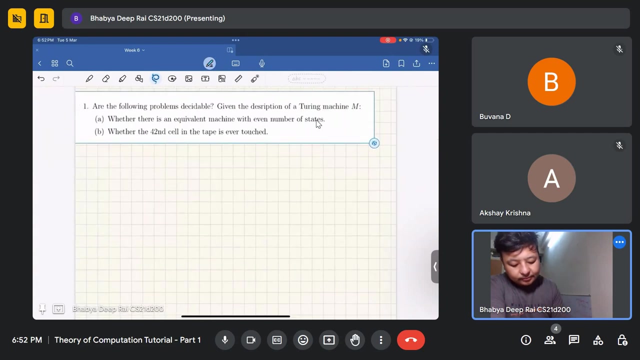 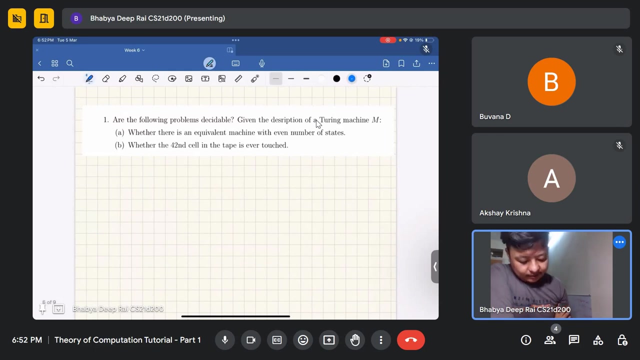 that m always holds. such a turing machine is what is called a total turing machine. okay me to duplicate. i think copy is better cut. yeah, now we solve some problems. yeah, okay, great. so the question says: are the following problems decidable, given the description of a? 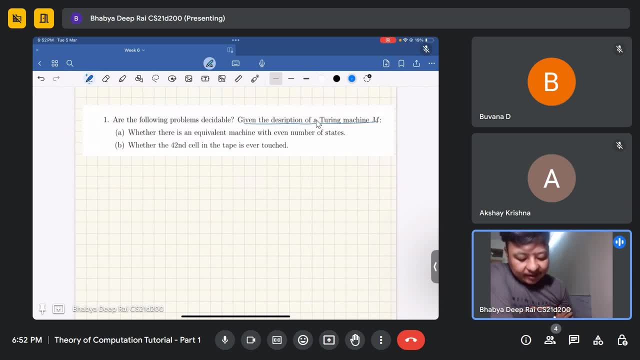 turing machine m. can you test whether there is an equivalent machine with an even number of states? this is the question: whether uh, this, this, this uh problem is decidable or not. in other words, you can interpret it as a language. what will the language be? it will be the set of descriptions of all m. remember that this is a string. 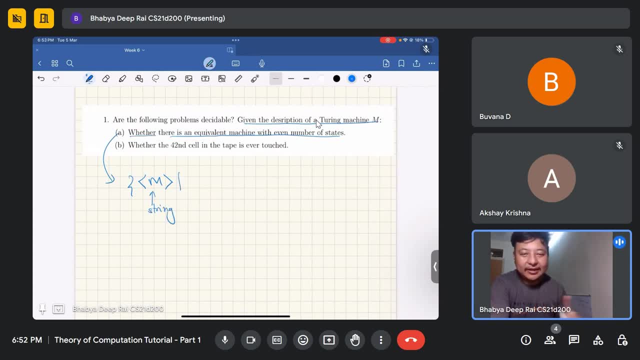 and in the lectures you've seen that any turing machine can be written as a binary string. right, so now, uh, okay, a string m. uh, that represents the description of m. okay, such that, um, there exists a turing machine, m, with even number of states. so any guesses? uh, would it be decidable or undecidable? 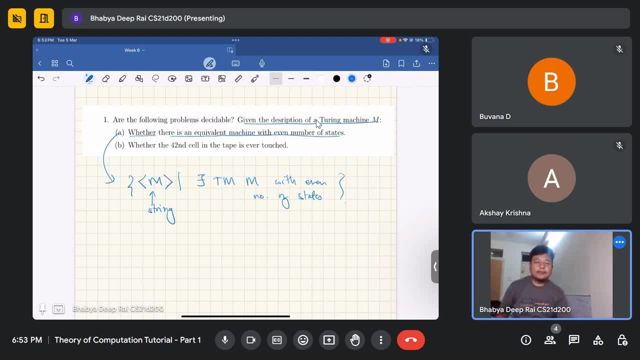 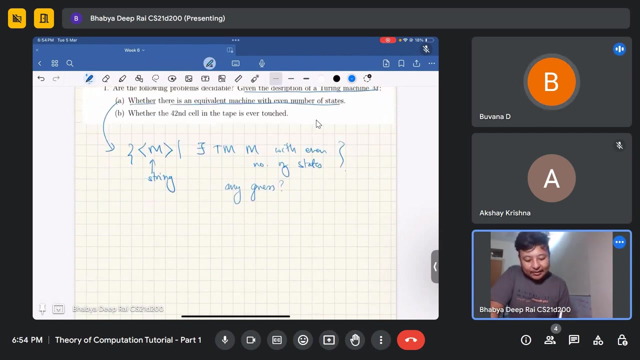 so any guesses? uh, would it be decidable or undecidable? um, decidable, it is redecidable. okay, good, why any? any reason you think turing machine, except the given a turing machine game. turing machine, Turing machine accepts even string. but here I will slightly explain this further. 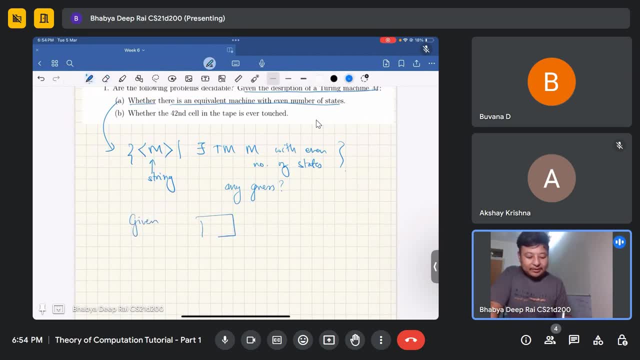 What we need to decide is given is a Turing machine M and description of M. it is a string and it is a description of M. you want to tell if there is a Turing machine N. you want to tell whether there is N, such that it has even number of states. 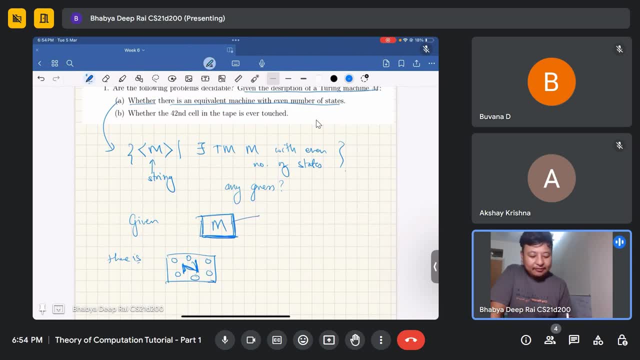 What you meant to say was: you look at the description and check whether there are even number of states. You look at the description and because what is contained in this description? it will be, like you know, sigma delta, sorry, gamma Q. final state, start state. 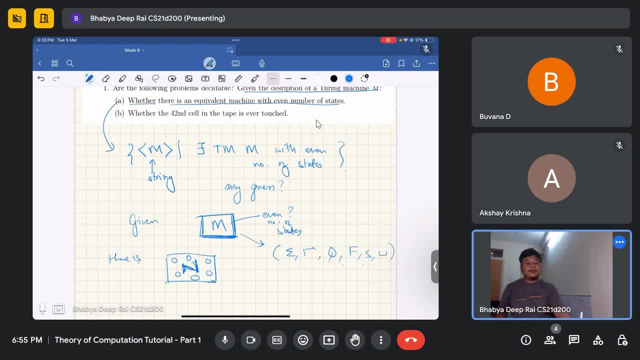 So you look at this and just look at Q, okay, and count the number of states and tell whether it is even or not. So is that what you meant, Bhuvana, or is there something else? Yes, sir, that is a Turing machine already. 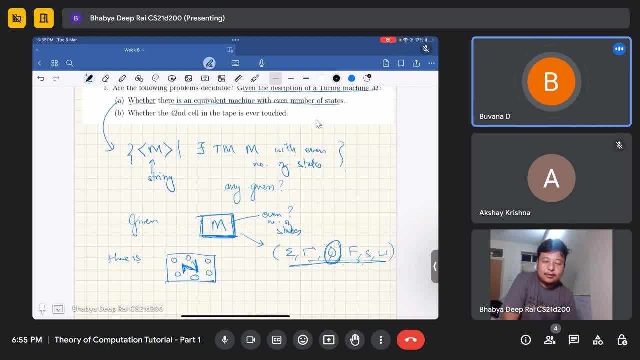 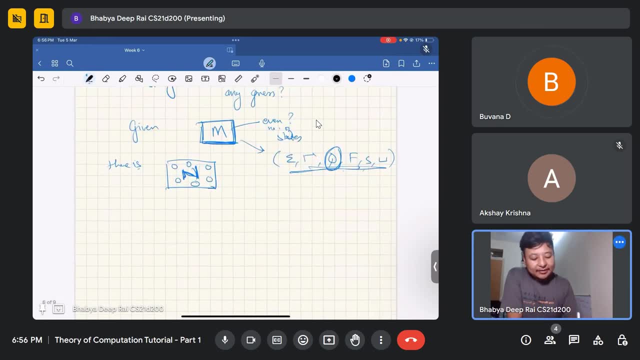 Yeah. So you said that there will be equal admission, Right, right. So if that, yeah, yeah, that is one thing. So if you look at the description and you observe that there are even number of states, then you can definitely say, yes, there is a Turing machine which accepts the language. 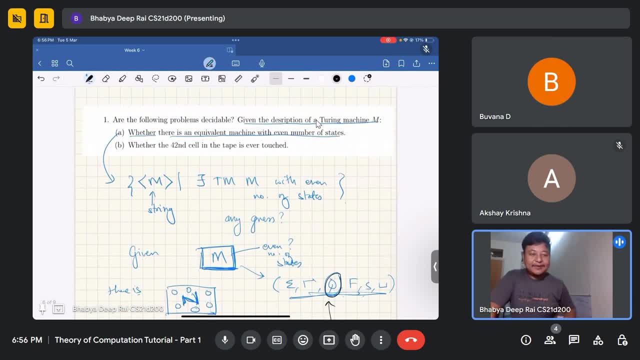 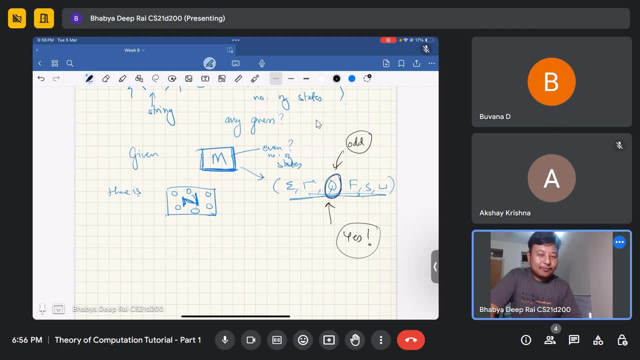 okay, which accepts the same language, which has even number of states. That is true. but the question is now: what if this turned out to be odd? Yeah, that is true. Okay, But how do we say for sure that we can never build a Turing machine accepting the same? 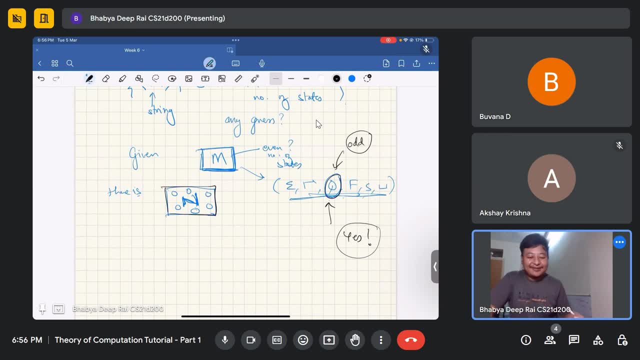 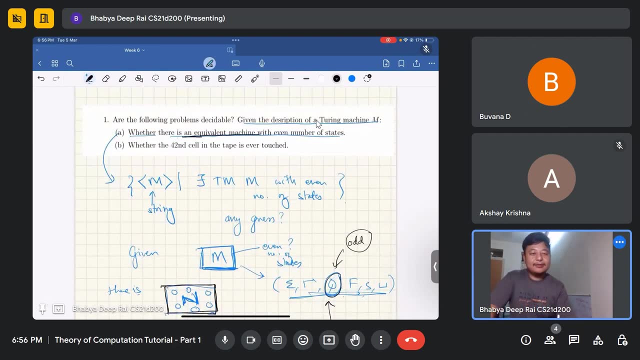 language with even number states, How can we say that we can never build another Turing machine? So if you look at the question whether there is an equivalent machine, or in other words, another machine which accepts the same language, with even number states, getting at what I 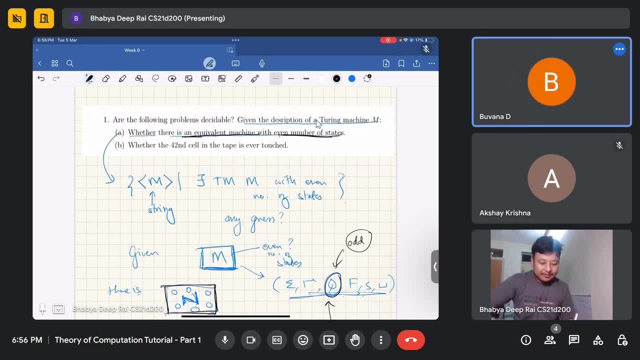 am saying? What I am saying is the problem is given a Turing machine, we want to check if there is an equivalent machine, which means another machine, another Turing machine that accepts the same language. Remember that every language need not have a unique Turing machine. 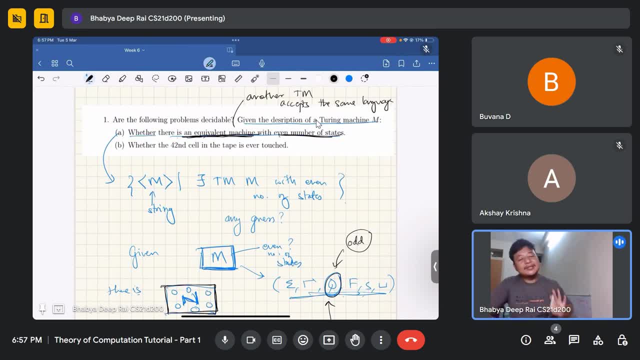 For a single language. there may be multiple Turing machines that compute the same language. Now I look at the input, which is M given to us, Okay, And I count Q. I count the number of states And the number of states turned out to be even. then I say okay, yes, there is a Turing. 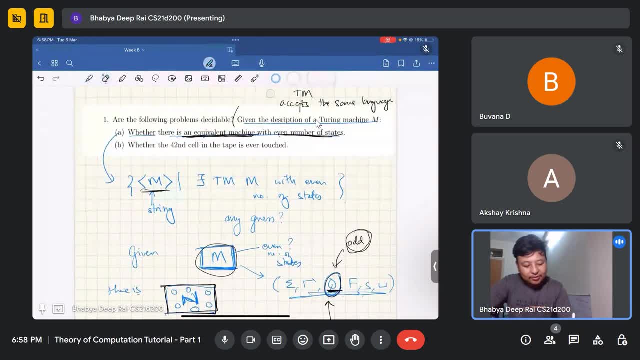 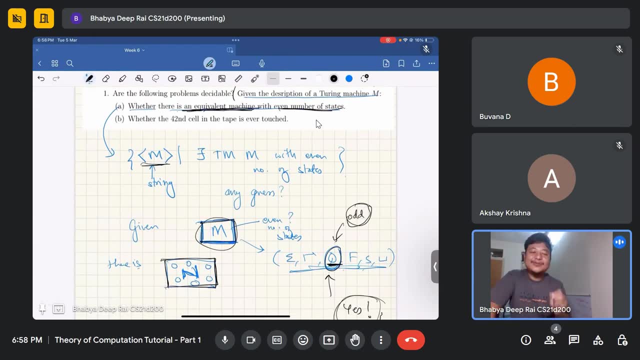 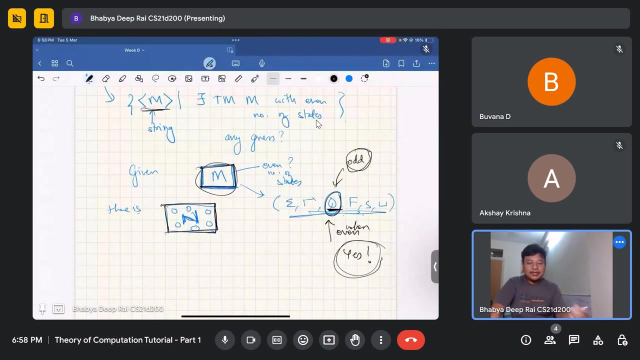 machine, not another, some Turing machine that accepts the same. Then we will say: oh yes, this machine itself is a machine which will accept the same language and has an even number of states. Then we will say that, yes, When it is even, when this is even. 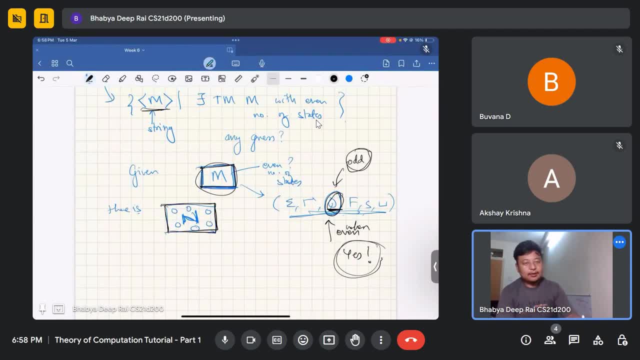 But what if this is odd? Now, like you said, if this is odd, then we will say no, But how can we guarantee that there will? M has odd number of states. that is fine, But how can we guarantee that there does not exist any other machine which will compute? 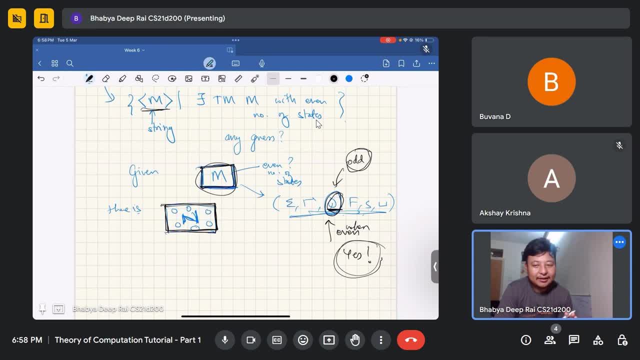 the same language. You get it now what I am trying to say. Yes, Yes, sir, Already they have told that commonly. they have told that Turing machine accept that the first statement. Hmm, Then, if there is an acceptor, definitely it may be of odd number or even number. 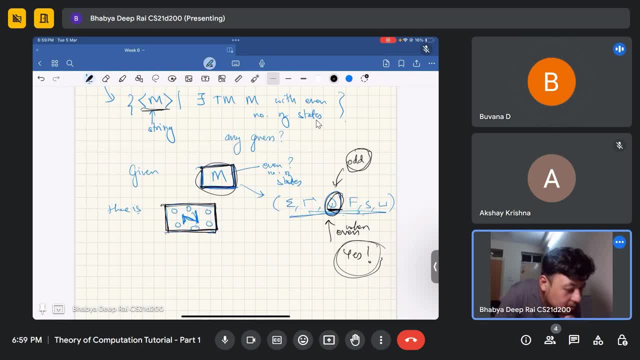 Yeah, Sorry, I cannot hear you properly. can you say again In the statement? Question statement: Say it again. Can you show me the statement? Yes, Yes, sir, I am, though the this this is. the channel is noisy so I cannot hear you from it, may. 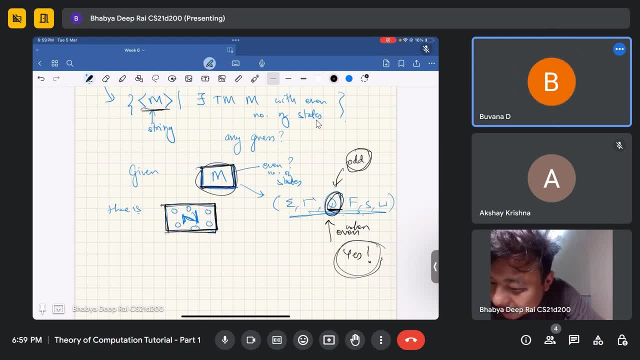 have odd numbers or even numbers, but it is accepted. yeah, it is a decidable also, right, right, it may not number. it may be, may consist of odd number of states. are it may consist of even number of sheet, right? okay, it may have an odd number of states and they could also exist. a tooling machine which has an 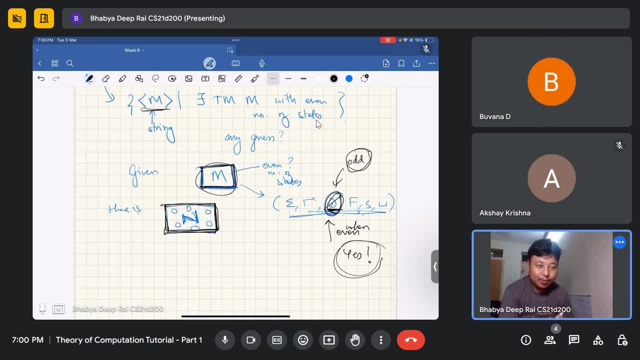 even number of states which accepts the same language. but how do I do that? how do I make another machine that accepts the same language, but with even number of states? now I'll tell you. what you do is take the same machine. okay. Where to add a dummy to a machine? 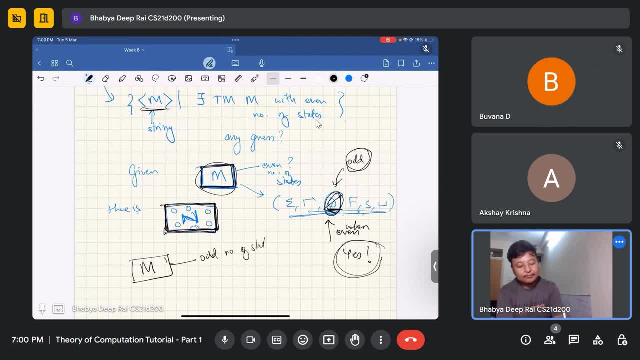 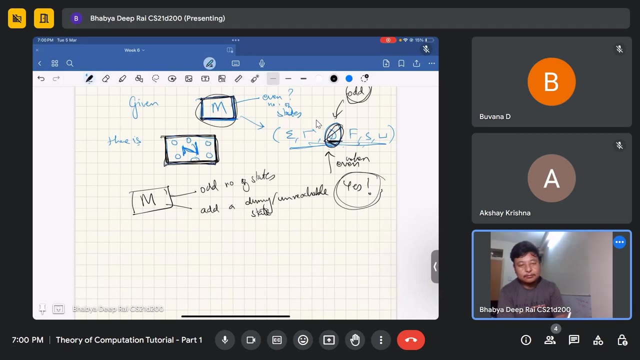 number of states. what I'll do is simply add a dummy state- ok, dummy. what do I mean by dummy unreachableör u getethe Doom, or dummy Unreachable state, to this machine method. my resulting machine will have how many states? odd number of states. it already had odd number. 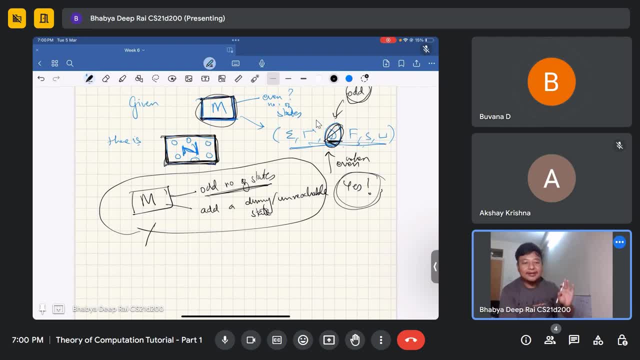 of states, I am adding one more state which can never be reached: Even number. it will give even number, Exactly even number. and does it affect the language computed? Yes, Does the language computed change If we include the dummy? it gets halted. sir. 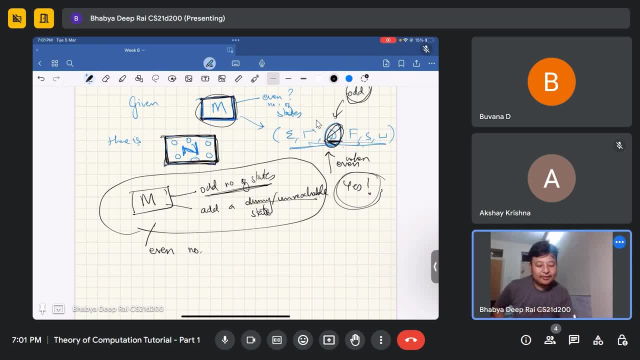 No, no, no, halting. m was already halting or it doesn't matter whether m was halting or not. I am just saying l accepts a set of strings: a, b, c, b, c, d and whatever. 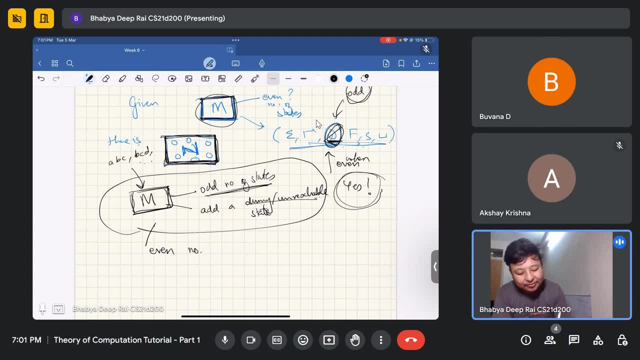 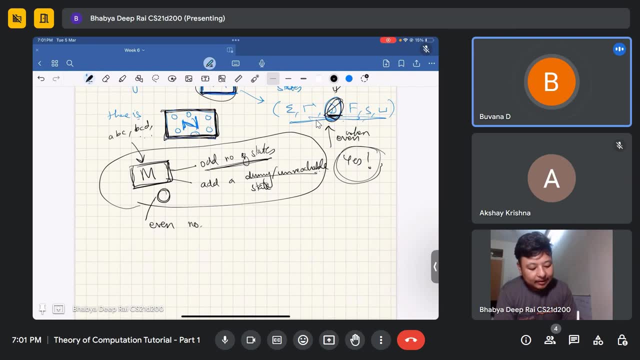 That is what m accepts. If I add one more state to it, Which is not, which it is not, I will explain using a DFA. okay, Let's look at the DFA accepting a star, b star, okay. So what does the DFA look like? here is the empty state, and if I see a's okay, then I 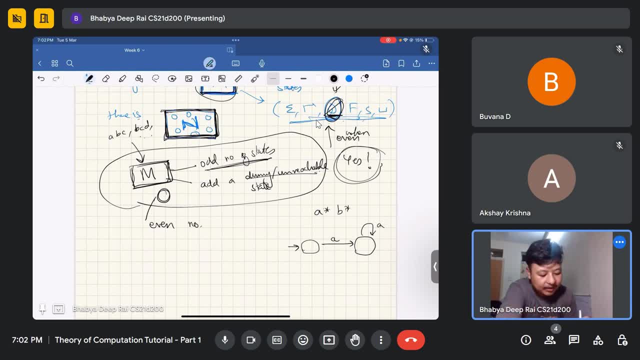 will go to a loop, okay. and or let's not even do a star, b star, let's just do a star. This is a DFA accepting a star, right. What happens here? It sees an a and it keeps seeing an a. it will still accept right. and if it sees a. 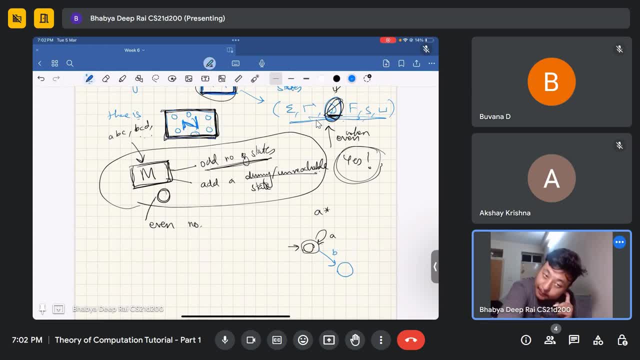 b anytime, then it will go to a dead state. Correct, This is the language. okay, What is the language? A star? Now, what I am saying is: let me add another state to it. okay, I will call the state 1,, I will call the state 2,, I will call the state 3, okay, and this. 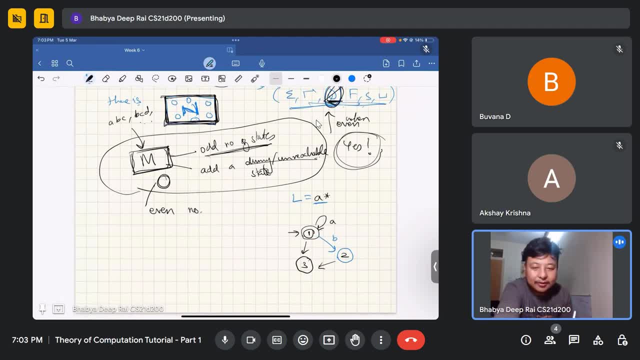 state does not have any arrows coming to it, Okay. Okay, If it has no arrows, it is what are called unreachable. or it is also what is called a useless state, because no string can actually encounter this state. okay, Now tell me, is this DFA accepting any more strings than it used to, or any fewer strings? 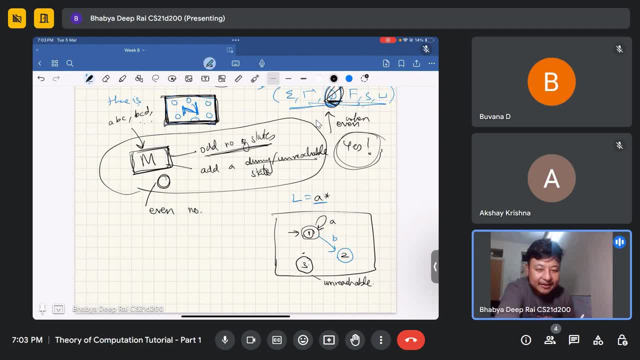 than it used to? Is the language of this DFA changing When I added the state No sir, No right. Yes, Because this state is unreachable, it is useless, it is not doing anything. Yes, sir, Similarly to this Turing machine M, which have odd number state, I added this: unreachable. 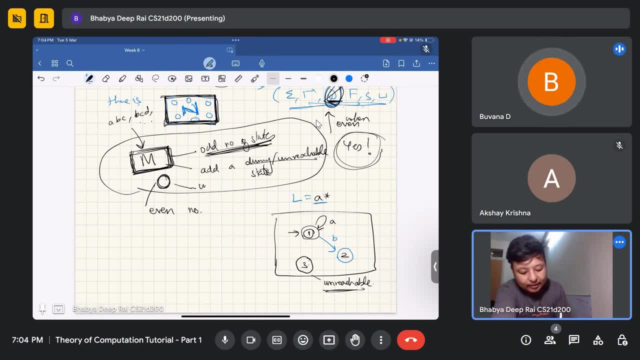 state: Okay, Yes, sir, And no string will ever reach this, Because there is no. There is no definition in the transition function that says: go to this particular state. let me call it D: go to this particular state. It is never saying that, so there is no string that reaches it. 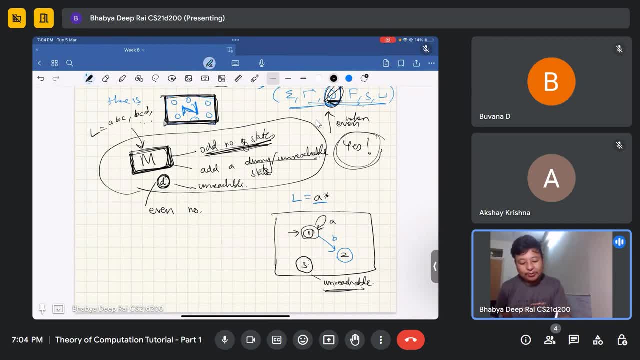 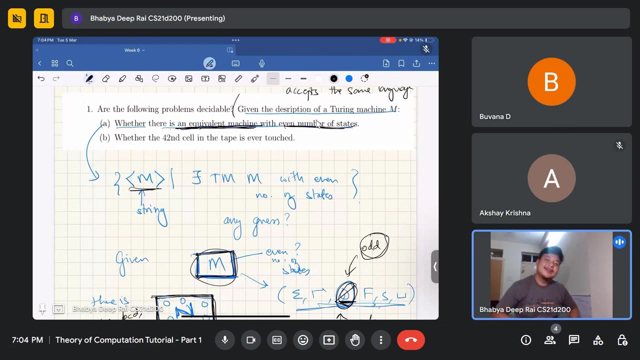 So if M was accepting a language, L, what will this bigger machine accept? This bigger machine with this unreachable state? It will still accept L, right, Yes, sir, Right. So now the question of whether, given a Turing machine, can I build another Turing machine that has even number of states, will always be true. 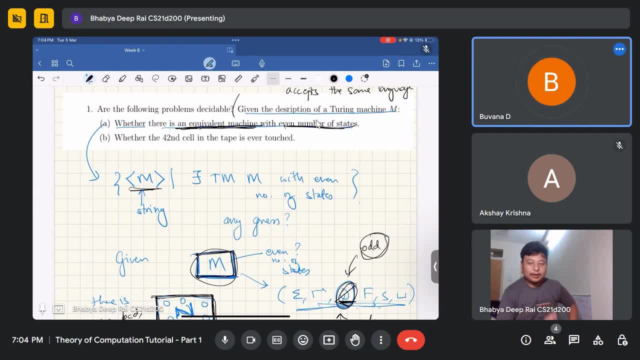 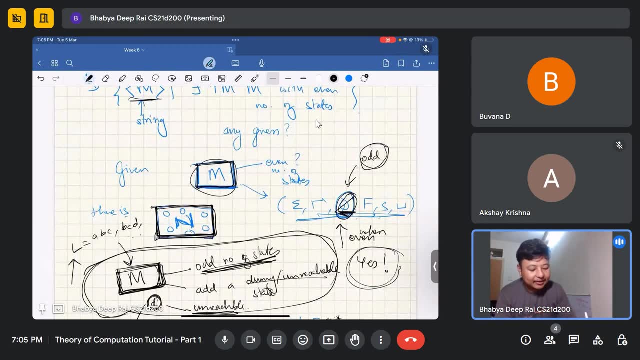 Even number of states will always be true. Why again, Because if it already had an even number of states, then, like you said, I will just say yes, Because itself it is an example of a Turing machine with an even number of states. 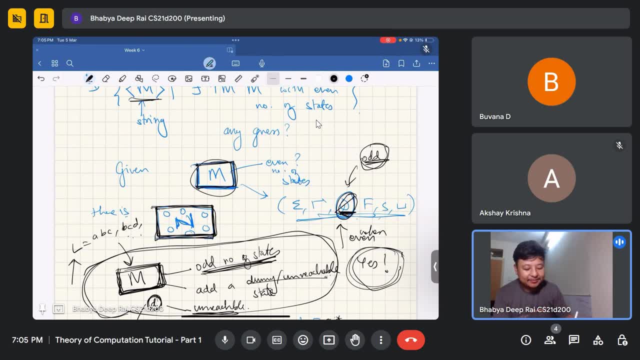 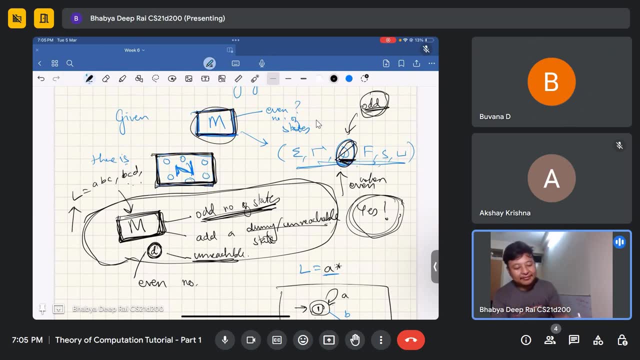 Okay, Right, But if it was odd, what I will simply do is I will add this dummy state and make it even number of states: Yes, sir. And then the language computed is same and therefore it is always true. The answer is always true for this problem. 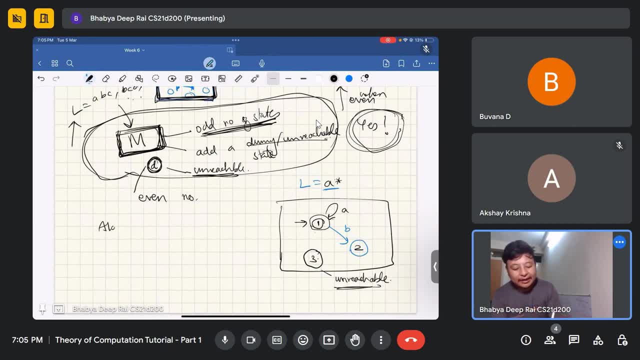 Sorry, answer is always yes for this problem. So what is the algorithm? The algorithm or the Turing machine? what is the Turing machine that does this? It takes us, When input a machine, M. it will just output yes and halt. 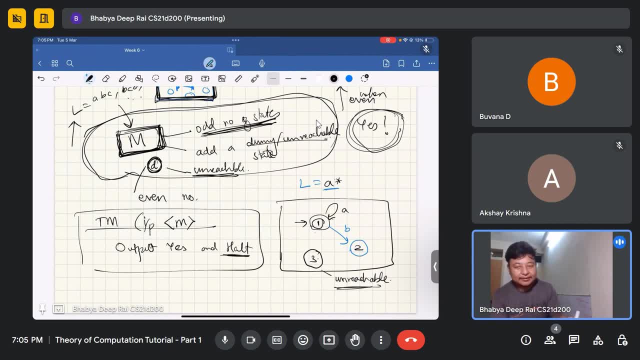 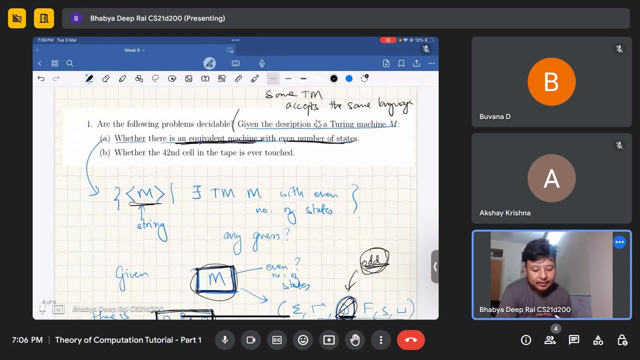 And since this Turing machine halts always, this is a total Turing machine And the problem. so the problem is decidable. Okay, The key idea is that it is always possible to come up with even number of states. Okay, Okay. 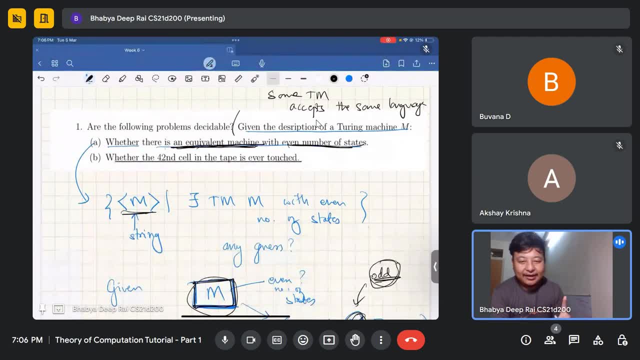 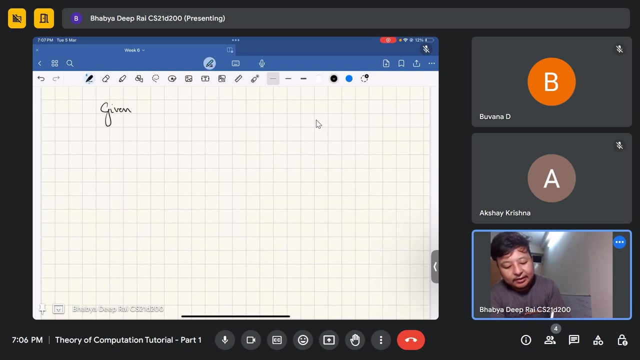 So this is Slightly of a higher difficulty. Okay, And Here is the question: Is it decidable, given a description of a Turing machine, whether the 40 second cell in the tip is ever touched? Okay, So, given M. 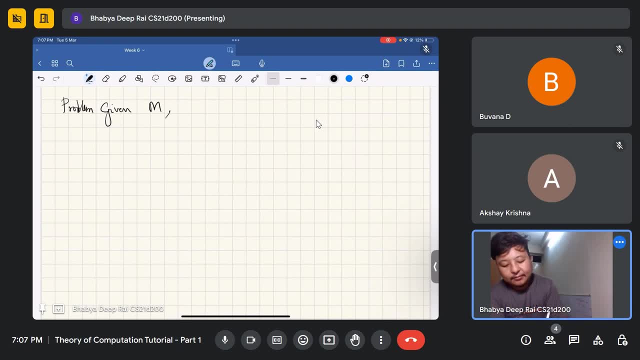 Okay, The problem is as follows. Okay, Problem is as follows: Input is the description of the machine, M. The output is yes. if there is the input such that M touches the 40 second cell, Good Then. Okay, It should be easy. 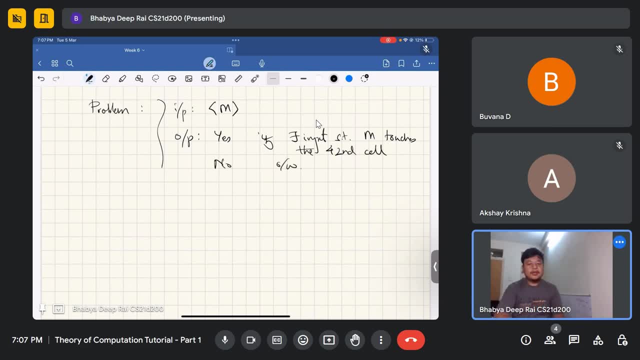 All right, otherwise. so this appears to be undecidable. okay, why I'll tell you this appears to be undecidable. why I'll tell you? because here this is what we need to do. okay, so this is the input. 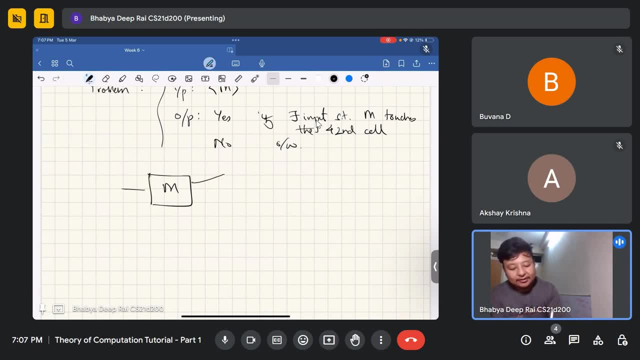 m. so if I run over the, let's say, over 0, I run. okay, I run the machine over 0 and it moves here and there. the head pointer moves here and there until it finally touches 42 and I say yes. 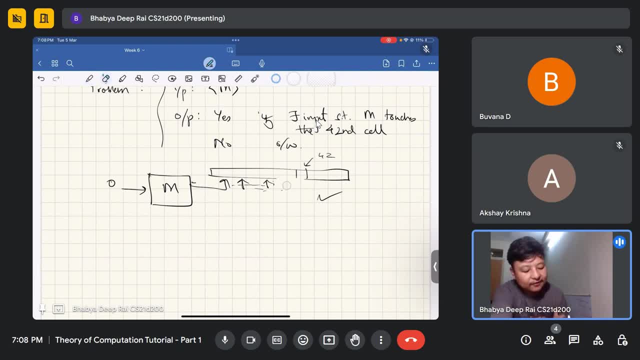 But what if it did not touch 42?? What if it never touches 42,? 0, given 0,, I'll give a 1. now, yeah, it could loop, right, it could always loop. and what if it loops inside here only getting it? what if the tip? what if the head? 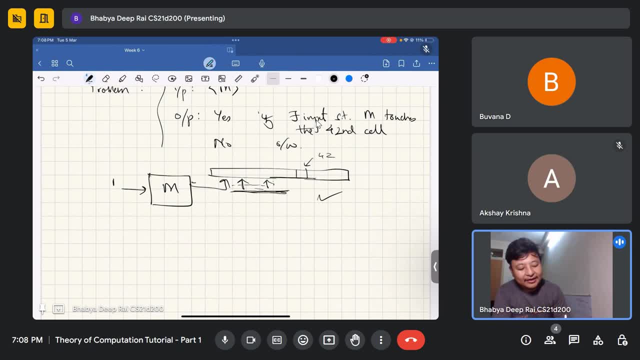 pointer. It keeps moving left right, left right, left right, but it never touches the 42nd cell. Yes, sir, Then I'll just keep waiting for the machine to reach the 42nd cell. no, and that will never. 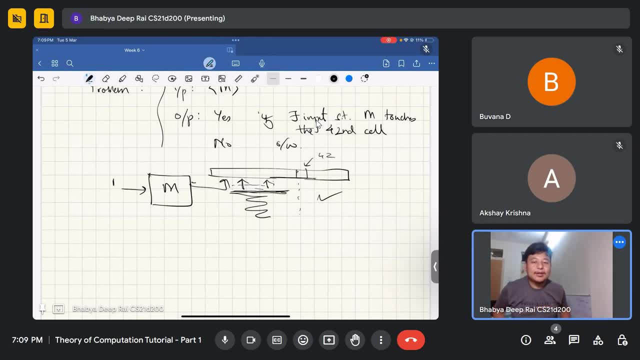 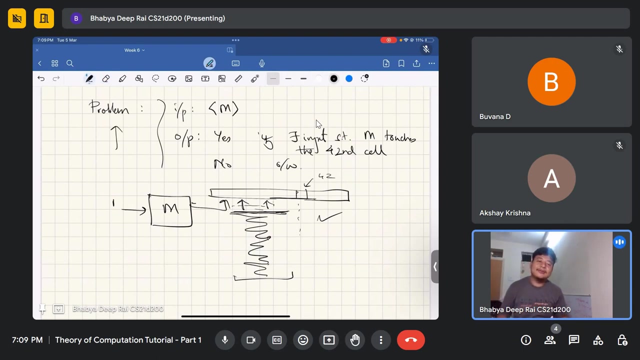 happen that that will never happen, because the machine is configured in such a way that it will always loop here. Okay, and therefore any. I would say that, oh, okay, any Turing machine that needs to solve this problem cannot be total, it cannot halt, because if the Turing machine takes the input and simulates it, then we'll keep waiting until the 42nd cell is touched. but what if it loops before going into the 42nd cell? 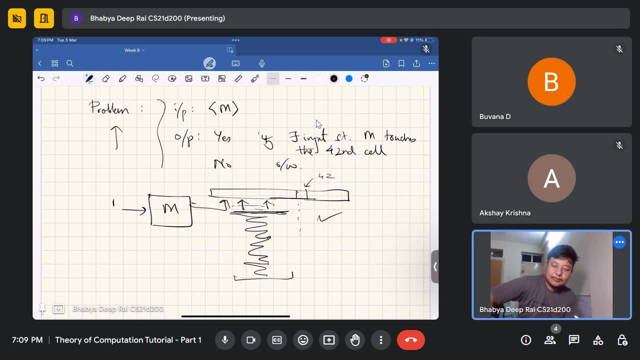 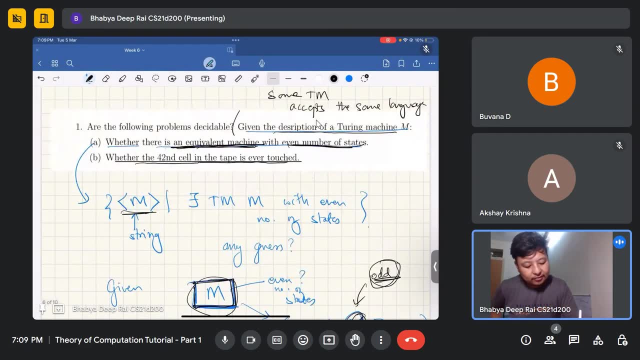 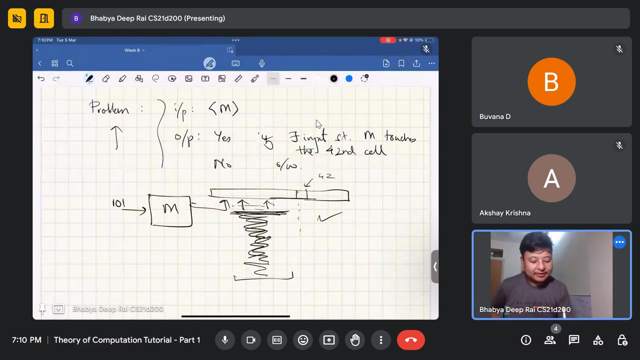 Okay, okay on on. sorry, Okay, Ever touched on input. let's call it 101, sorry, this is a full question on input 101, so I input 101,. what if, on input 101, it keeps going back and forth within the first 42 cells and it never touches 42,? my Turing machine will keep waiting for it to touch 42, is the? is the problem clear? 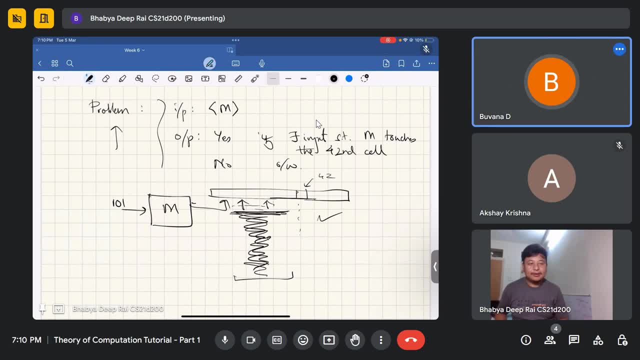 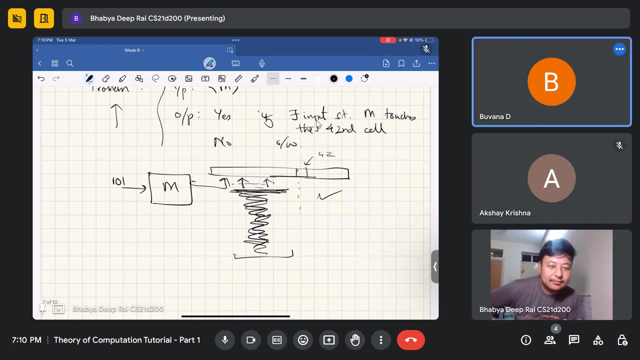 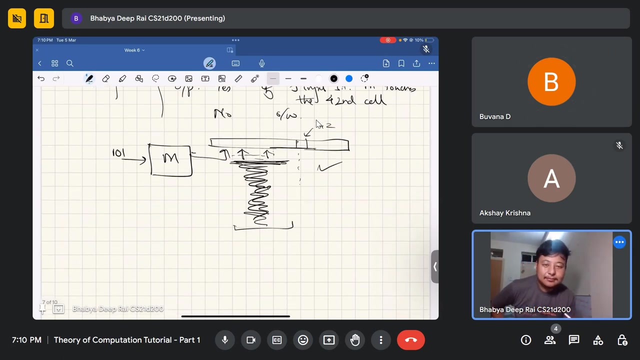 Yes, sir, it is undecidable. sir, Yeah, Wait. well, it appears undecidable. that is what I want to say. it appears undecidable but surprisingly it is decidable. surprisingly okay, okay, why, yeah, yeah, yes, sir, okay, okay, yeah, um. 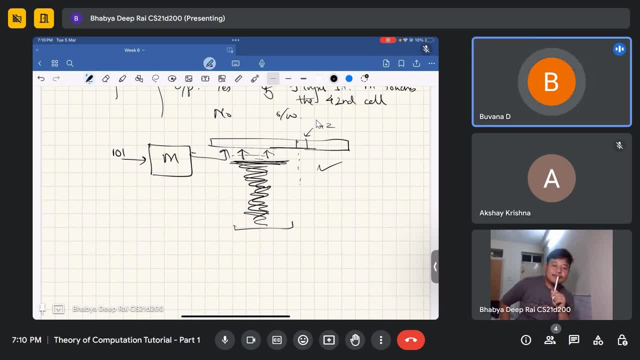 that is. it is a loop, sir, it it goes on looping. Hmm, Is is, yeah, the. the question is: can we detect the loop? Can we detect that it will go in an infinite loop? Uh, no, sir. 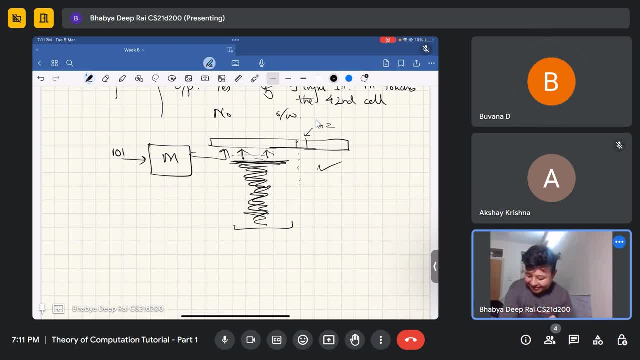 No, why? Why? It makes sense to say no, that is true, Because, um, if, if you could detect the infinite loop, then I mean um, it, it. it would be like um, the, the, the problem, the halting problem itself would become decidable, but the, the main thing is um, this is the answer here. okay, the 42nd cell. uh, Akshay, are you with us? are, are you with me? 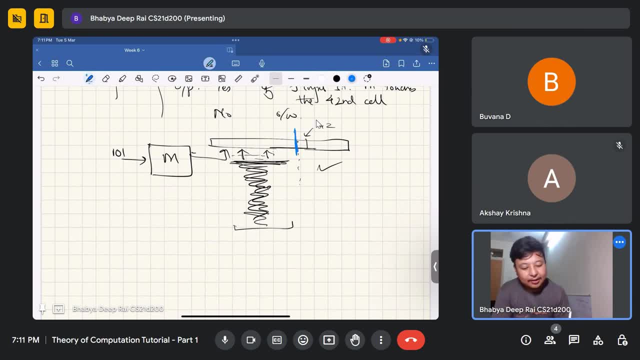 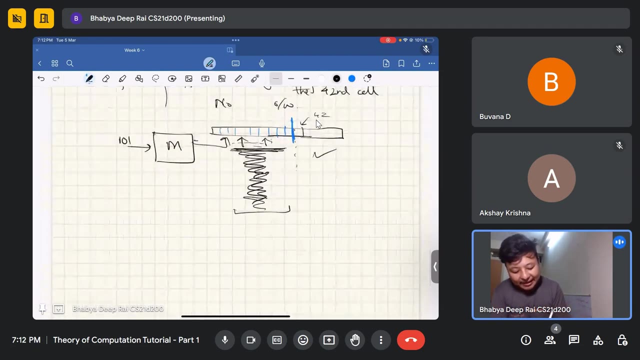 Yes, sir, Yes, sir, Yes, okay, Okay, The. the fact that I'm bounding the length of the tape to 42 is the is the key here. okay, is the key here. So, what is the bad case? okay, what is the good case? first, 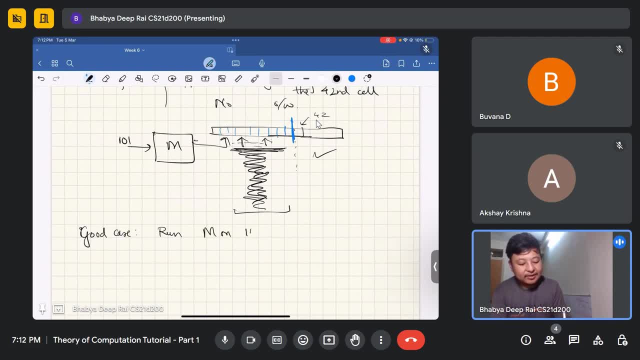 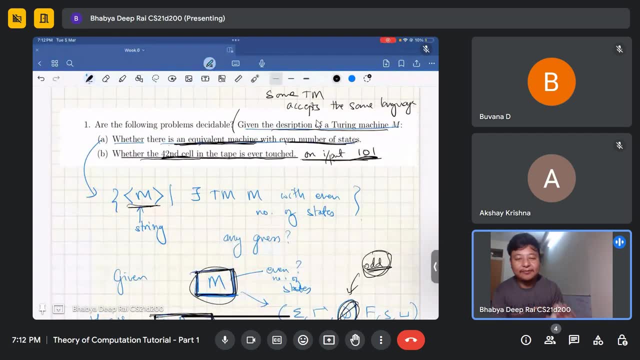 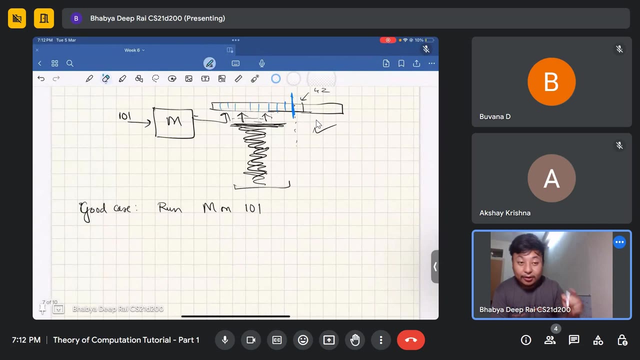 Run M on 101, okay, that is what the question is. okay, whether it will ever touch the 42nd cell on input 101. That is what we need to test. okay, Run M on 101, okay, this is this is what our total, supposed total tuning machine will do and, um, uh, M halts, okay, after touching cell 42, then output: yes. 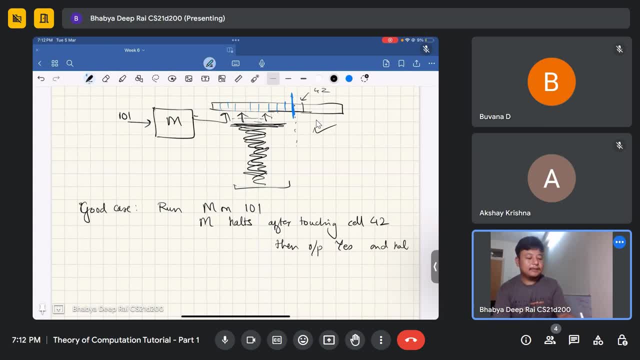 And halt. Yes, Yes, Yes, Yes, Yes, Yes, Yes, okay, good, this is a good case for us. okay, it keeps going. we simulate and it touches- though, it touches- the 42 cell. I'll output: yes, okay, it touches the 42. 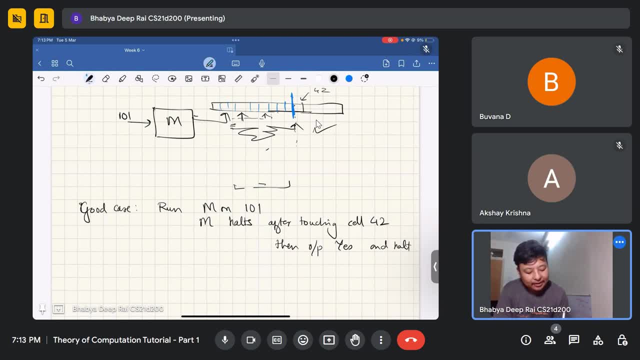 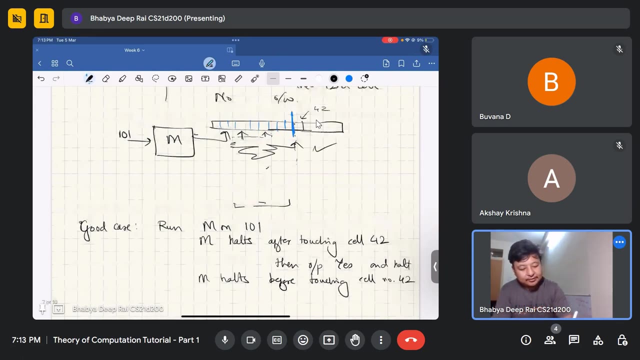 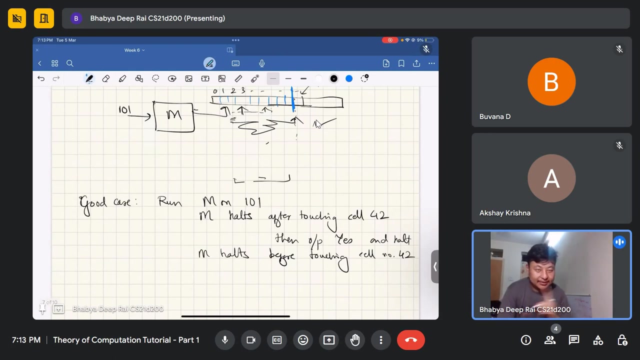 cell. good. but another thing is M halts before touching cell number 42. okay, so I'll call this 0, 1, 2, 3 and so on till 42 before touching 42. so since it M never touches 42 cell number 42, so it will output. then we need to output no it. 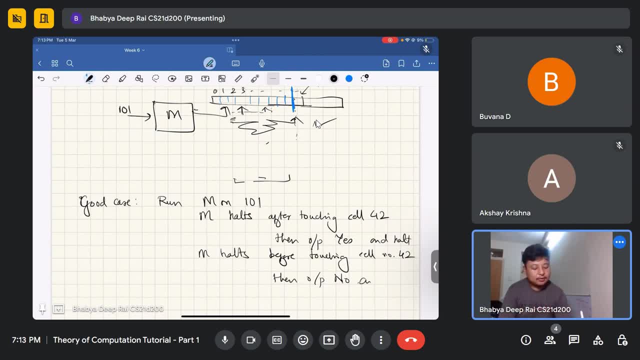 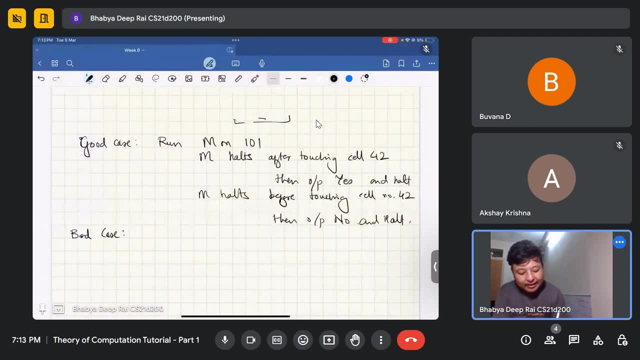 never touches 42. now, what is the bad case? what is the case that we are not handling M loops, okay, okay, M loops. yeah, M loops also while looping. okay, while looping, M touches 42, while looping, M touches 42. this is also good for us because you 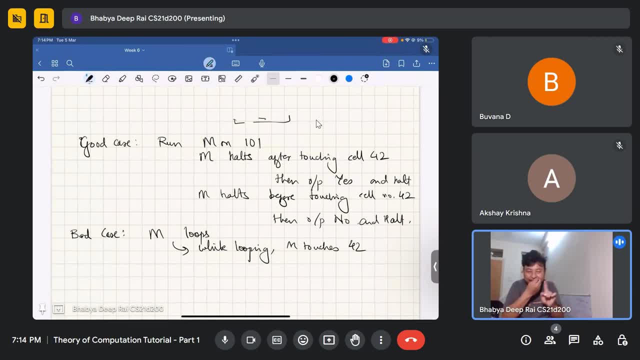 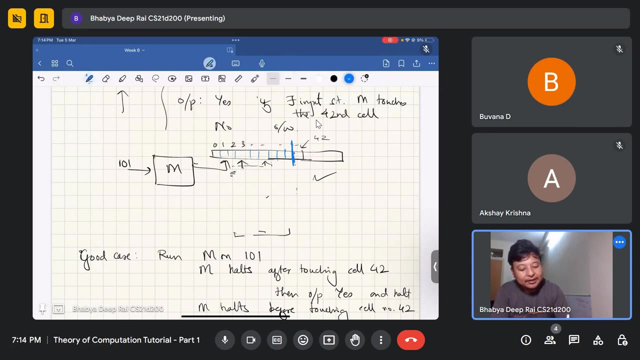 know, since we ran M on 101 and we will keep, we kept checking, okay, we kept checking, it is guaranteed. we are guaranteed to see a case when M touches states 42. for example, okay, I run run M on 101 so it is looping, but it is touching 42 also, it is. 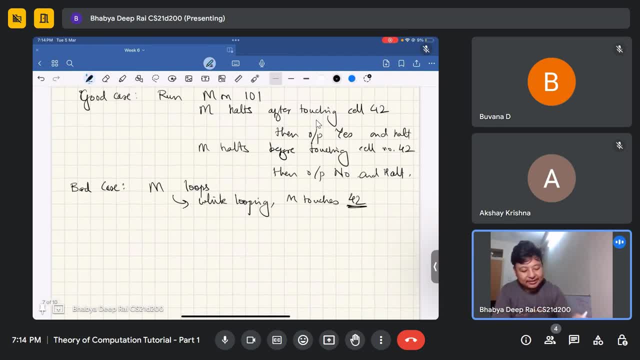 touching 42 also. so this is a good case, this still a good case, this still a good case. let me try to have a close up cut. so the one with Amtouch and if we are able to update the serial number, yeah, when m harness is going again one, it will pong in the spot. 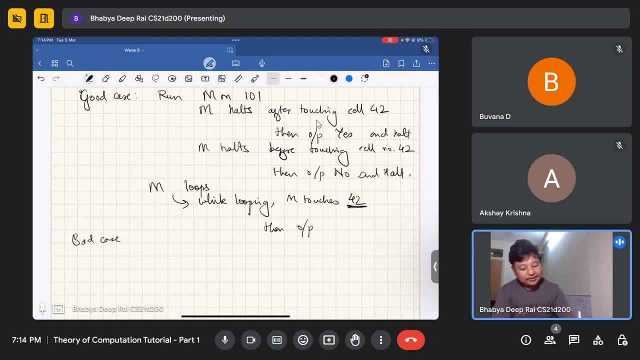 right and a myth here. that's not right. M loops here and touches, then output M saç, Shift out, test M loop the assistant, so this one. okay, we will stay in their oven, so let me output: yes, it touches, and then we'll hold as soon as it touches the 42 cell. 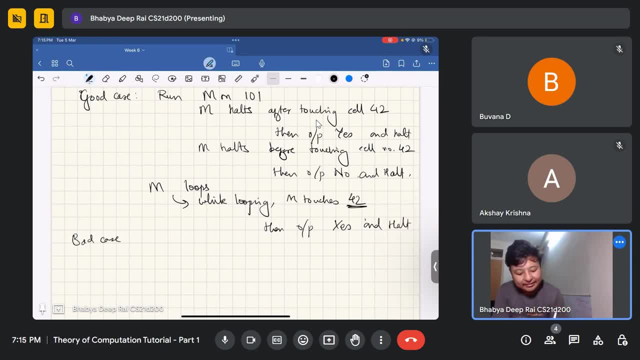 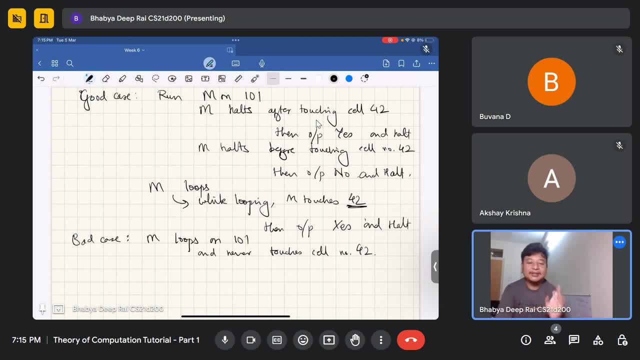 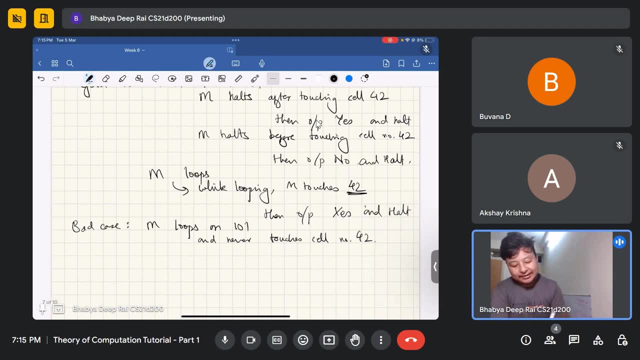 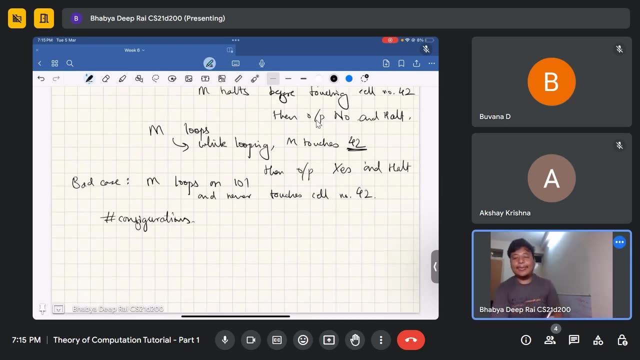 waiting. okay, but it will never touch 42. this is the bad case. question is: how can we detect? how can you detect this? the answer lies in the number of configurations. okay, number of configurations possible. I'll quickly touch on what configuration was and if configuration is the current. 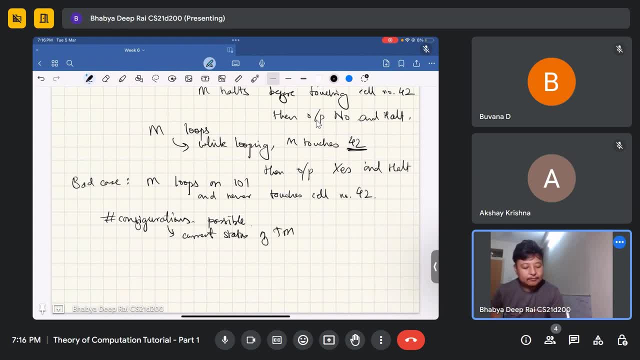 status of Turing machine: okay. what does it contain? okay, current state, which state you are in. okay, head position: okay, and head position and tape content. tape content: yeah, current state, head position. tape content: okay, now, if observe. 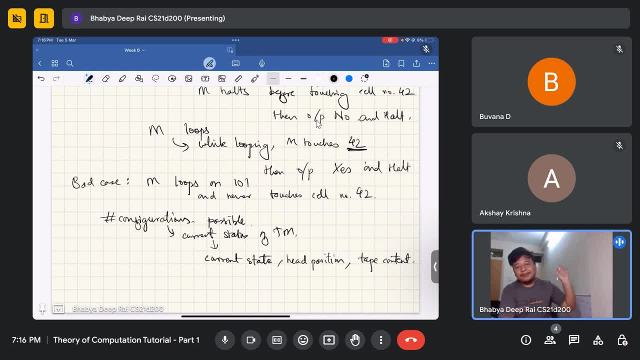 that if my Turing machine has infinite tape length and infinite it loops infinitely, then there are infinite possibilities for the configuration to have. head position could go infinitely wherever it wants. tape content could also have infinite number of possible strings and current string. 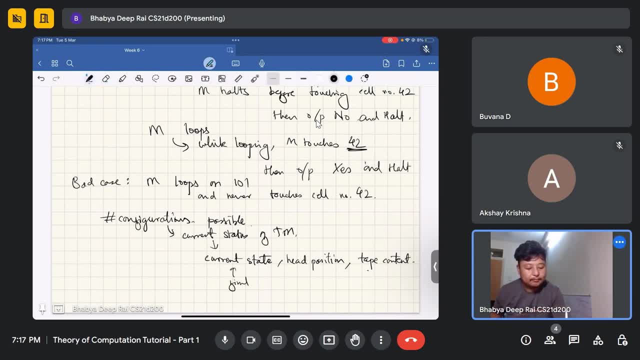 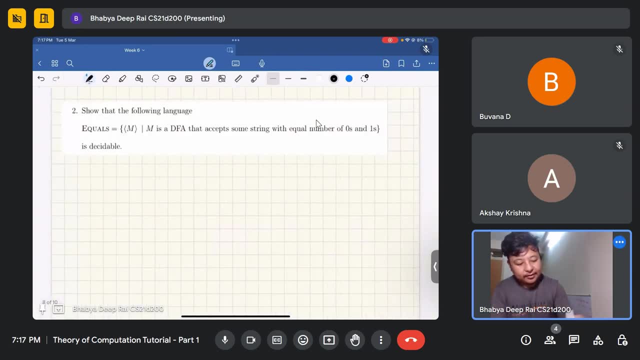 current state. this is at least finite. this is finite, okay, so it will. it will look something like: okay, configuration looks something like: okay, Q0,. I am at state Q1, sorry, not Q0,. let's. 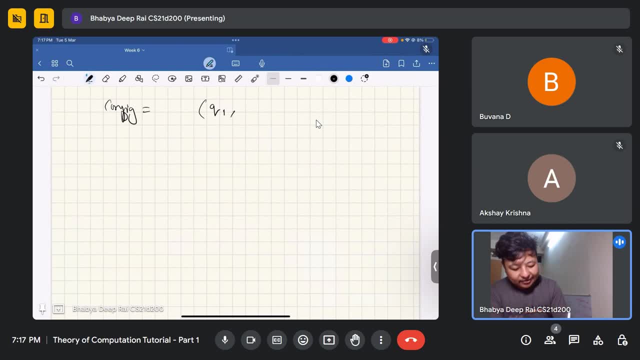 say Q1, and head position is at 21,. this is the head position and what is here? this is the tape content: 10110,. this is what it looks like. and then what can happen on the next step, step 2,, it could move to another configuration. 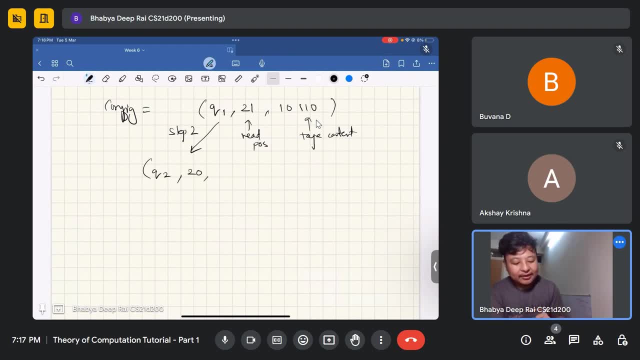 Q2, head position. it could move left or right. let's say it moved left, okay, it moved left and it went back to 20, right and tape content: it is still 10110, and then on step 3, the Turing machine configuration changed. it changed to Q3, okay. 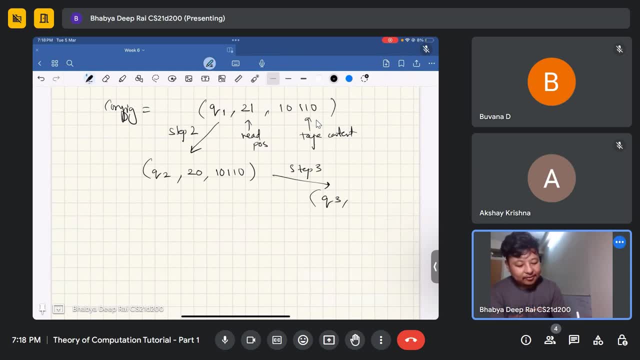 and it went to. let's say right again: okay, the cell in the cell, this is 20,, this is 21,. it moved from 21 to 20, and moved from 20 to 21,, and so on. and let's say: 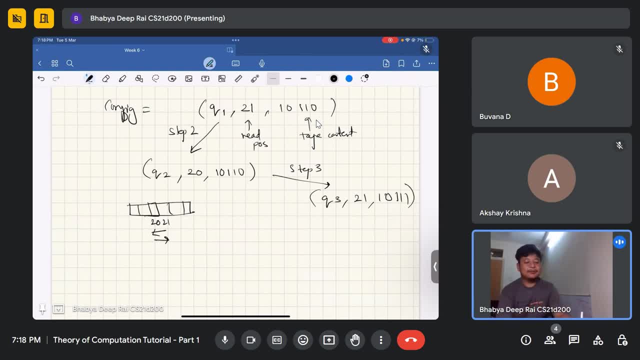 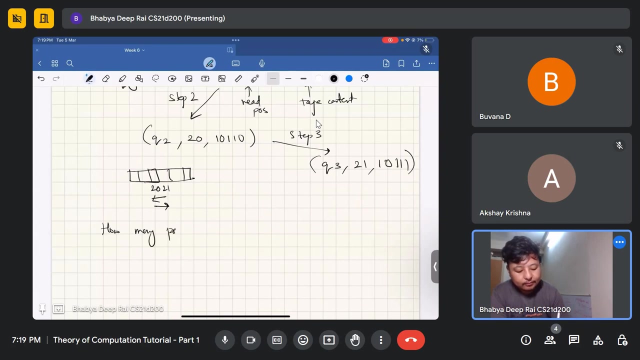 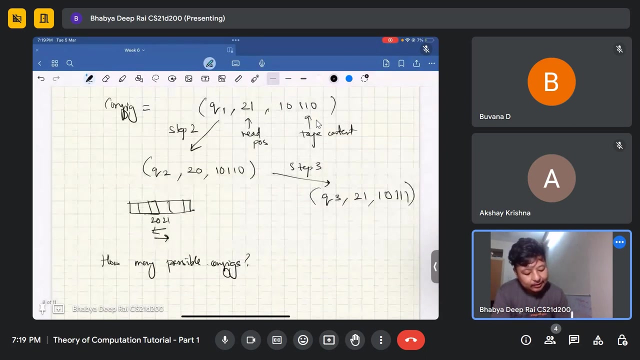 tape content changed: 10111,. now it has become okay. so something like this: this is what happens. it says: question is: how many possible configurations are there? okay, how many possible configurations are there? well, number of states. the first, if the number, if Q is, represents the set of states. 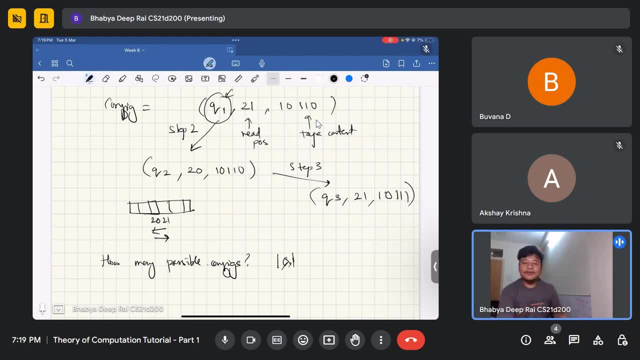 then the number of possibilities here are only number of Q, the size of Q, right times. how many possibilities are there in the head position? three, yeah, oh, by head position I don't mean left, middle, right, I mean 0,, 1,, 2,, 3,, 4,. 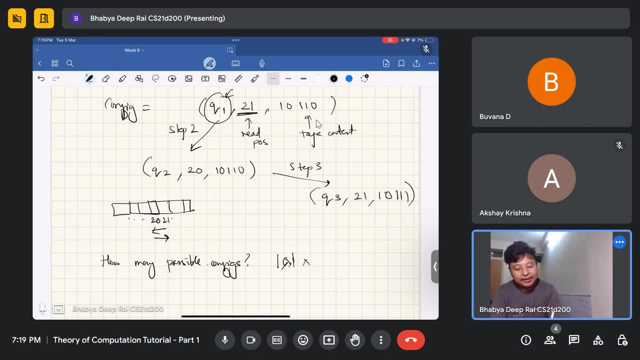 what is the position in the getting it? 0,, 1,, 2,, 3, and so on. that is what I mean by head position. okay, so how many possibilities are there? how many possibilities are in this place? 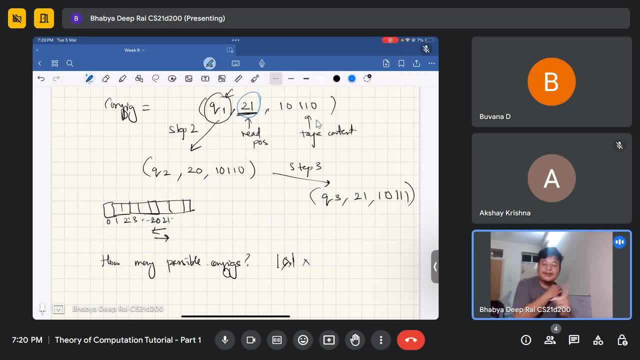 if, if, if, if, if, if it was left, middle left, stay or right, then it is 3, that is correct. but if, if this is what I mean by head position, now what, what? what do you think should be the number of possibilities? 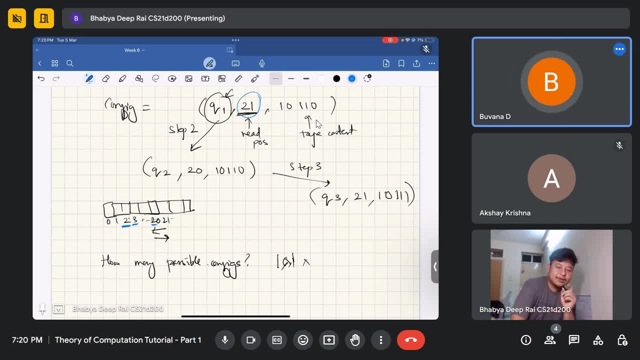 I think both left and right side we have equal possibilities, sir. yeah, but no, but head position, I'm telling you, it does not mean. head position does not mean left, right. head position means, and it is an integer. 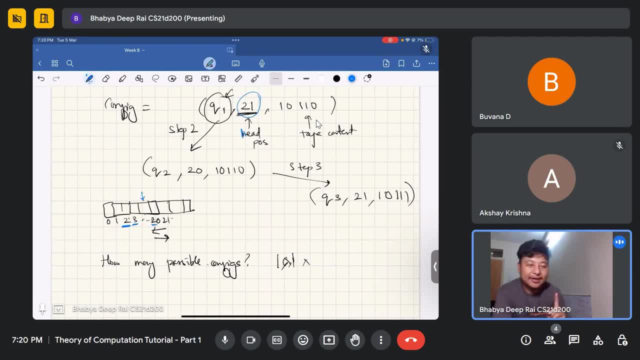 it tells where it is the position cell number. it is the cell number. okay, which cell we are in, whether we are in 20,, whether we are 21,, whether we are in cell number 3, that is what the head position says. 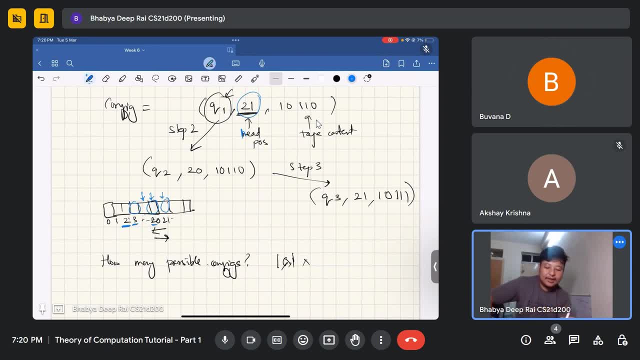 21,. so so yeah, 21,, 20, and so on. so how many possibilities are there? Two possibilities, sir: 21,, 21.. No, I mean that that is in the example I gave, but for a general tuning machine. 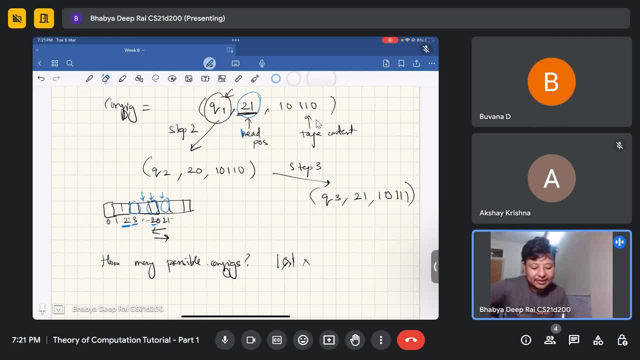 what? what is for a general tuning machine? what is the length of the tip For any tuning machine? what is the length of the tip? Infinite, sir, Infinite, correct. So how many head positions are possible on the tip? 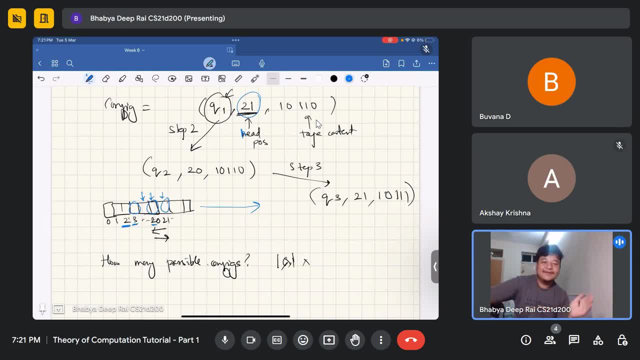 Like, how many cell positions are possible on that infinite tip? Again, it is infinity, Again infinite good. So how many possible configurations? Well, q times some natural number right, which represents, sorry, the, the size, the size of natural number. 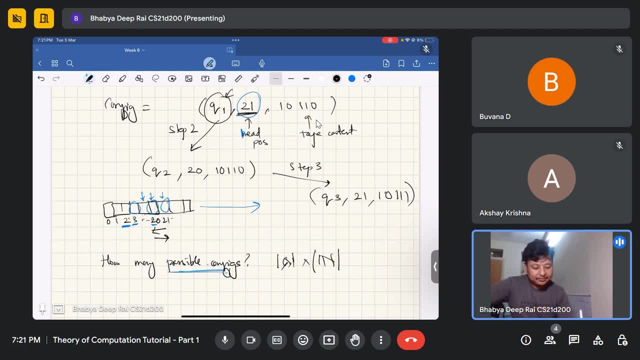 okay times. tip content which is also 2 power, infinity, infinity, Some 2 power. sigma star, oh sorry, size of sigma star, which is also infinite, which is also infinite. This is the tip content. possible tip content are sigma star right. 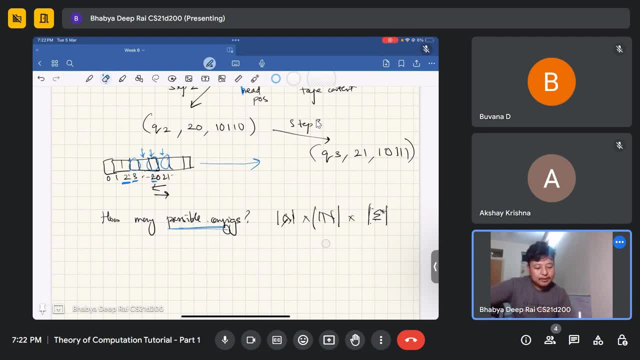 Right, There are infinite possible tip head positions, infinite possible tip contents. Let me know if there is a problem. Yeah, hello, Yes sir, Yeah, this is fine, right, Yes sir, Okay, now, now, now is the interesting thing, okay. 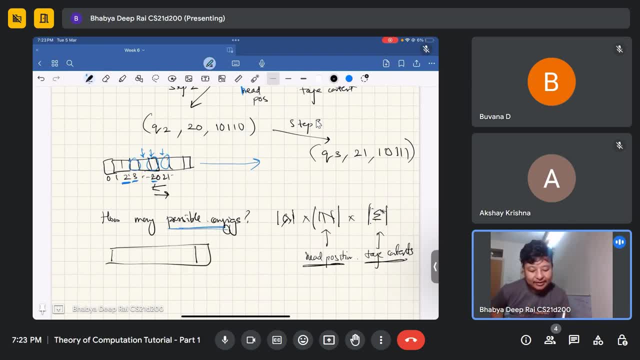 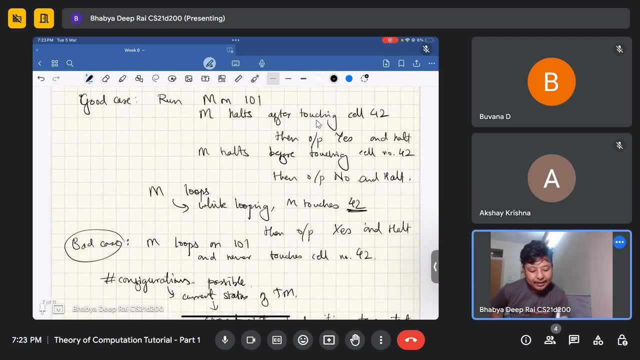 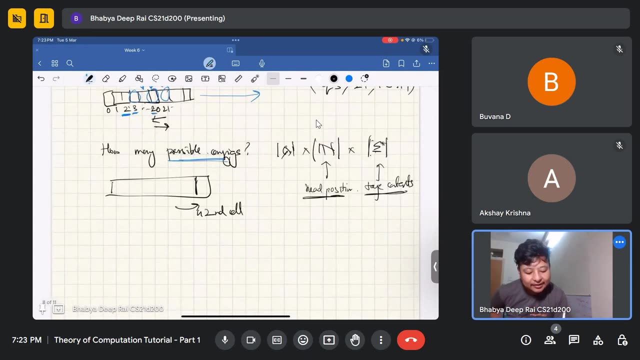 But for our case we are saying: the machine will never go outside the 42nd cell. for this particular case, the bad case: M loops on 101, never touches the cell number 42.. If it never touches the cell number 42,, if it does not ever touch the cell number 42,, 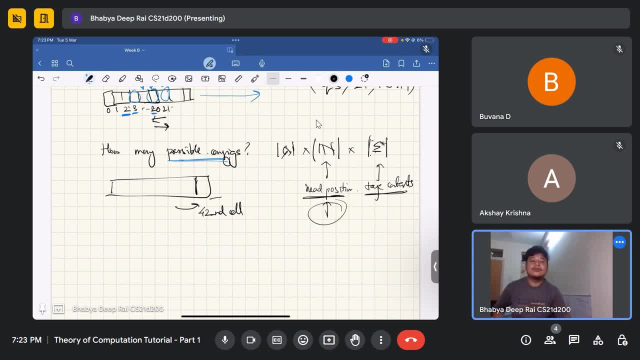 the head position. the number of head position is bounded. now The number of head positions are bounded. What are the number of head positions possible In this case? if it is not just 42,, then 41,, it could be 41.. 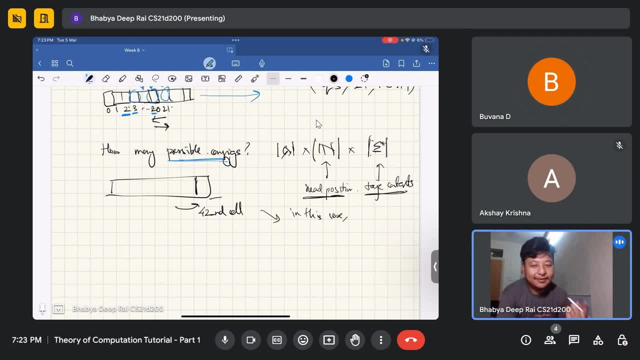 It could be 40. also, It could be 39,, 1234, whatever, until 41.. It could be anything besides 42. And above 42,, right? So in this case I need to charge. just give me a moment, I need to charge my phone. 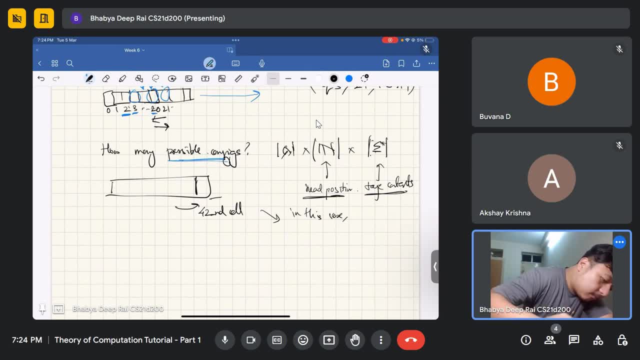 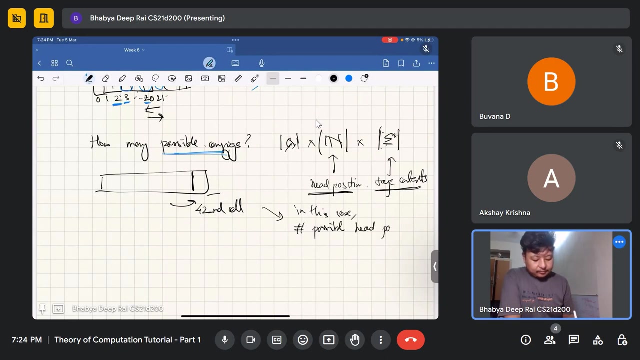 Okay, Let's see if I can charge my phone. Okay, Yeah, So yeah, it could be in this case. number of possible head positions: It could be, you know, it could be 0,, 1,, 2,, anything till 41.. 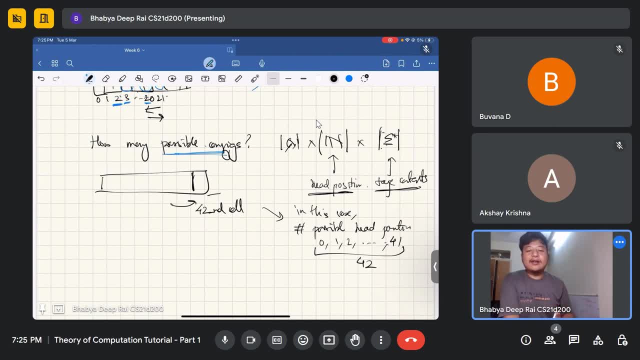 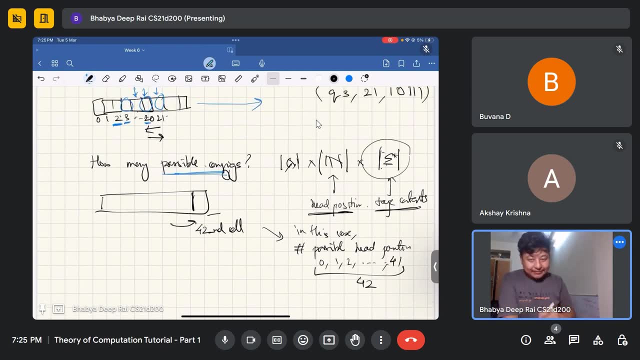 So there are 42 possibilities for the configuration. Okay, And the tape content. the tape content, the, the my, my head never, head never moves past 42nd cell. Head never moves past 42nd cell, So I cannot modify any content here. 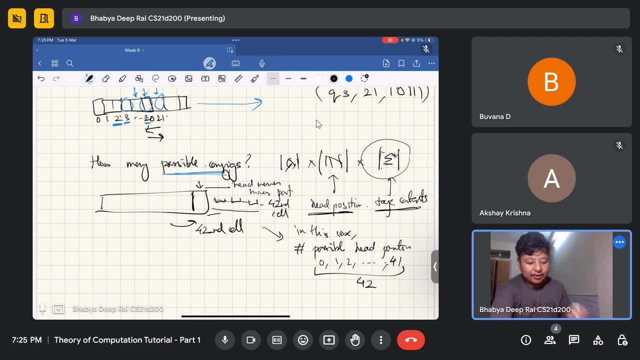 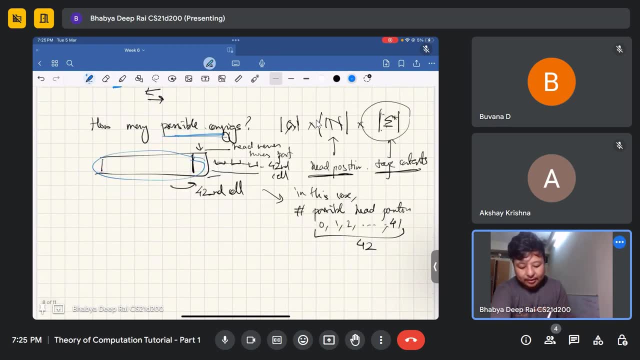 These are all blanks. So what is the only possibilities for my tape content? This area which could be either 0 or 1.. So this area which could be either 0 or 1 or whatever. So how many possibilities are there? 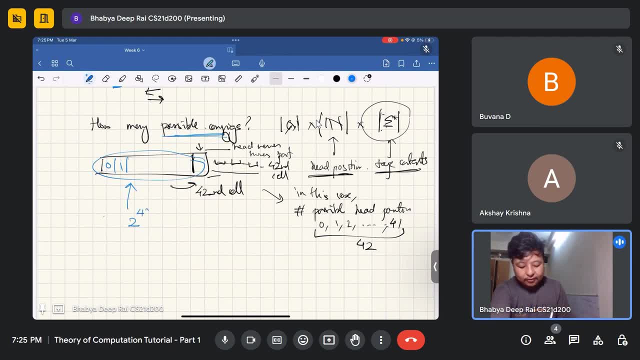 Well, 2 to the power 42. Okay, Okay, So Getting it. So this infinite number of configuration is now finite. for us Now, number of possible configurations is equal to number of states, which is already finite times number of head positions. 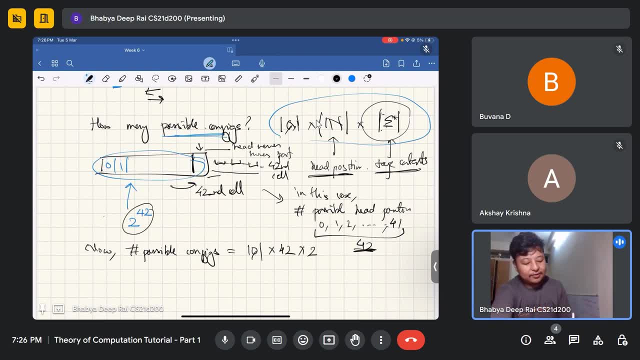 42. Times. Number of possible tape contents: 2 to the 42.. This is the maximum number of possible configurations I have, Since my head is never moving away from the 42nd cell, only getting it. Since I'm not moving past the 42nd cell, the head positions okay. number of possible head. 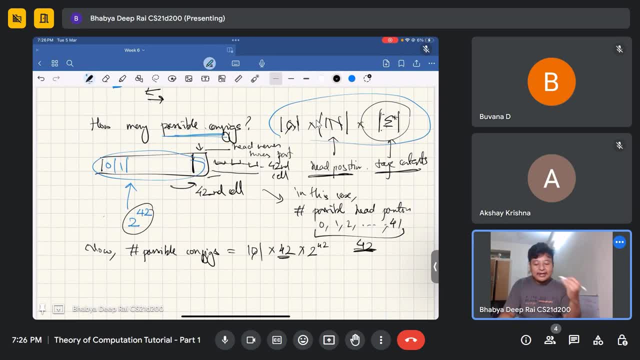 positions is bounded by 42. And And the number of possible tape contents is also bounded, because I cannot write on it, write on a cell that is past 42. So the length of the string is that most 42. So how many number of strings are there which is of length 42.? 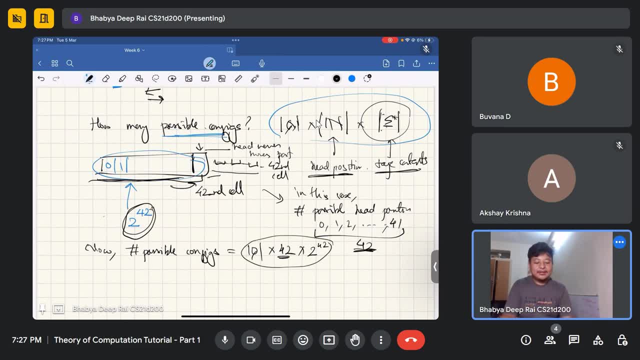 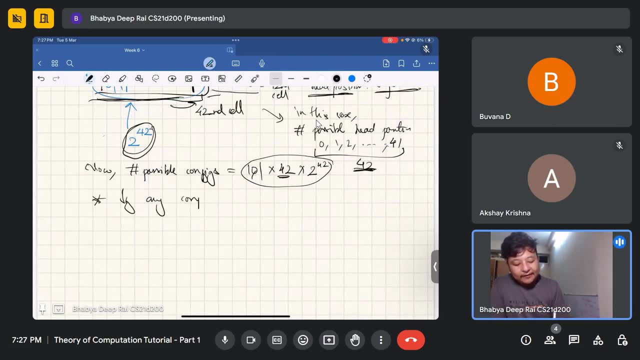 Well, 2 to the 42.. So this is the number of configurations, Now the main. The final observation is that If Any configuration, If there is a loop, Then If there is a loop, Then there is a loop. 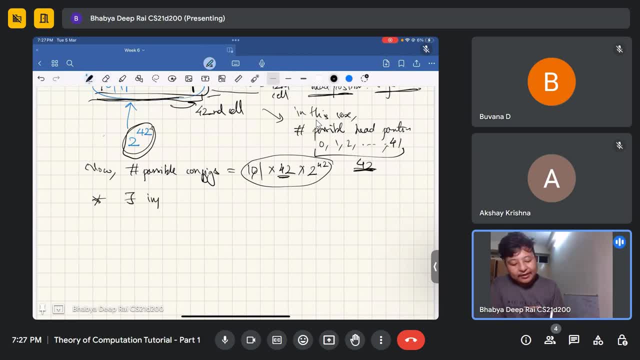 Then there is a loop, There is an infinite loop. some configuration is repeated. so run my Turing machine for Q times 42 times 2 to the 42 steps. If 42nd cell is still not touched, then because if it means it takes more than this many steps. 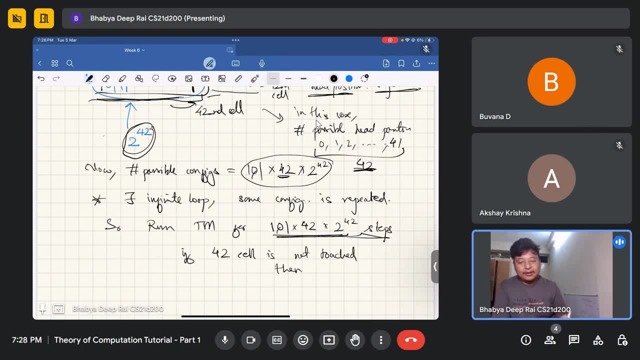 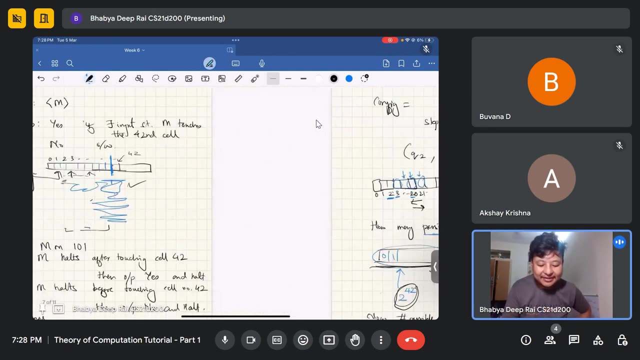 it means definitely, I have entered a loop, Then output: yes, are you getting this? Yes, sir, Right. so even what is the lesson here? even though it might seem deceiving for us, even though it might seem deceiving that this looks like an undecided problem, because I'll just 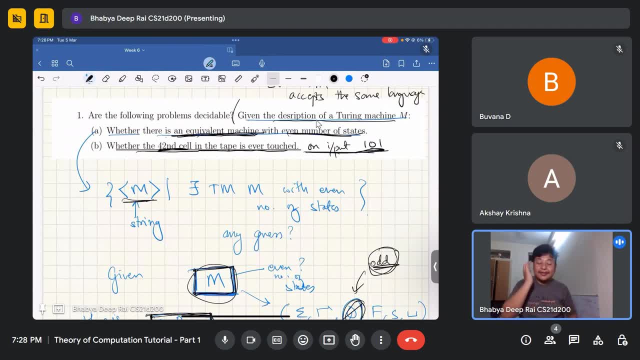 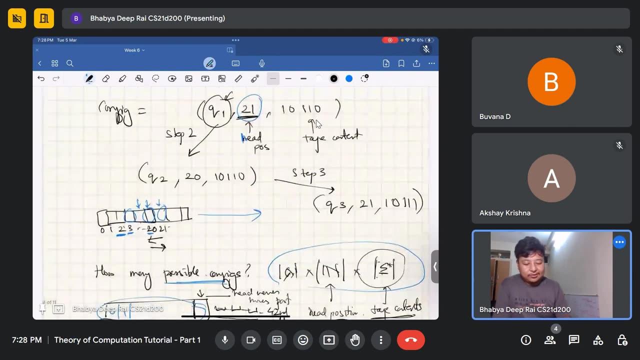 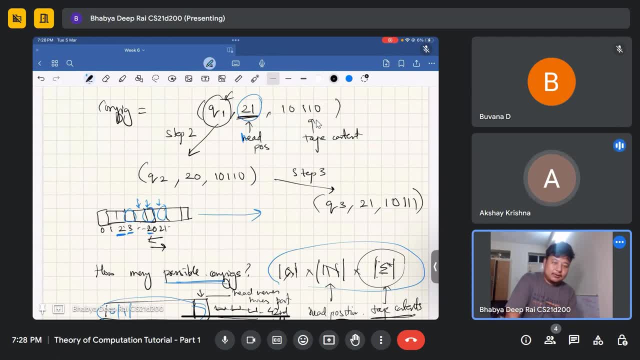 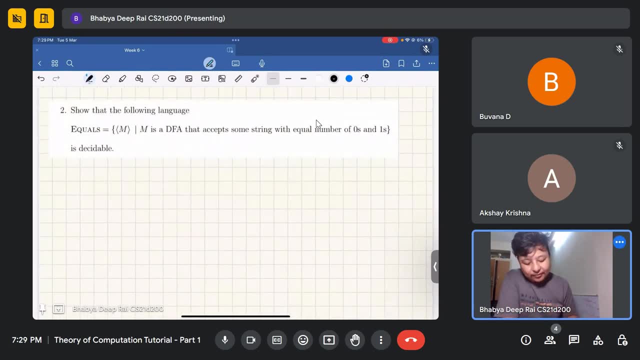 Yes, sir, Okay, good, Okay. so, guys, let me know if anything you want to ask. okay, okay, so we'll quickly look into these questions. okay, I'll do the first one, then the remaining, please tell. 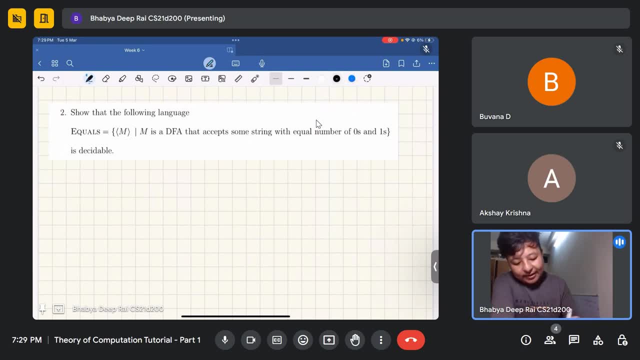 me what some suggestions. Okay, so here I'll demonstrate the first one. Okay, So that the following language equals: which takes a description of this. this denotes the description of Turing machine M. Okay, And such that M is a DFA that accepts some string with equal number of zeros and ones. 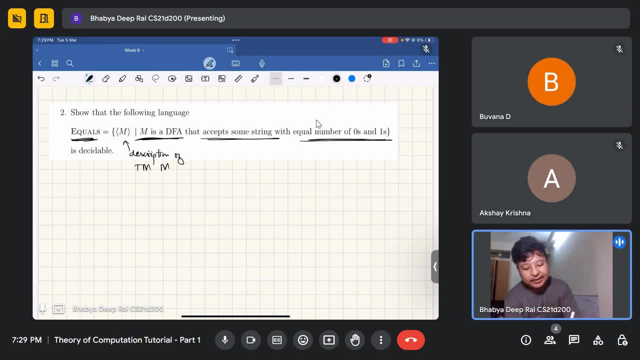 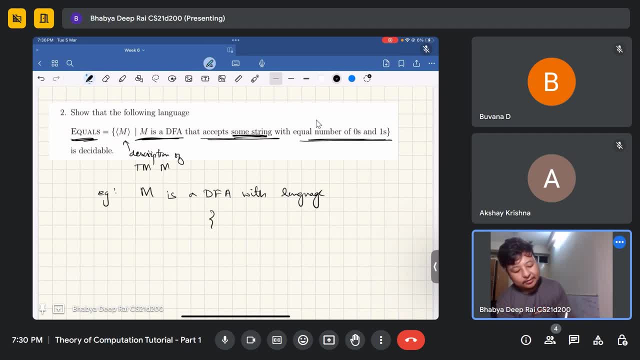 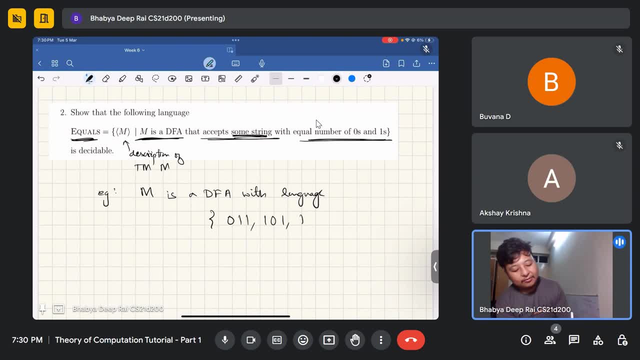 1, 1, 1, 1, 0, 1, 1, 0, 1, 1, 0, 1, 0, 1, 0, 1,, and so on. 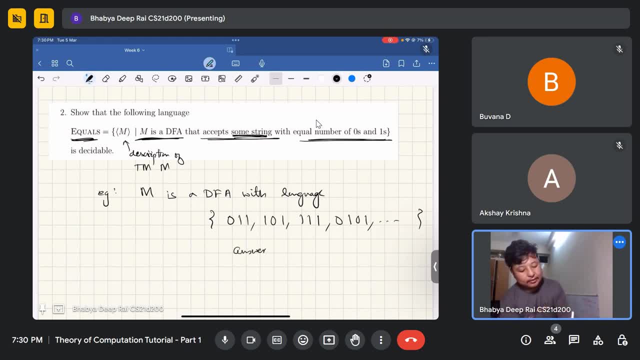 Then answer is yes. My total Turing machine should say yes when given this DFA as an input. Why? Because this guy has equal number of zeros and ones. Okay, What is the problem here? What is the problem? Okay? Problem Simulating: 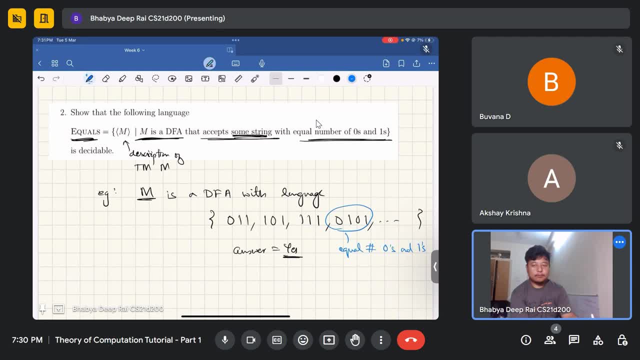 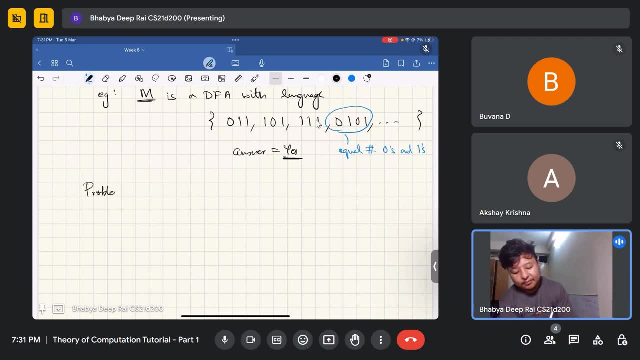 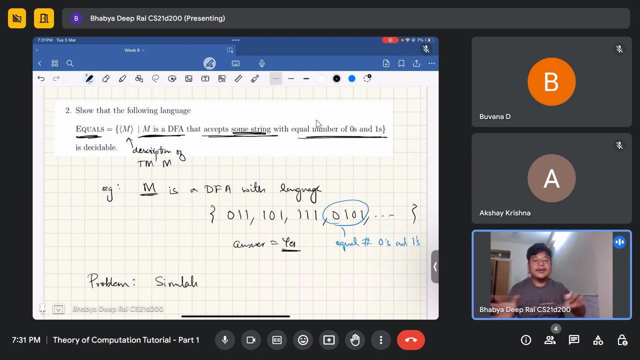 One direct approach is what I take- one possible input. Let me take one possible input. What is the direct approach? I take one possible input. What is the direct approach? I take one possible input. Let me take one possible input. I put it through the DFA and simulate it. 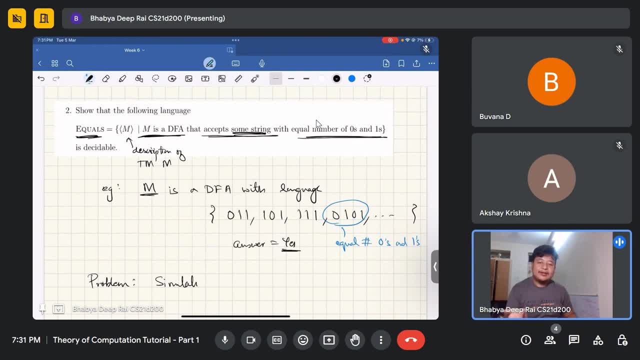 Run it On zero, Then I wait and it will give me the answer. Then it will give, Then I will do 1.. And then it will run on 1 and then give me the answer. Then I do 0, 1.. 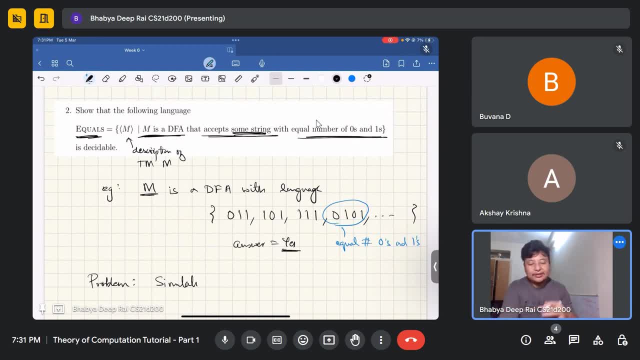 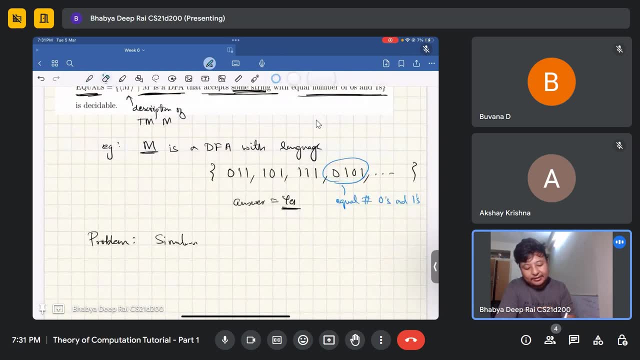 Then on 0, 1, it will run and give me the answer Okay, And so on, And okay, Let us say problem. This is the simulate on. let us say One, Two, let's say 0, 1, 0 0, 1, 1 0, 1 0, 1 0 0, 1, 1 0. okay, 0, 0, 1, 1 has already done 1 0, 1 0. 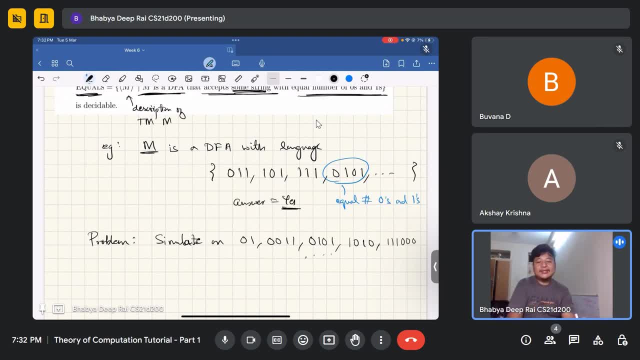 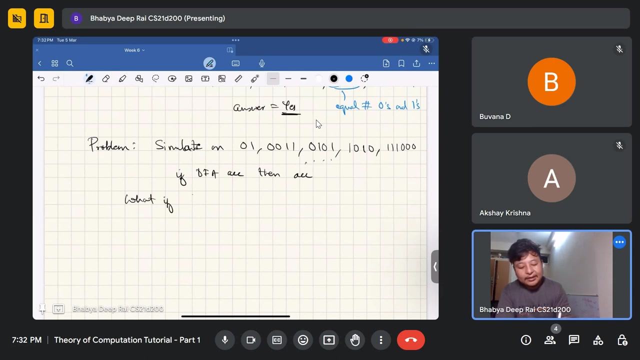 and 1, 1, 1, 0, 0, 0 and so on. all these strings have equal number of zeros and one. simulate on. i'll simulate it on all strings that have equal number of zeros and ones. if dfa accepts, then accept. but what if? problem is, what if there does not exist a string? 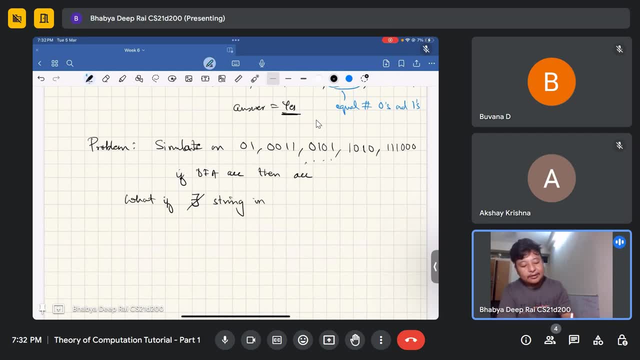 in the language of m language of the dfa, such that there are equal number of zeros and ones. what if there is no string in the language such that there is equal number of zero? that means the dfa will never accept it. any language which means dfa never accepts. 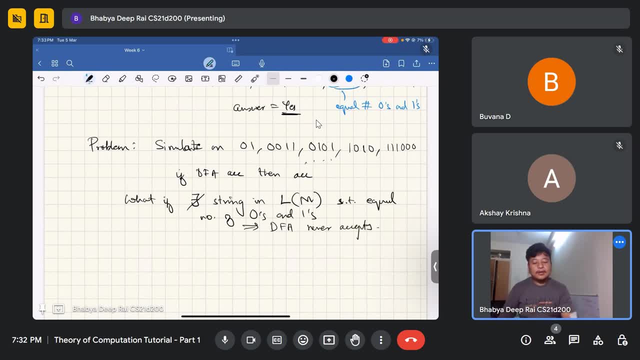 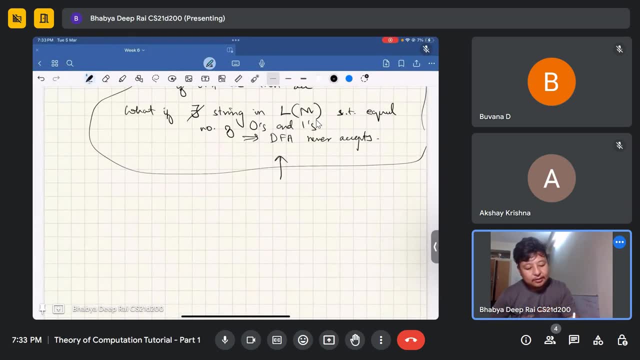 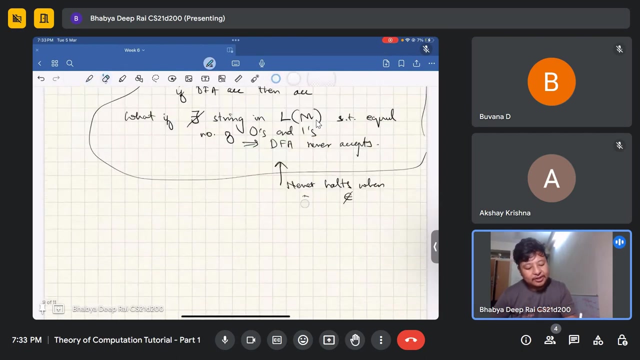 so this simulation will never end. in that case, this never halt. when dfa does not belong to equals or machine m description: machine m does not belong to this language, equals will. when the machine will never accept a string which has equal number of zeros and ones, this simulation will never run. so does that mean it is undecidable? well, there is a more. 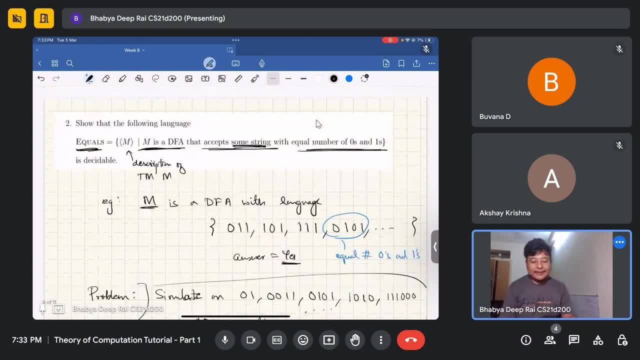 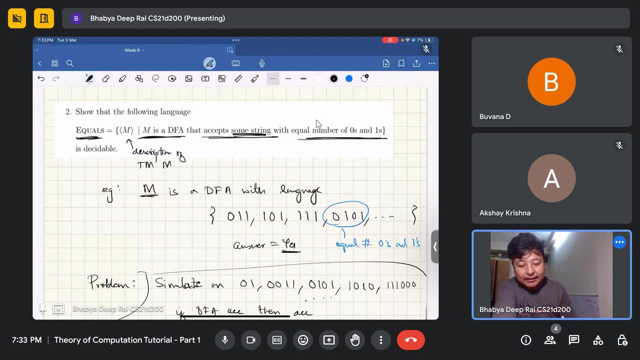 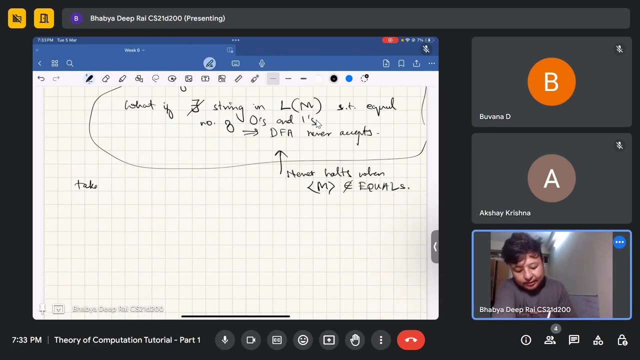 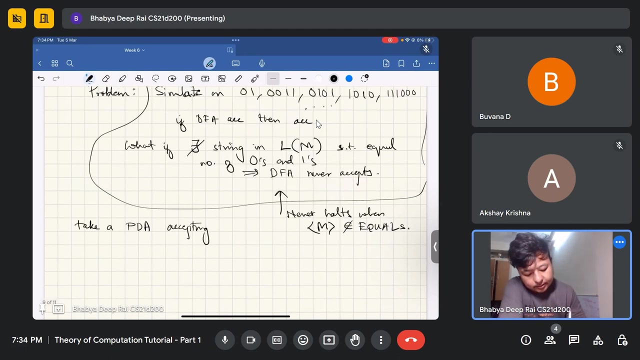 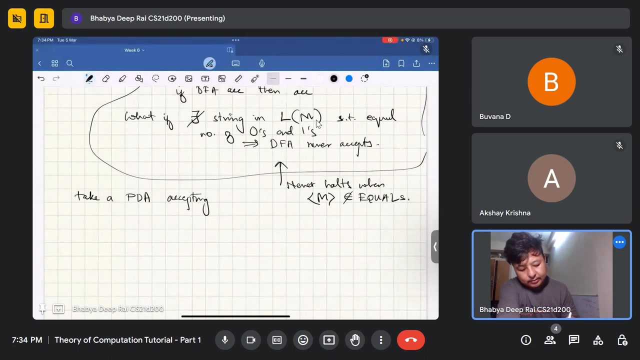 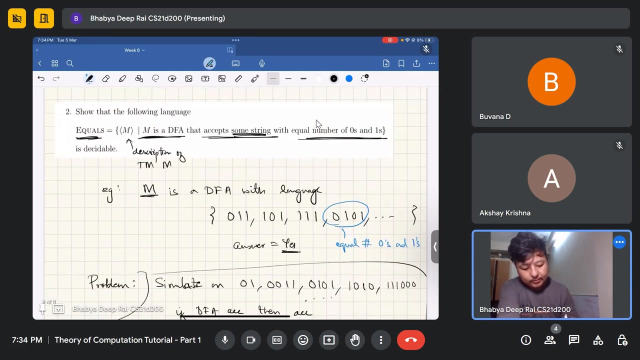 clever way to do this. okay, that is the more clever way to do this. and look at this technique carefully. okay, what i'll do is i'll take a dfa, not a dfa. take a pda. okay, accepting Seit count what. there's a problem with this, actually? 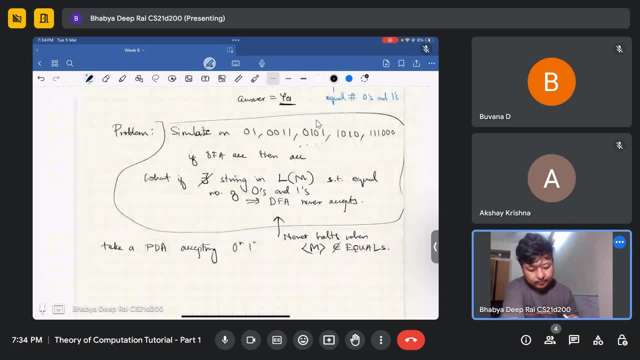 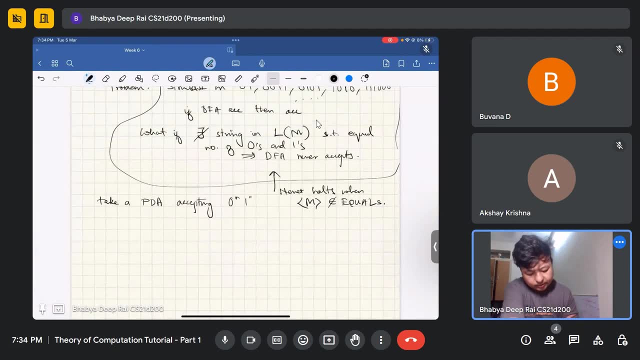 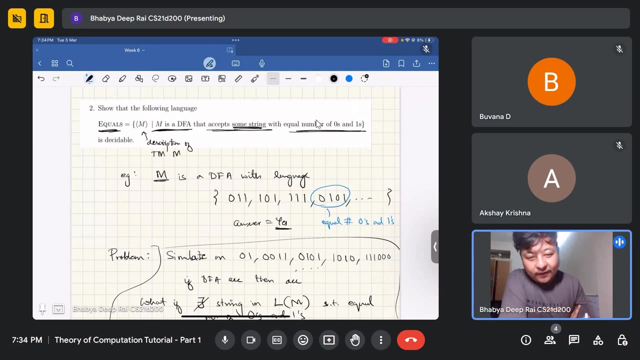 there is a problem with this. actually, that's the problem with this, actually Все the problem with this, actually. okay, i'll slightly modify this question. okay, equal number of zeros and ones um ones follow. sorry. where zeros followed by ones. okay, okay, where zeros are followed by ones. 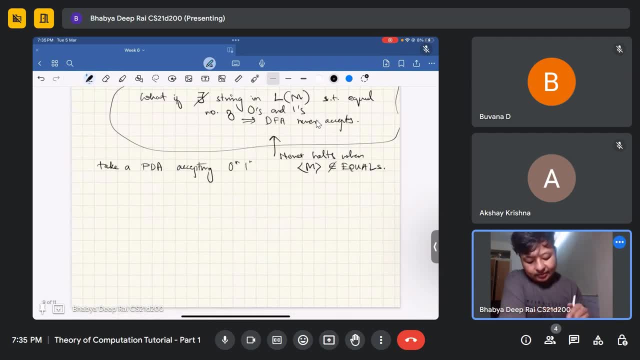 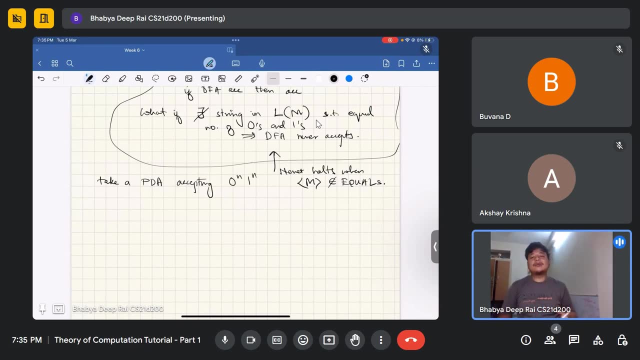 so okay, now let's try PDA. so take a pushdown automata accepting 0 to the n, 1 to the n. why is there a pushdown automata? why is there a pushdown automata? because 0 to the, because 0 to the n. 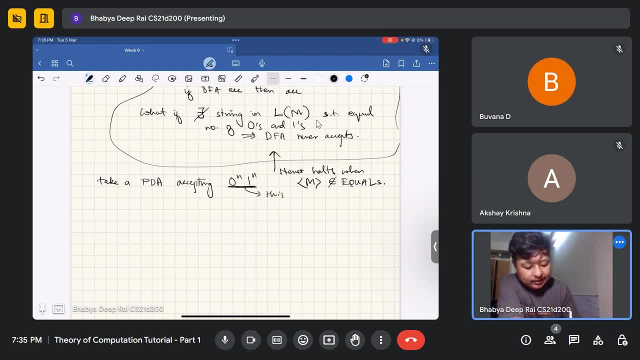 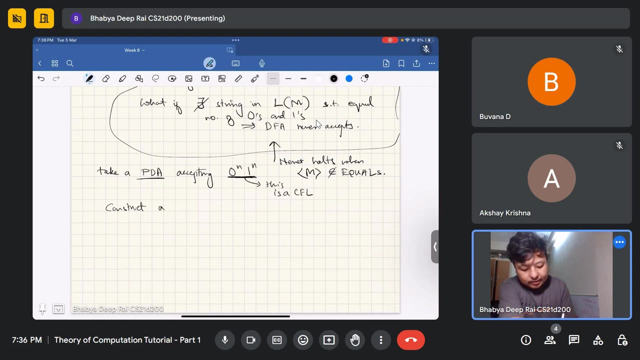 1 to the n is a CFL. this is a CFL context free language, so pushdown automata always exists. so what do i do? i will construct a, a a construct a PDA, okay, such that it accepts. okay, let me call the PDA n, okay. 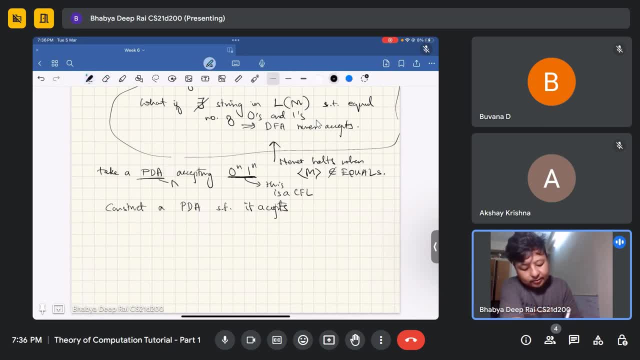 i'll call it n. okay, i'll call it n. it accepts the language of n intersection. this is a PDA. this is the DFA. how do i do this? using subset construction. okay, construct a PDA which accepts the language of an intersection- language of n- using subset construction. 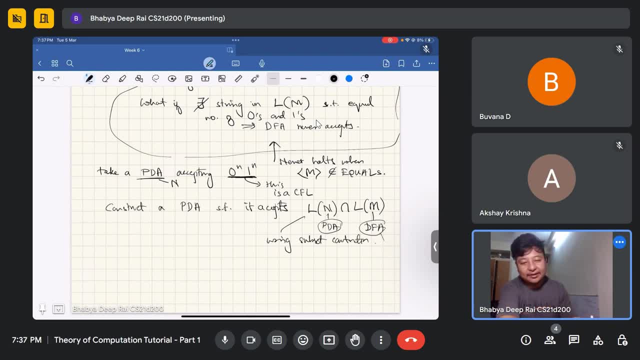 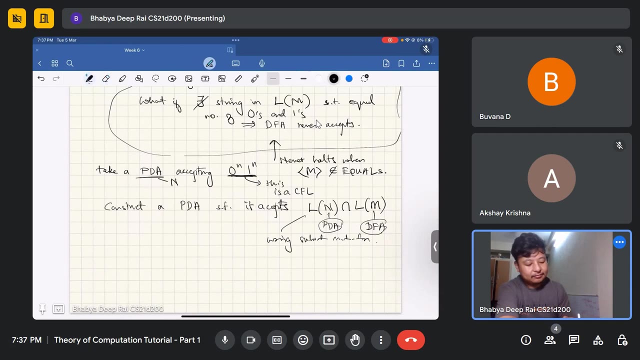 why can i do subset? Because DFA is also a PDA only, So the same mathematical definition will still apply. So DFA is just a PDA that does not use a stack. So, using subset construction, I got this And I will call this machine MN, N, NN, PDA, MNU. let me call this MNU. 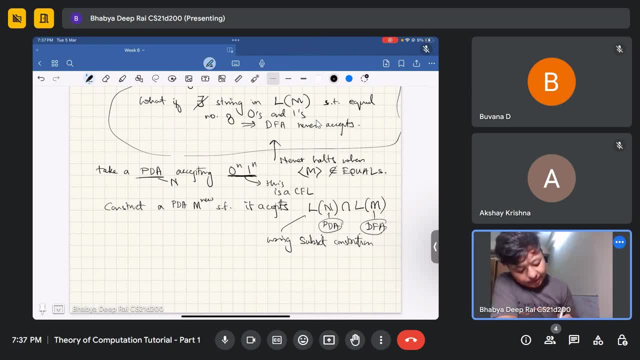 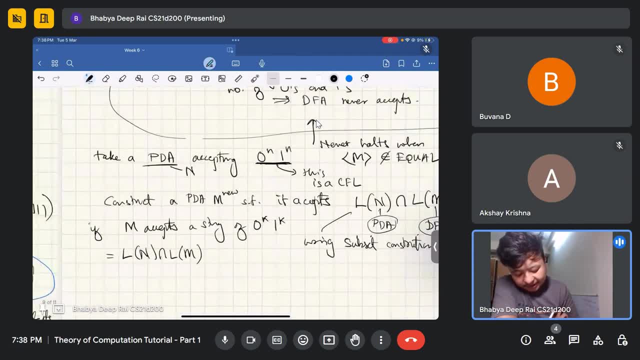 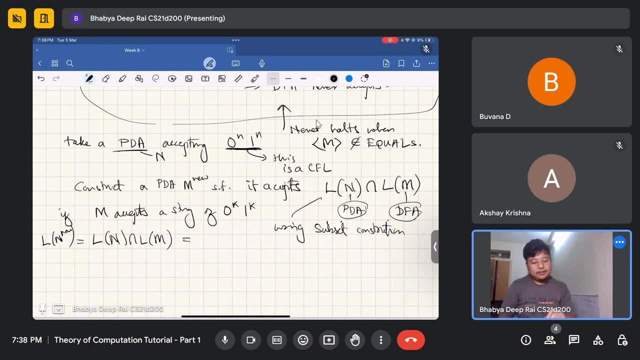 0 to the k: L' L' L' L' L' N, L' N, NNU, NNU. so this accepts 0 to the n, 1 to the n and this accepts some arbitrary language. okay, but we know that M accepts at least one string of the form: 0 to the K, 1 to. 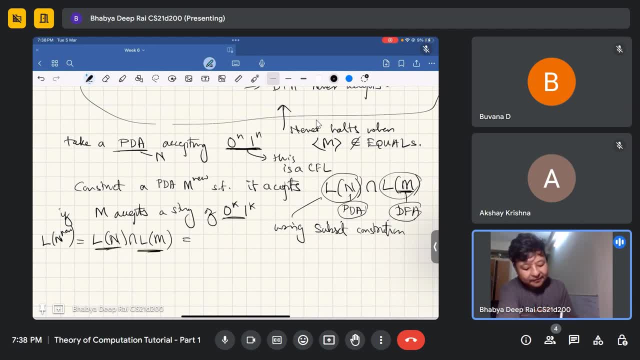 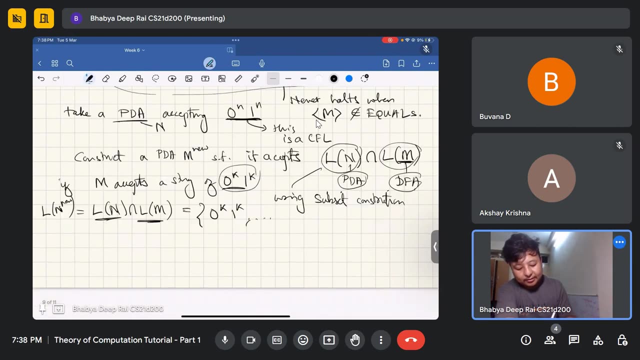 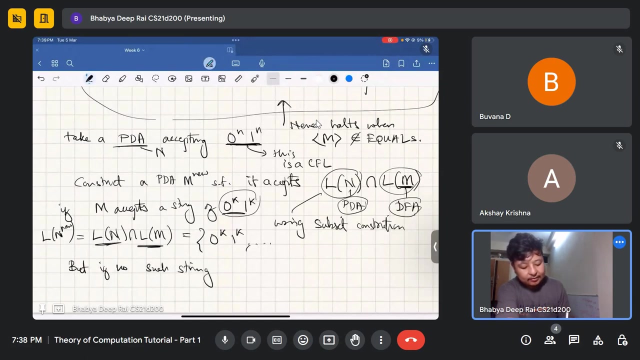 the key, then L of M, L of n, intersection L of M will definitely contain L of K. 1 to the key, 0 to the key 1 to the key, because this string is common between them getting it. but if no such string of the form 0, the key 1 to the key is: 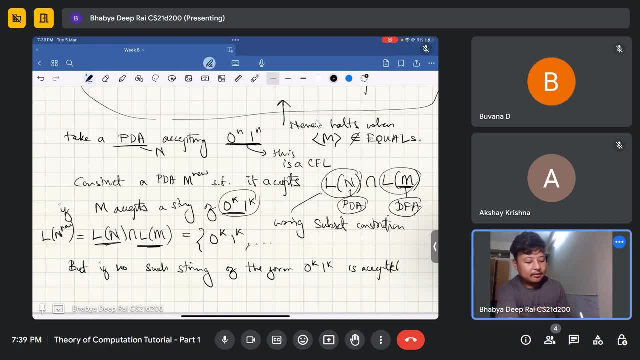 accepted by M, then what'll intersection B? since there is mode such string which L accepts, and L always has strings of the form 0 to the n, 1 to the n or 0 to the k, 1 to the k, their intersection is empty. 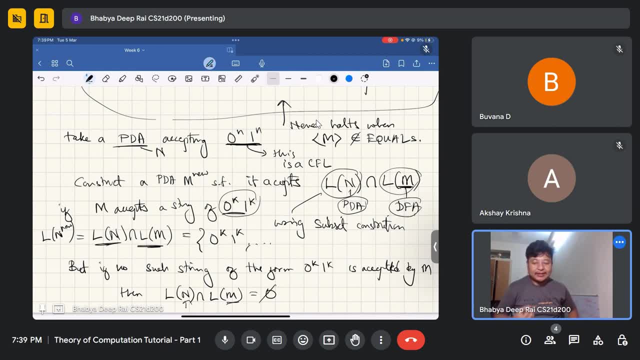 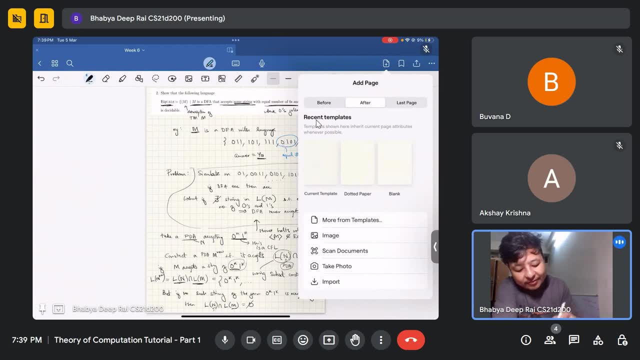 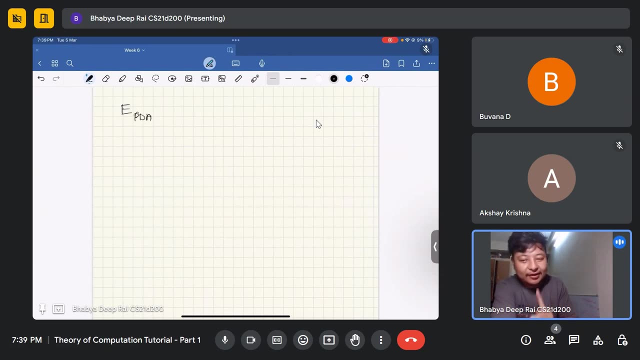 No such string exists, then their intersection is empty. So therefore, you almost have your answer. What you need to do is you need to remember that this E PDA, which is done in the lectures. okay, that is checking if PDA language, checking if language of PDA is empty or not, is. 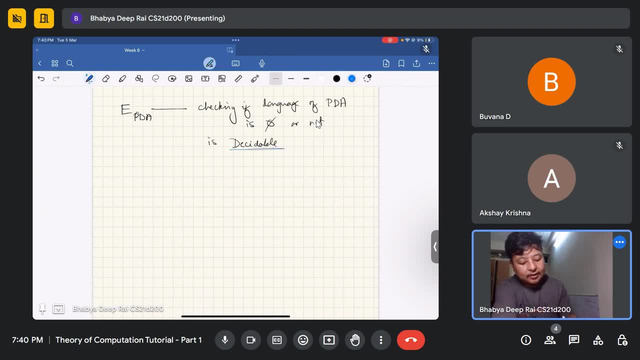 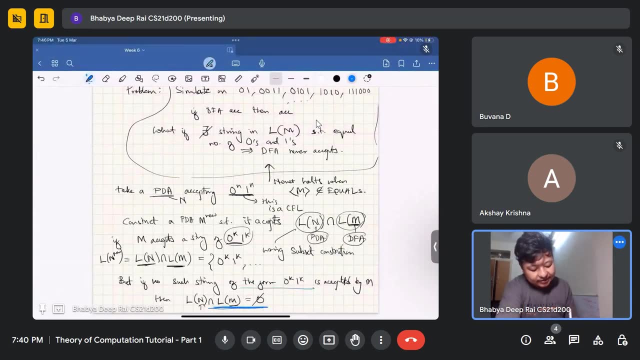 decidable. So here too we are doing the same thing. If it does not accept a string of this form, then the language is empty, the construction is empty. and if it does accept a string of the form- 0 to the k, 1 to the k- then the language is not empty. It has 0 to the k, 1, at least 0 to the k. 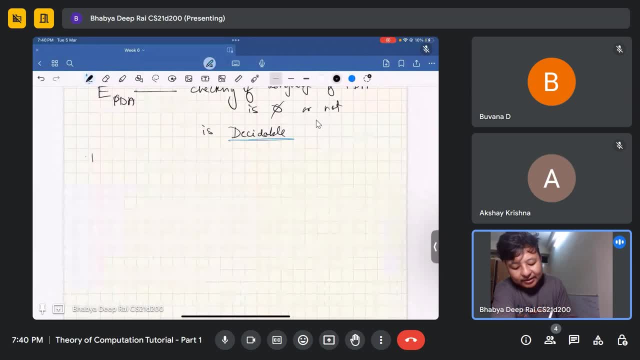 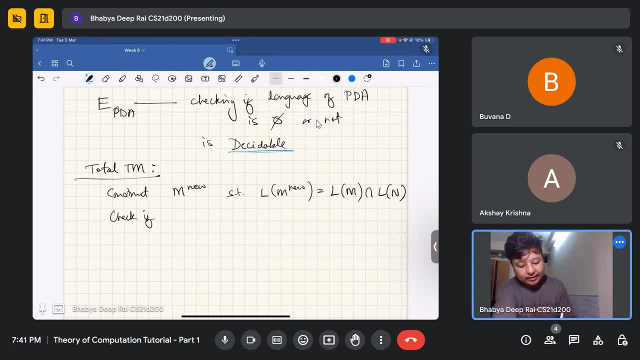 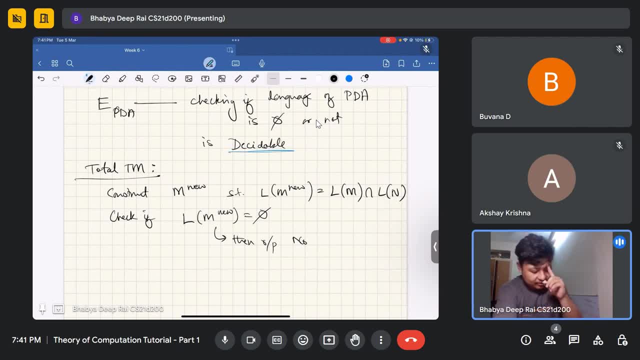 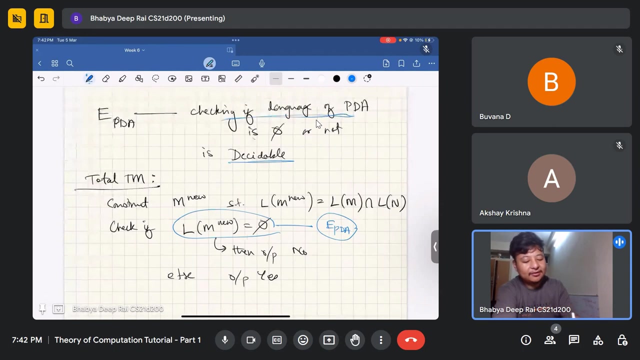 no, sorry, sorry, just the opposite. if it is not empty, then it accepts and else output. yes, and this thing is nothing but same as EPDA checking. whether the checking if the language of EPDA is empty or not, it is decidable, and this part is decidable. 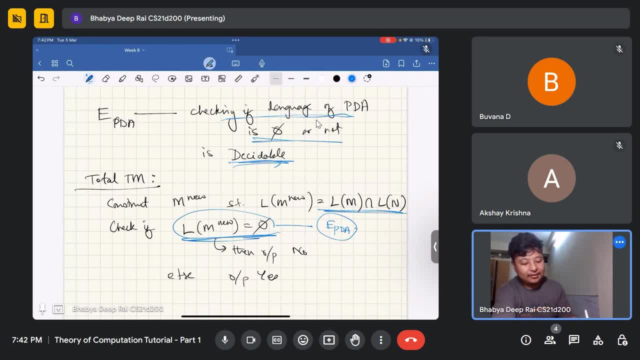 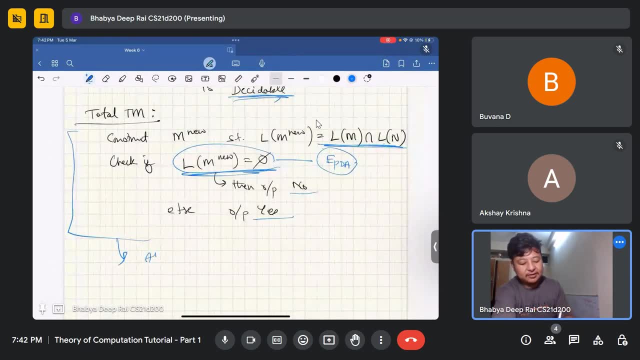 and this part is also, you know, it will never halt. I mean sorry, it will always halt and these parts will always halt. so this machine always halts. So language of sorry, this question, the language of the question equals, is decidable. 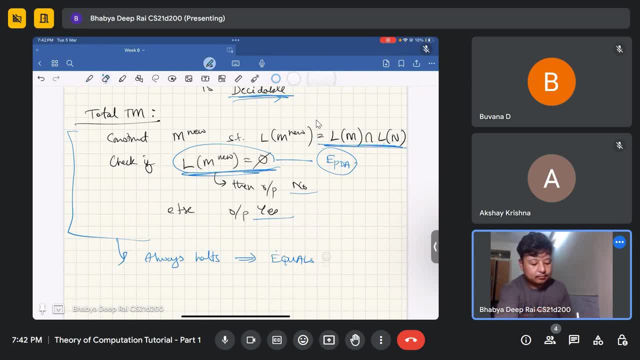 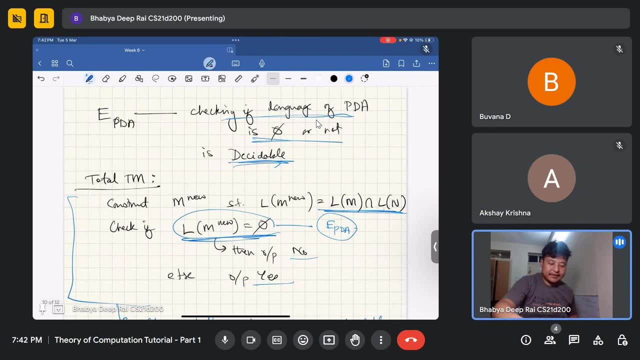 To repeat what I have said, we want to check whether the given a DSA, is it true that it accepts a string of the form 1 to the 0 to the k, 1 to the k, or, in other words, I also. 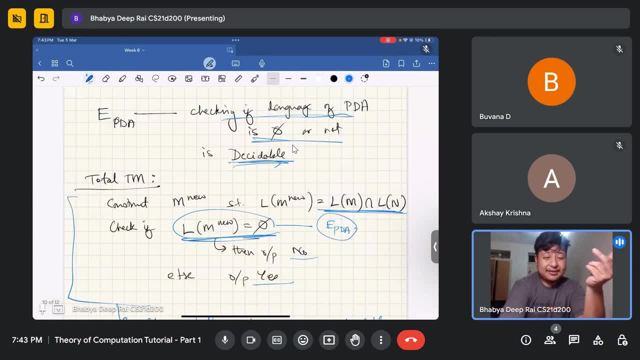 said equal number, 0 to 1, where 0s are followed by 1s, Which simply means 0 to the k, 1 to the k. So what did I do? I took a CFL, which is CFL. what is the name of the cf? what is the? 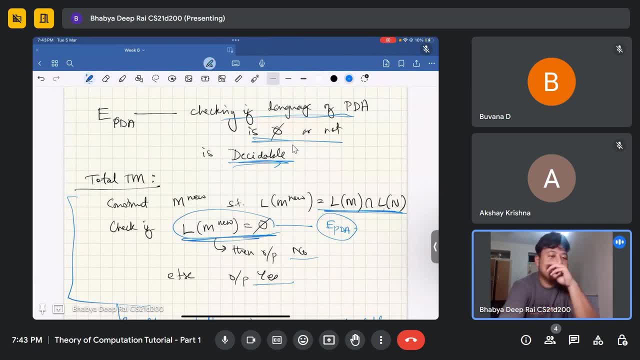 language, 0 to the n, 1 to the n, and we know this is a CFL, so it definitely has a push-down automata for it. What I'll do is I'll do. I'll construct a new push-down automata that accepts the intersection. 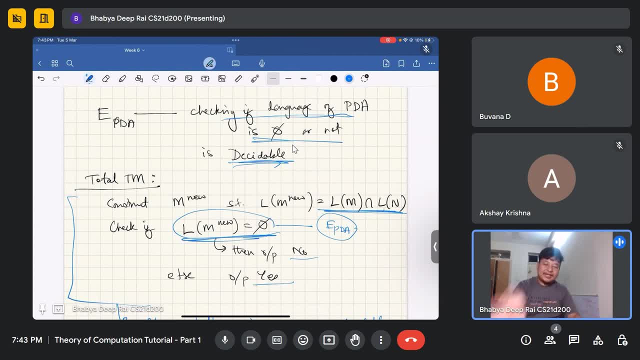 of the this of the DSA, So I'll do, l'll do this, So that's it. So that's it. I hope you have understood of the language of the DFA that I have and the and this new, sorry, this pushdown. 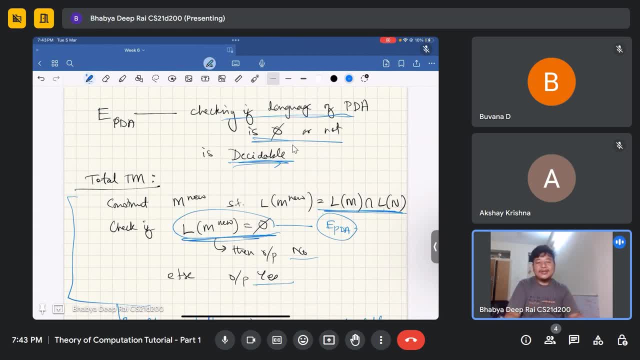 automata a computing: 0 to the n, 1 to the n. if it so happened that the machine M accepted a string of the form 0 to the k, 1 to the k, then the intersection definitely would have been non-zero. otherwise their intersection would have. 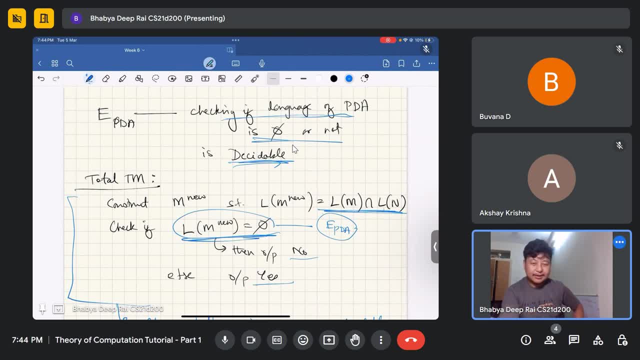 been empty, otherwise, meaning it M does not accept any string of the form 0 to the k, 1 to the k, then the resulting language of the intersection would have been empty, and if it is empty, then we would output. no, if it is not empty, then we would. 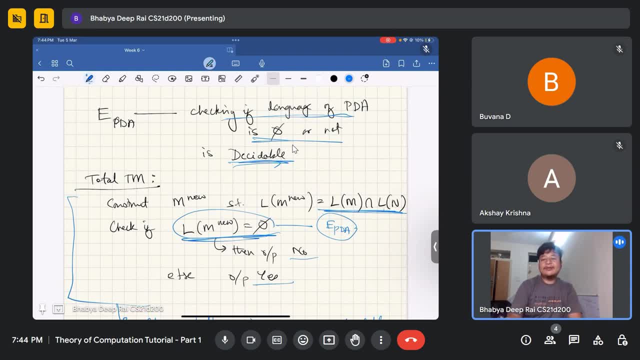 output. yes, checking whether the language of a PDA is empty or not is nothing, but what is called E PDA, and E PDA is decidable. that is what we saw in the lectures. so is it clear, or what's this? okay? yes, sir, I have understood partialism, okay. 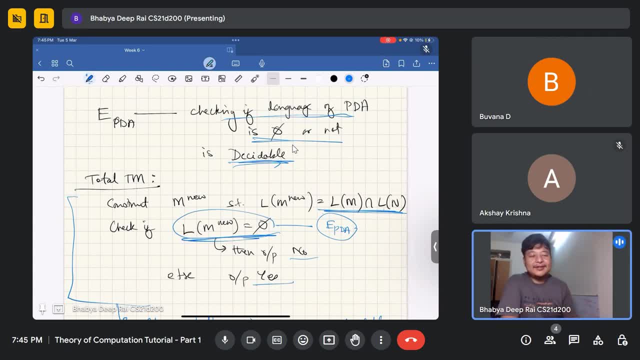 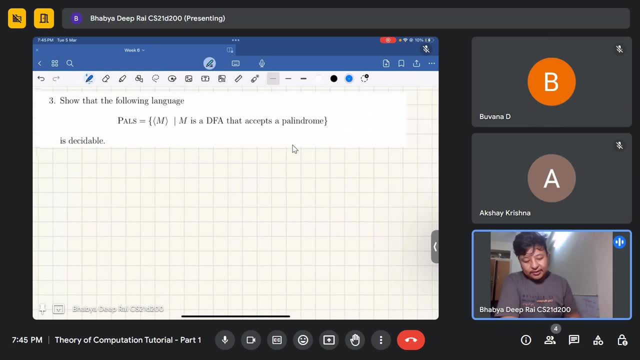 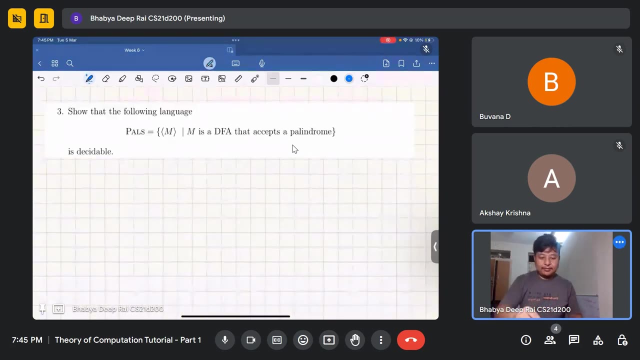 the that that if you see the next one, you'll fully understand. okay, okay, so here is the next one. okay, here's the next one. oh, we are okay, we have some time left. here's the next one. okay, similar flavor again. i want to come up with a push down automata or a dfa and finally do. 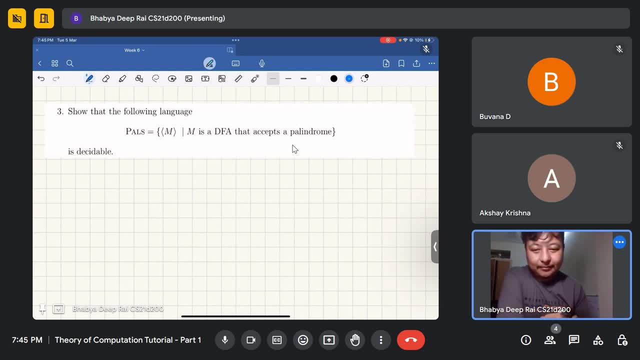 an intersection and then talk about their emptiness. okay here. here is the question: given a machine m check if the dfa ever accepts a palindrome or not, okay, so i i want to do again l of m intersection. i want to construct a pda such that 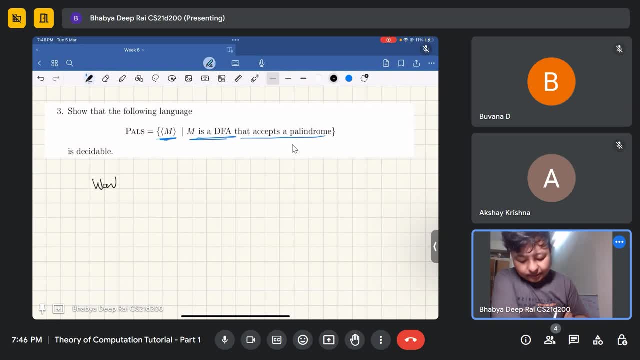 want to construct pda such that l of m language of my new pda, m new is language of the machine, language of the dfa given to us intersection language of n. okay, now, what should this language of n be? that is the question. okay, and why? why do i need this? so that 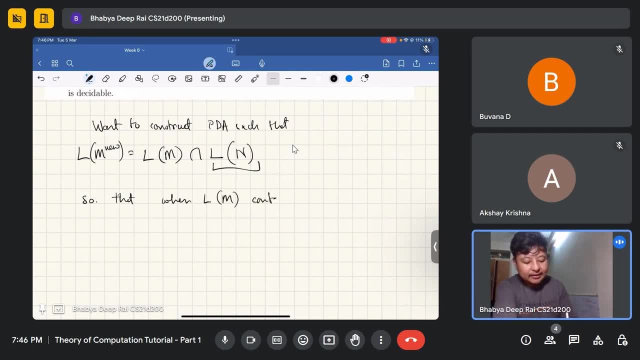 when lm contains a palindrome. when lm contains a palindrome- i love language of- contains a palindrome. this, this language of m new, that is the intersection. this language of m new, that is the intersection. this language of m new, that is the intersection, is this language of m new, that is the intersection, is. 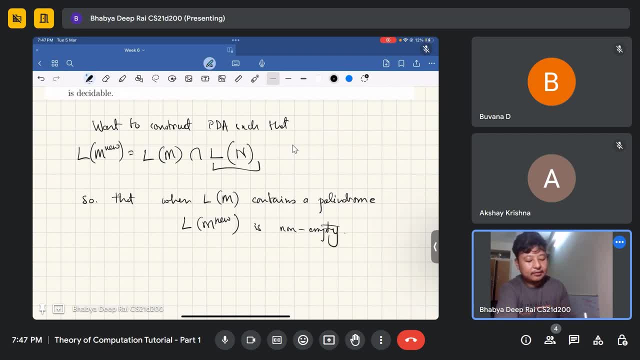 this language of m- new, that is the intersection, is non non. this language of m new, that is the intersection, is non empty. and and and l of m, l of m, l of m does not, does not, does not contain, contain, contain palindrome, then l of, then l of. 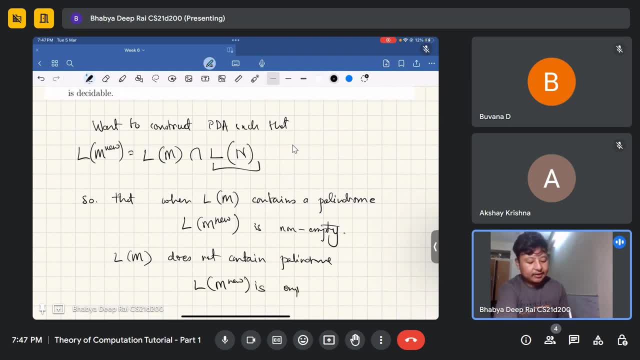 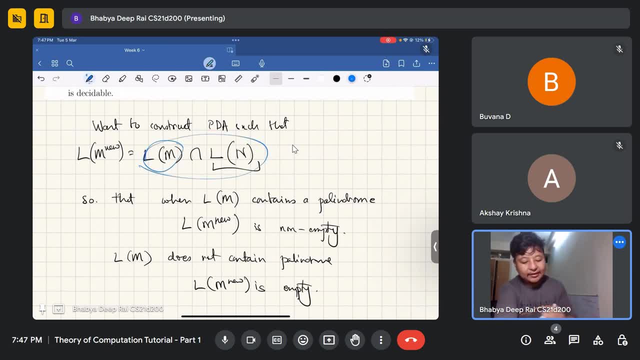 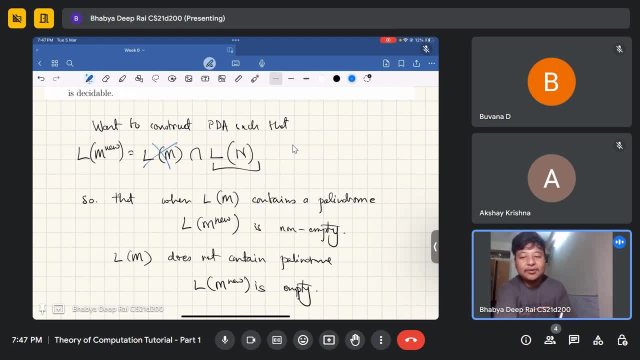 the set resulting set should be non-empty. the set resulting set should be non-empty. and if it, and if it, and if it does not contain a palindrome- no, does not contain a palindrome, no, does not contain a palindrome, no, palindrome here, palindrome here. palindrome here, then the interest, their intersection. 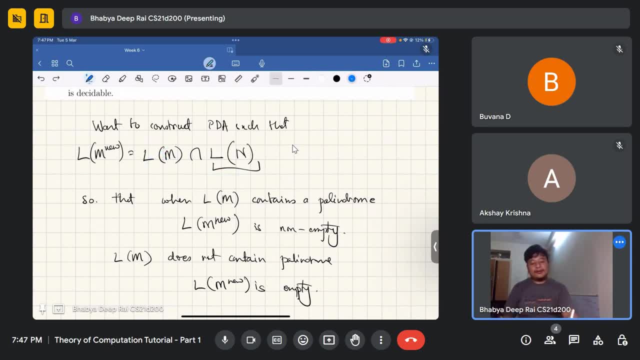 then the interest, their intersection, then the interest, their intersection should be empty. so any idea should be empty. so any idea should be empty. so any idea: what, what, what l of n should be, l of n should be, l of n should be what should l and b? 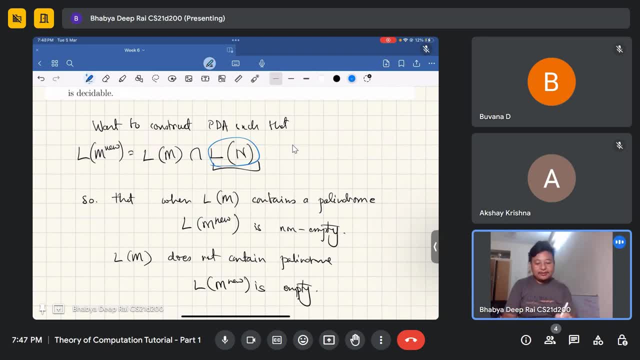 what should l and b. what should l and b? okay, l of n b, so that, okay, l of n b. so that, okay, l of n b, so that, when this accepts a palindrome guy, when this accepts a palindrome guy, when this accepts a palindrome guy, okay, okay. 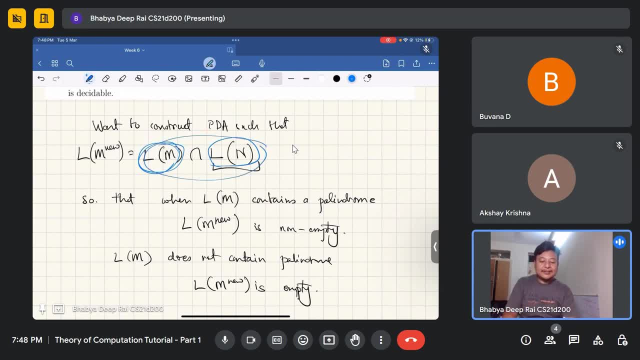 okay, this guy accepts a palindrome, then this guy accepts a palindrome. then this guy accepts a palindrome, then their intersection: these two, the their intersection, these two, the their intersection, these two, the intersection is, intersection is. intersection is. non-empty, it will contain something. non-empty, it will contain something. 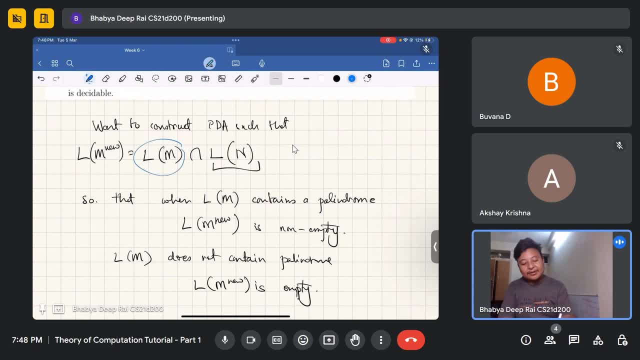 non-empty. it will contain something and and, and. if l of m does not contain a palindrome, if l of m does not contain a palindrome, if l of m does not contain a palindrome, then on intersecting with l of n, then on intersecting with l of n. 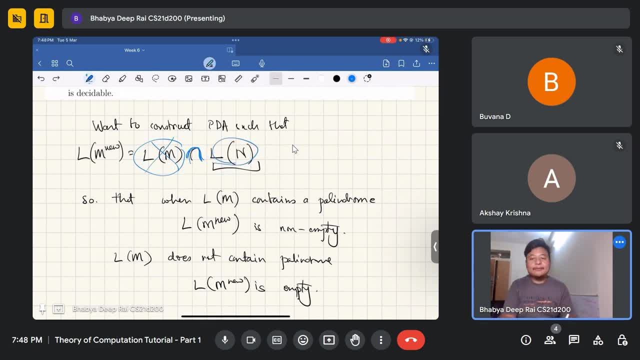 then, on intersecting with l of n, my, my, my set is set is set is empty, empty, empty. think about it, think about it, think about it. compare with what we did previously. it's quite logical also. it's quite logical also. it's quite logical also, any idea. 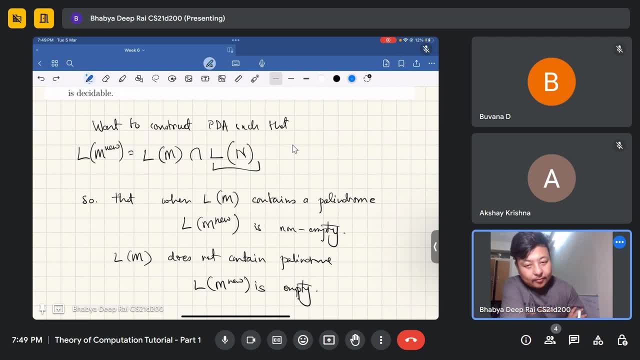 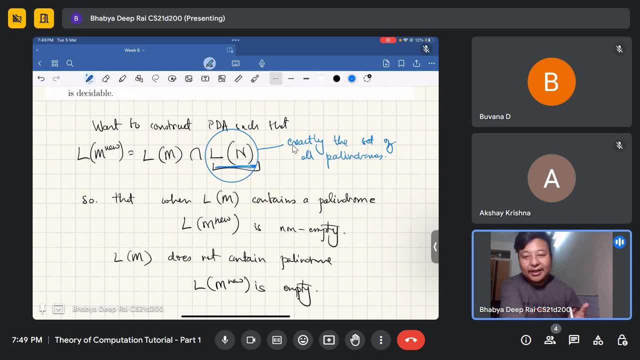 the set of all palindromes, if it contains all palindromes, if elephant, if it contains all palindromes, if elephant, if it contains all palindromes, if elephant contains all palindromes, contains all palindromes, then if l of n contains even one palindrome, 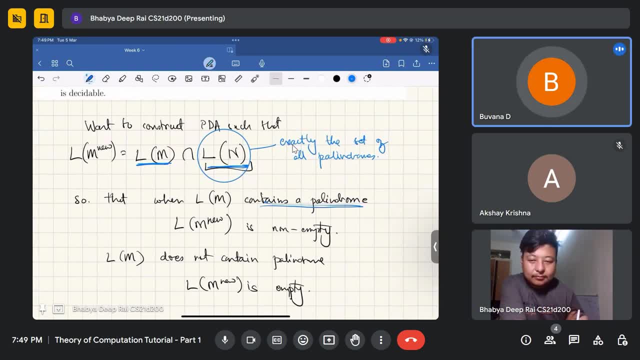 then if l of n contains even one palindrome, then if l of n contains even one palindrome, sir, sir, sir, yeah, this i have understood sir, this, you, yeah, this i have understood sir, this, you, yeah, this, i have understood sir, this you understood, right, understood, right understood, right getting it. so, if you take it good, so if 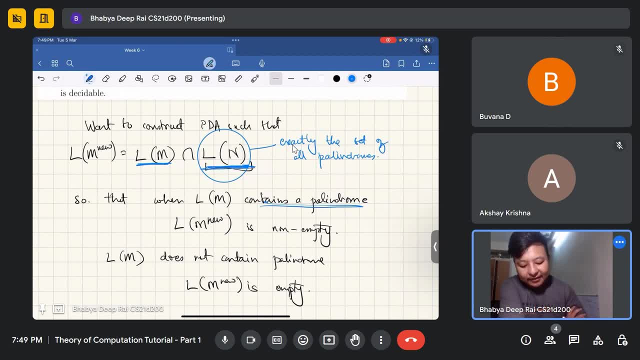 getting it, so, if you take it good. so if getting it, so, if you take it good, so if you take this to be the set of all, you take this to be the set of all, you take this to be the set of all palindromes, even if this guy has at. 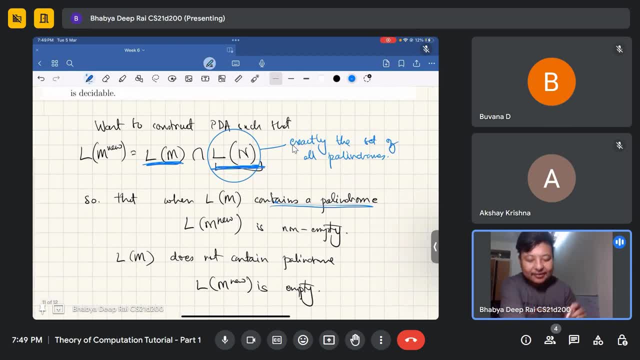 palindromes, even if this guy has at palindromes, even if this guy has at least one palindrome, their intersection, least one palindrome, their intersection, least one palindrome, their intersection. there is one common member, there is one. there is one common member, there is one. 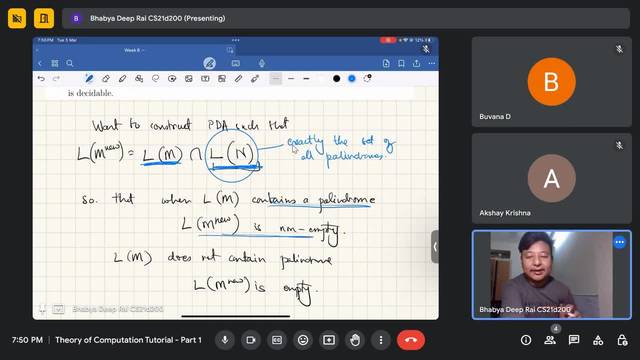 there is one common member, there is one common element, and therefore m new is common element, and therefore m new is common element, and therefore m new is non-empty. it contains at least that non-empty. it contains at least that non-empty. it contains at least that particular string, which is a palindrome. 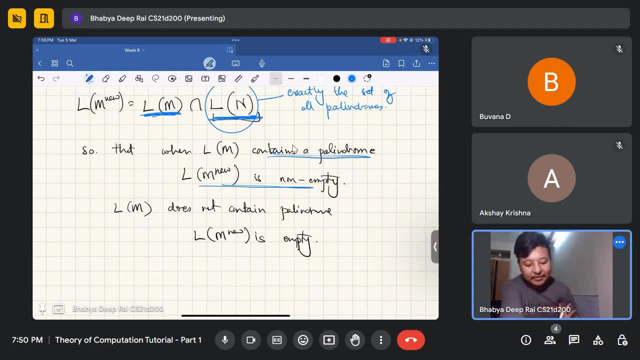 particular string which is a palindrome, particular string which is a palindrome, which l of m, which m accepts okay, which which l of m, which m accepts okay, which which l of m, which m accepts okay, which is contained in elephant. now if elephant does not contain any. now if elephant does not contain any, 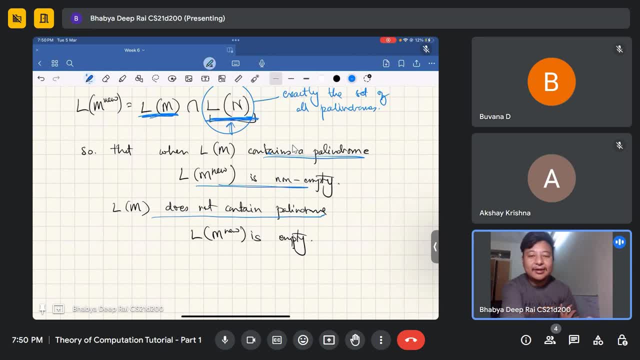 now, if elephant does not contain any palindromes, palindromes, palindromes, obviously it has nothing in common with. obviously it has nothing in common with. obviously it has nothing in common with this set right, because this guy is only this set right, because this guy is only 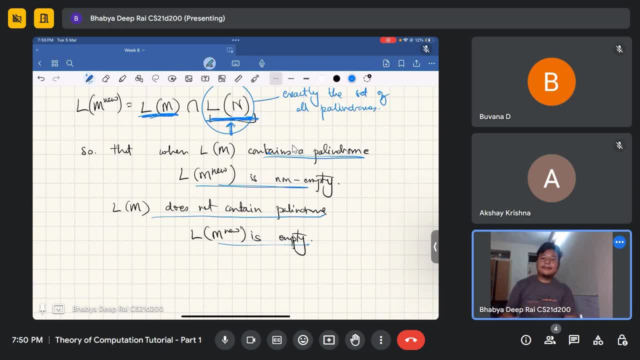 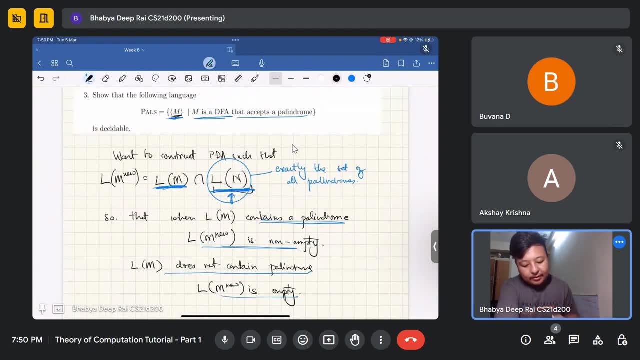 this set right, because this guy is only consisting of palindromes. so obviously consisting of palindromes. so obviously consisting of palindromes. so obviously, lfm new is empty. lfm new is empty. lfm new is empty. okay, okay, okay, so. 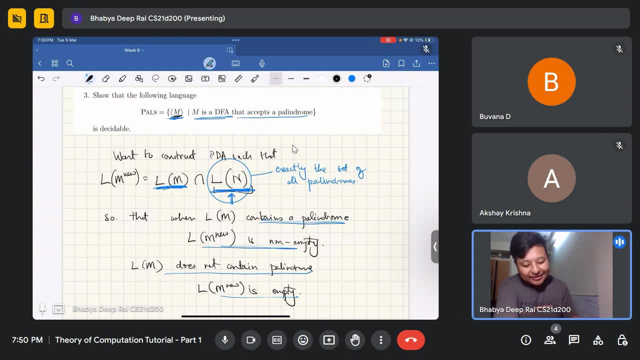 uh, uh, uh, right, right, right now. the question is: uh, why is this a? now? the question is: uh, why is this a? now? the question is: uh, why is this a pda? why is n a pda? well, because. now the question is: uh, why is n a pda? well, because. 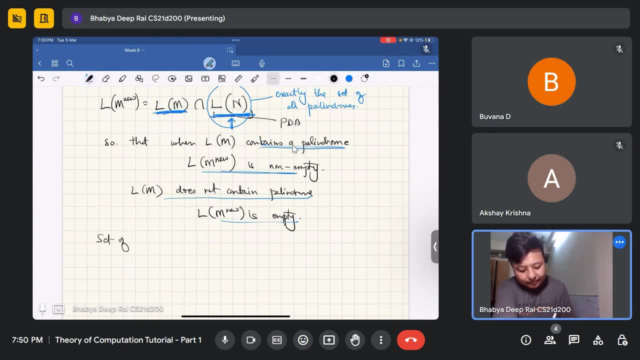 now the question is: uh, why is n a pda? well, because the set of all palindromes is a context-free language. why, well, you is a context-free language? why, well, you is a context-free language? why, well, you can generate a grammar for it, you know. 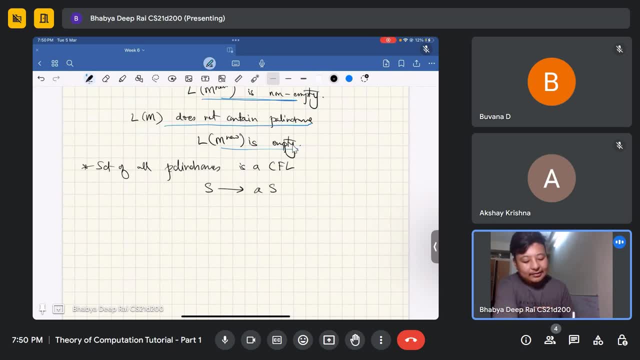 can generate a grammar for it. you know can generate a grammar for it. you know you can do, you can do, you can do. this is the grammar for it, is the grammar for it, is the grammar for it: s, s, s, b, b, b or, if you take binary: 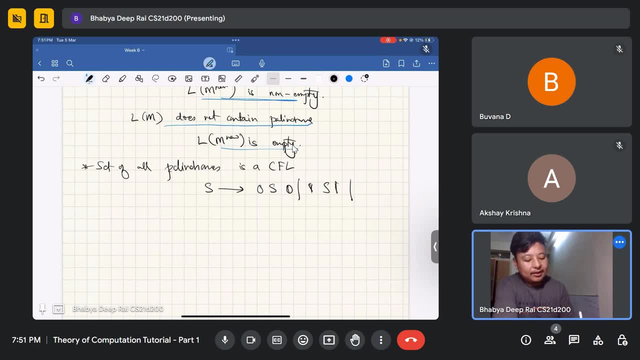 or if you take binary, or if you take binary, 0s, 0s, 0s, 0s, 0, 1 s, 1, 0s, 1, 0s, 1, um, um, um, zero, zero, zero, one, one, one, or epsilon, or epsilon. 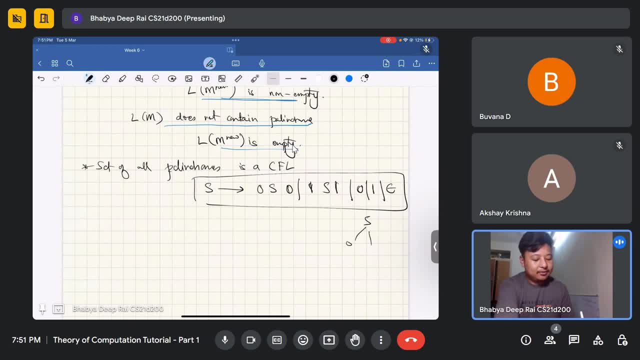 or epsilon. so this is the grammar that generates. so this is the grammar that generates. so this is the grammar that generates palindromes like zero, palindromes like zero, palindromes like zero s, zero s, zero s zero, one s one, one s one. 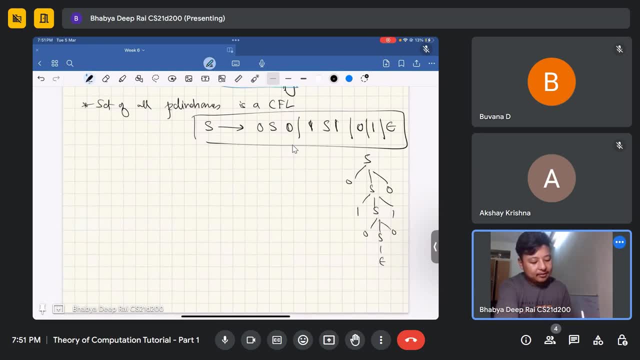 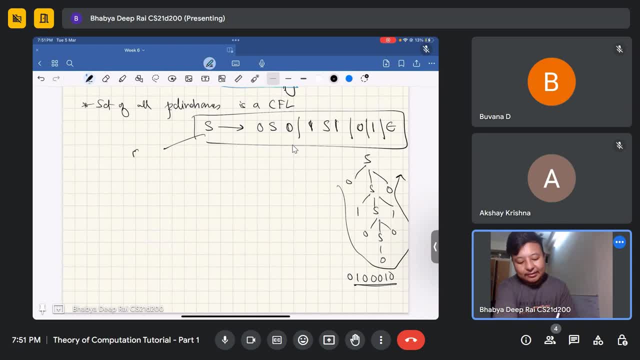 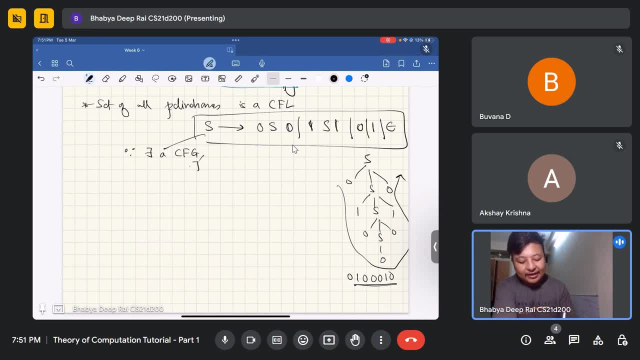 since there is a cfl cfg, since there is a cfl cfg, that means a cfl. that means also a cfl. that means a cfl. that means also a cfl. that means a cfl. that means also a cfl. there exists a pdf. 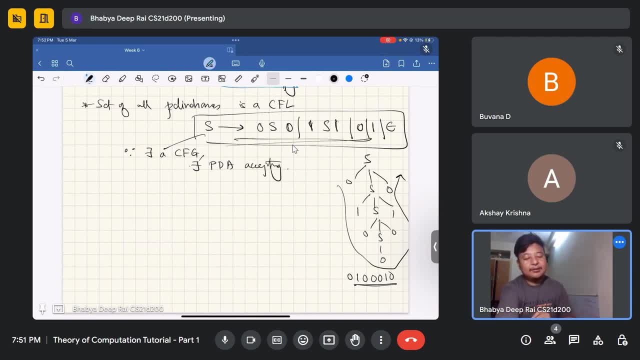 there exists a pdf, there exists a pdf accepting, accepting, accepting this, this, this grammar, grammar, grammar, which is nothing but a set of all, which is nothing but a set of all, which is nothing but a set of all. palindromes, so a pda exists. palindromes, so a pda exists.